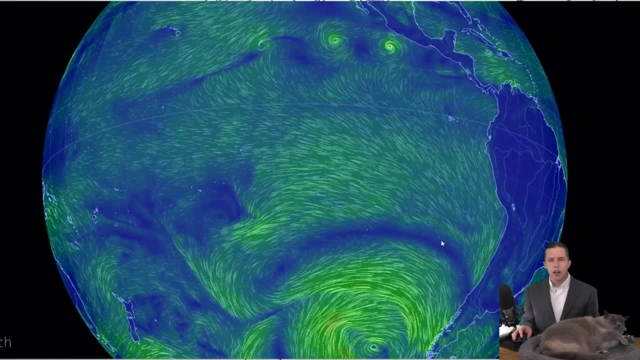 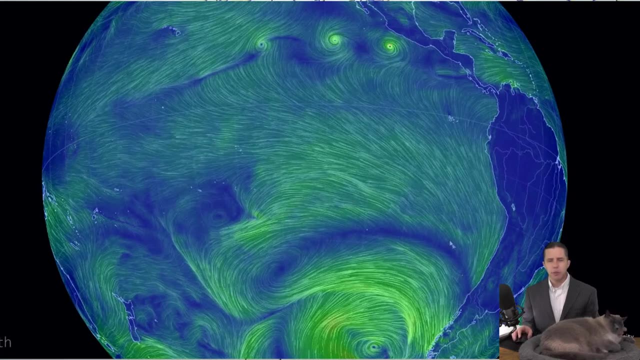 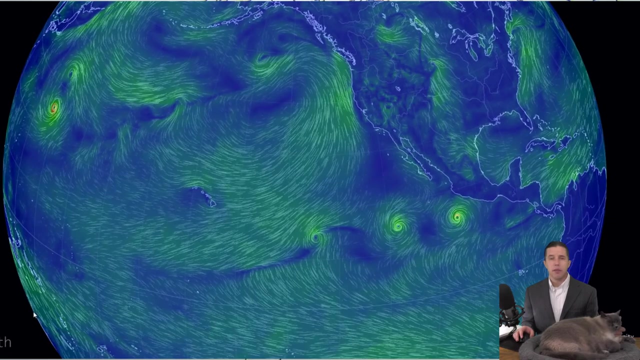 And if we look down here, we can also see this funny-looking thing. here is also another subtropical high. It's not very symmetrical, It's a weird shape today. Okay, so what I'm going to do is I'm going to look at sea surface temperature. So to do that, I click the word. earth Mode is ocean. 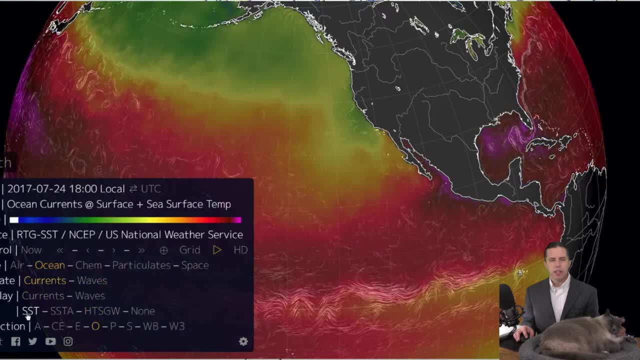 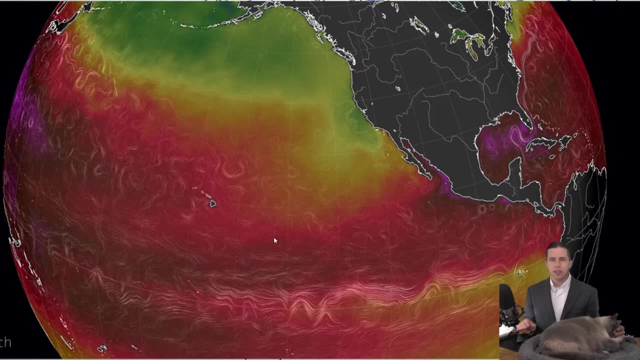 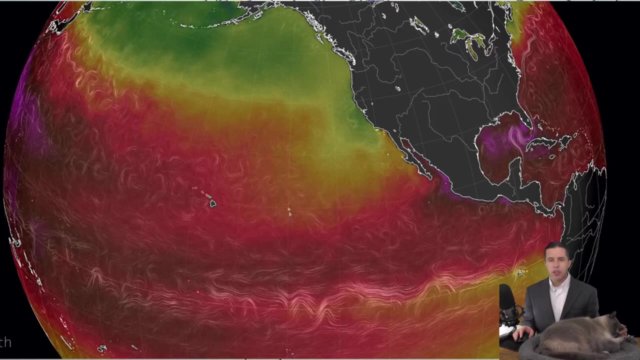 Animate currents Overlay. SST for sea surface temperature. Okay, so the colors now represent what we call the skin temperature of the ocean. So this is the temperature of the ocean water right at the surface, And we can actually measure this. We've got satellites up that measure this every day. 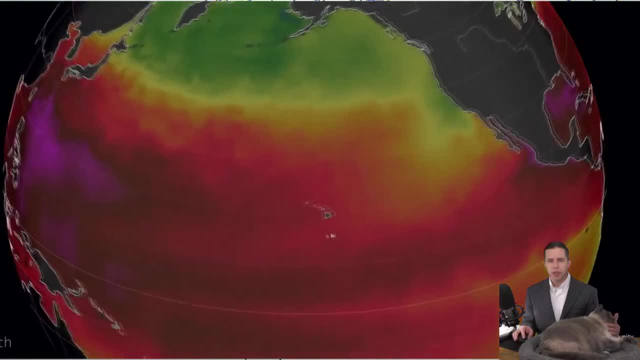 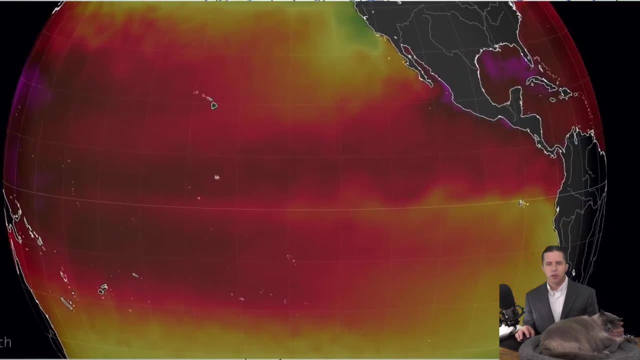 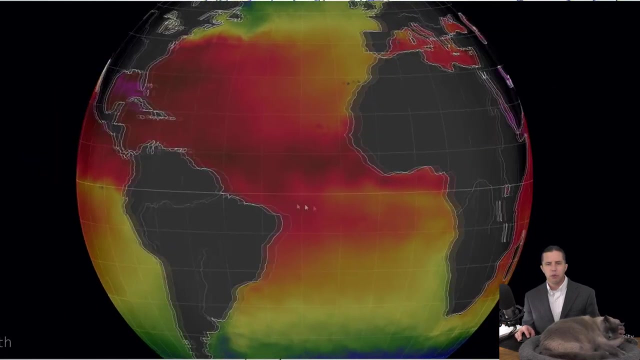 And so the colors represent temperatures you might expect. And so a couple things we can see. For one thing we can see there's a band of pretty warm temperatures, not exactly at the equator but kind of around the equator. So if I just kind of zoom out right, so we've got a band of pretty warm temperatures near the equatorial region, but it's not very symmetrical. 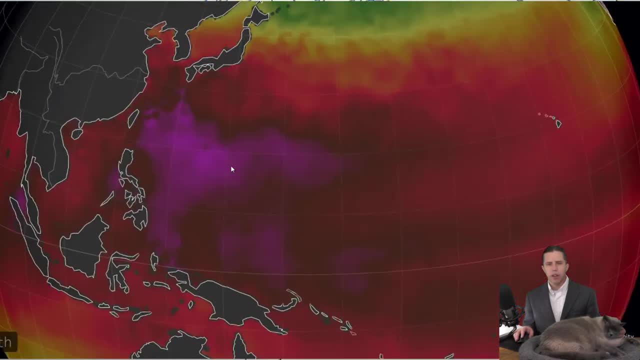 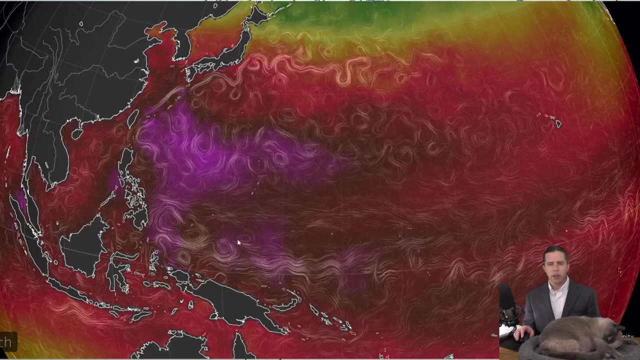 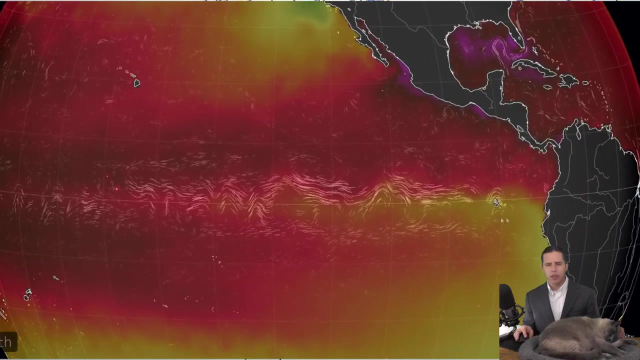 For example, over here this purple that's even warmer than the red. So you've got this pool of really warm water kind of over here in the western part of the Pacific Basin. And then there's this weird thing where, right at the equator, it's actually kind of cooler than the water around it, which is maybe not what you would expect. 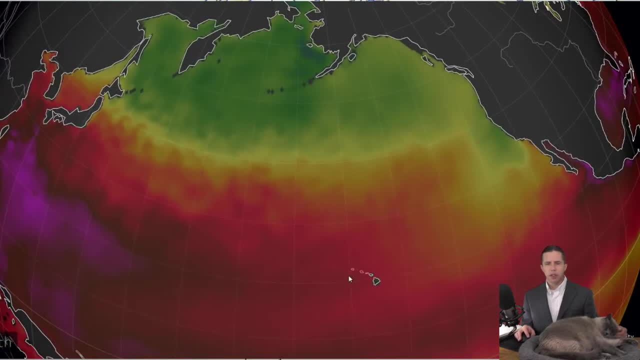 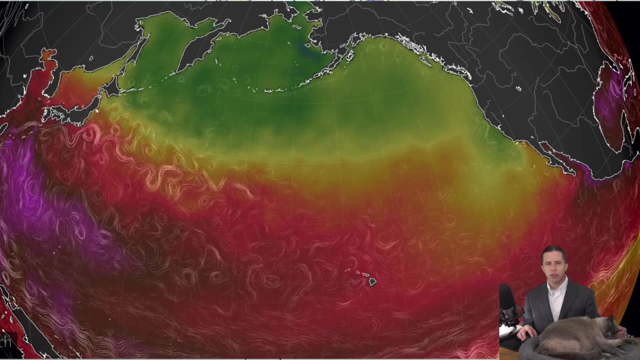 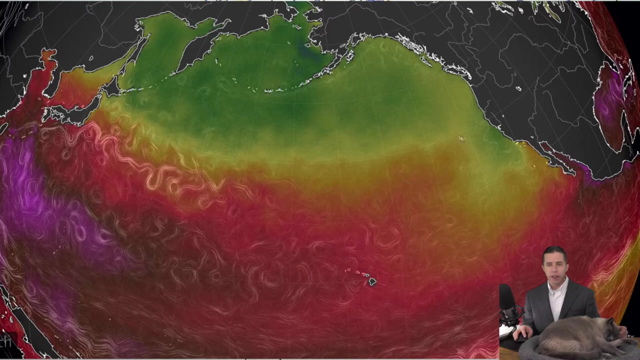 Now, if I look around here, let's look at the Pacific Basin- Notice that if I were to pick, say, a certain line of latitude and go straight across, stick at this line of latitude right here, that over on the eastern side of the Pacific Ocean it's colder than it is on the western side. 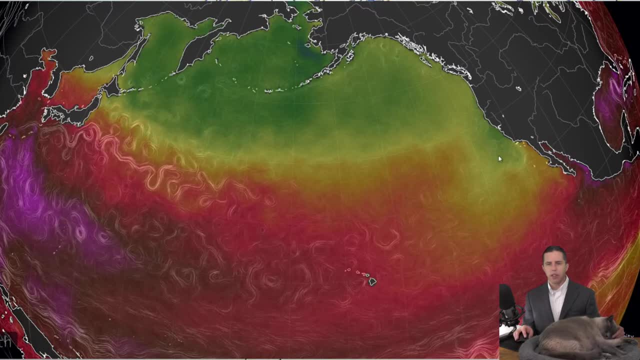 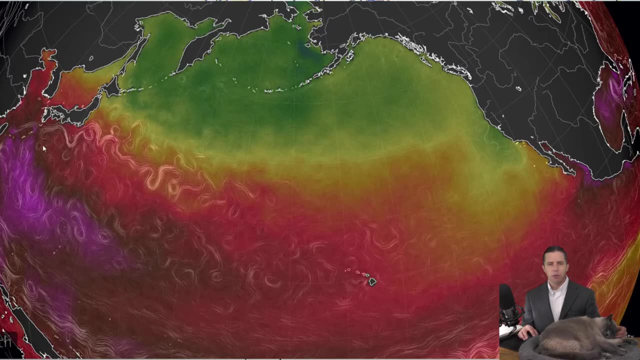 Right, so you can see this greenish, yellow color coming down here, whereas if I just pick one line of latitude like that spot right there and I go all the way across, it's much, much warmer on the western side, where, as if I just pick one line of latitude like that spot right there and I go all the way across, it's much, much warmer on the western side. 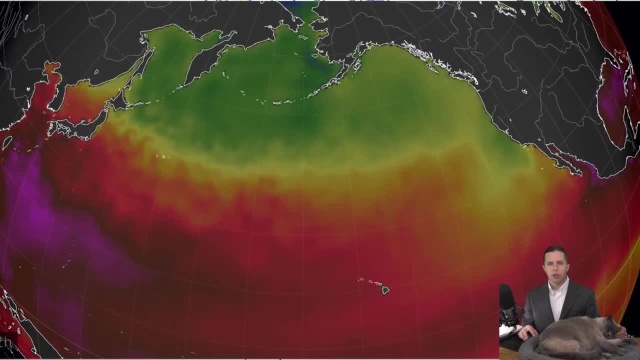 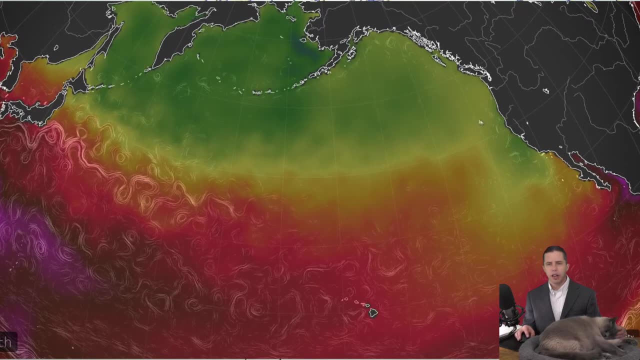 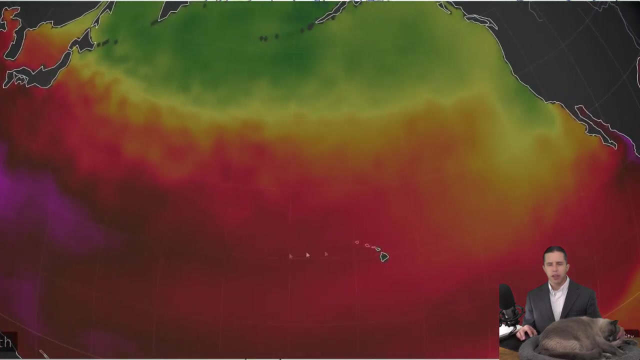 than the eastern side. so something is causing the ocean to be asymmetric in terms of temperature, that there's something that's dragging colder water down from the north and allowing this warmer water to kind of come up from the south. okay, and if i look at the southern basin, 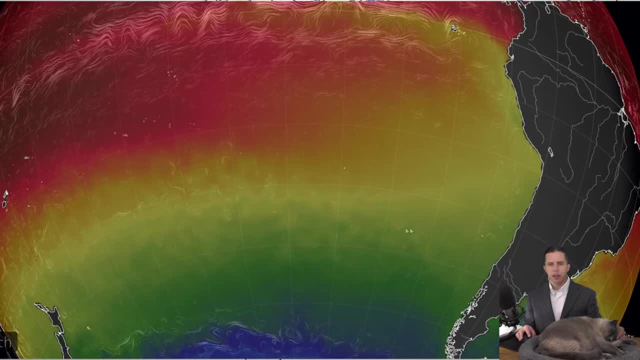 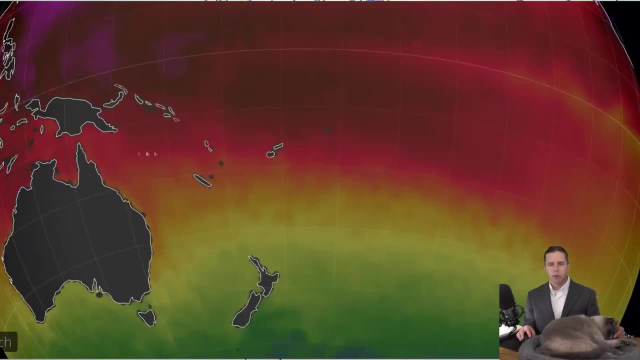 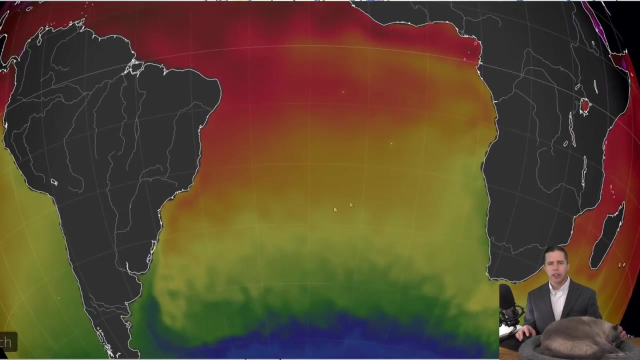 i see kind of the same thing. i see cooler water that is being pulled up here to the north and i see warmer water over here to the west. it's not symmetrical. and if i move over to the atlantic i see something kind of similar. i've got cooler water up here, warmer water down there. 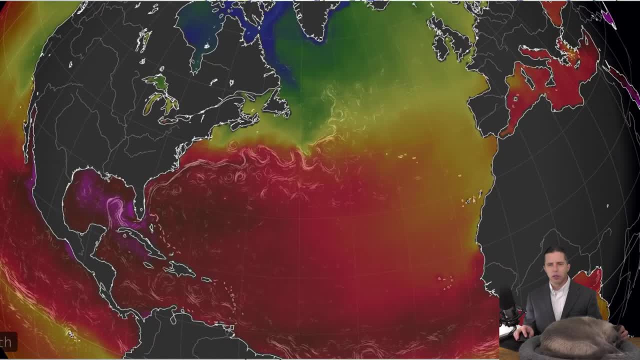 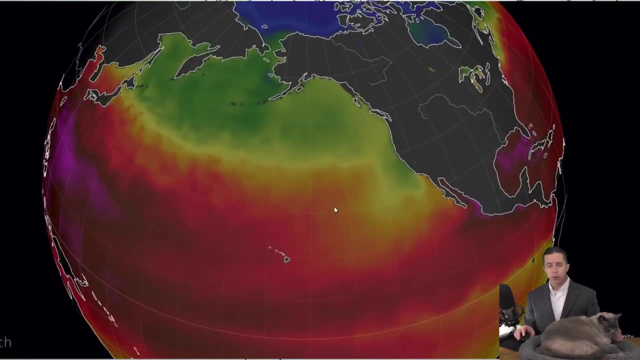 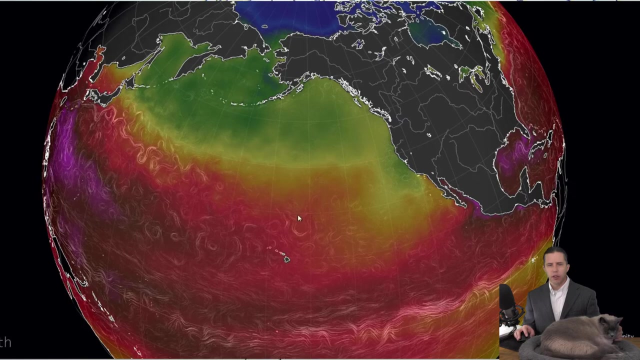 and up here somewhere again. cooler water down there, warmer water up here, so the the ocean basins are not symmetrical in their temperature. so the first question is: why is that okay? why would it be colder over here and warmer over here? so the answer is that just a minute ago we saw 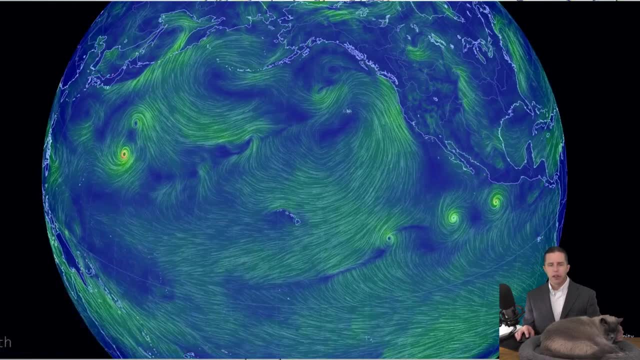 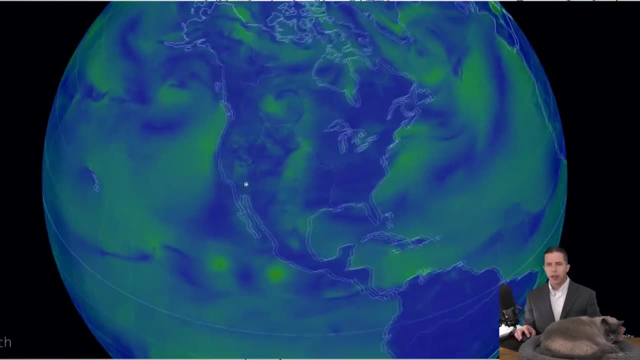 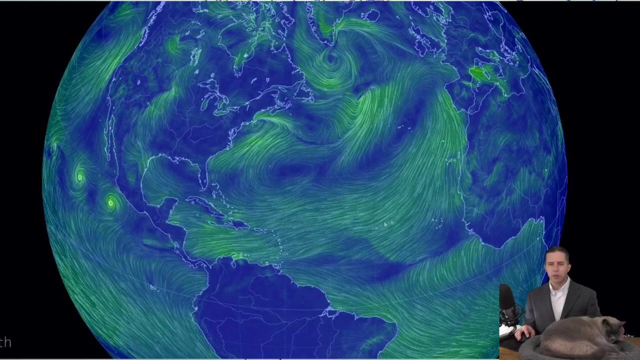 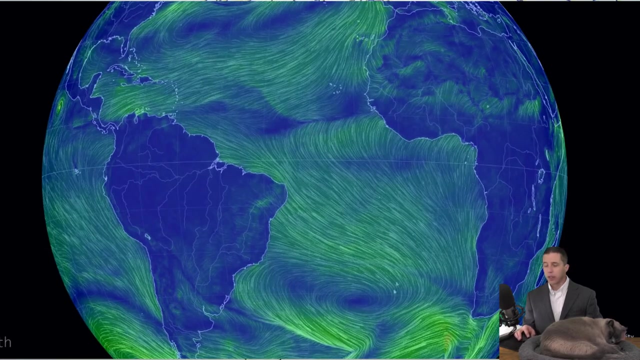 that there are big clockwise winds out here in the pacific, the pacific subtropical high, and then over here in the atlantic another one, big again- it's not perfectly shaped on on this particular day- and of course they go uh counterclockwise in the pacific or, i'm sorry, in the in the southern hemisphere. so you've got. 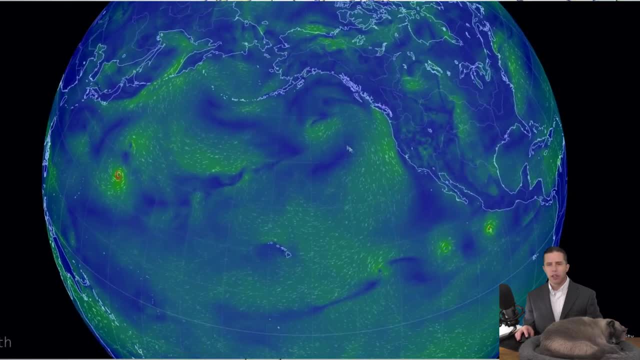 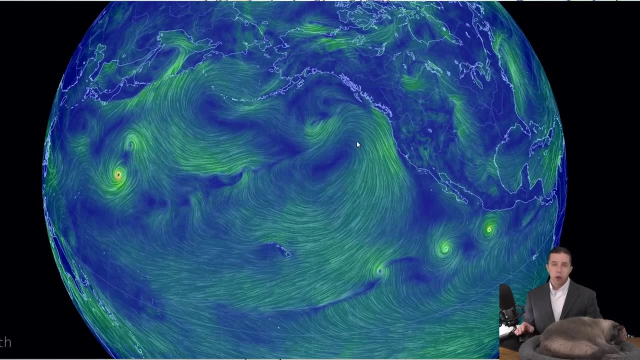 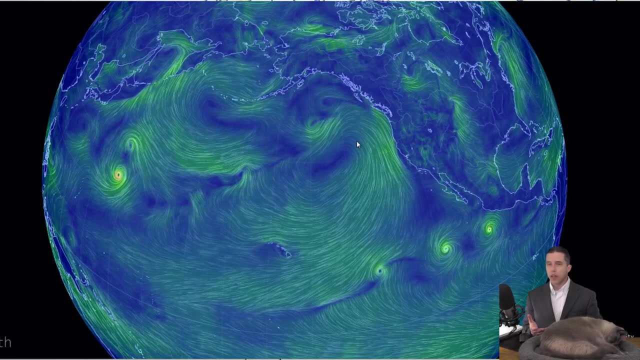 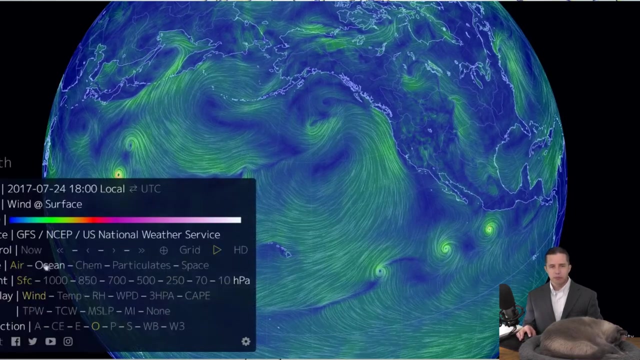 these subtropical highs that are just spinning around and around and around all day long, every day out in the ocean, and the wind blows the ocean. so the reason we have ocean currents, for the most part, is wind. the reason we have waves is wind. wind is what's pushing the ocean around, and so when we look at this temperature, so again, 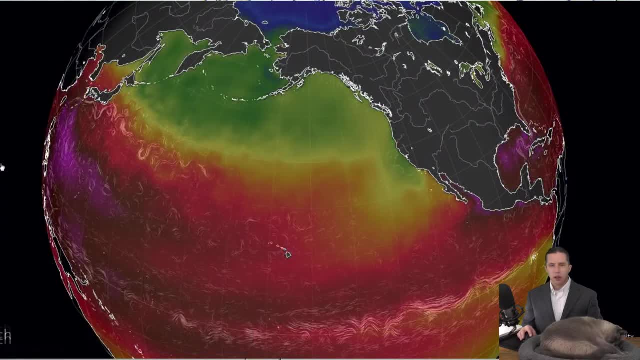 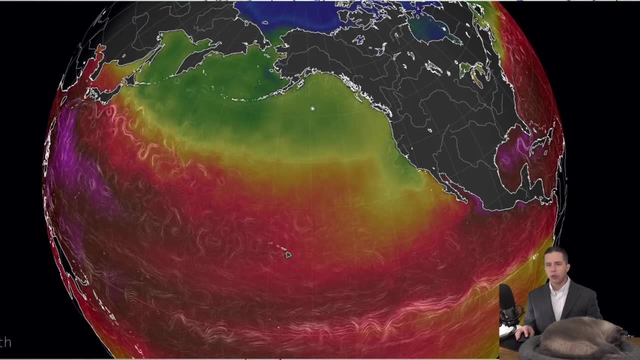 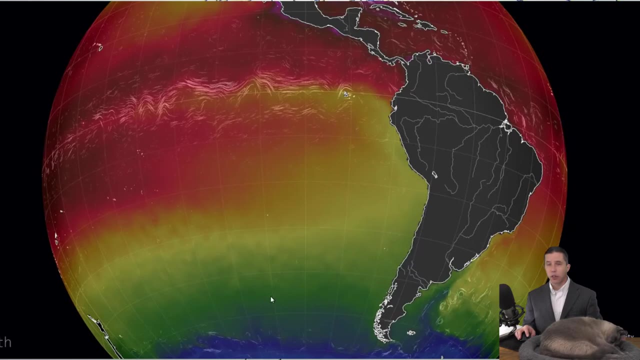 ocean currents sst. that is the result of the pacific subtropical high blowing the ocean towards the south, blowing this colder water down towards the equator and down here. same thing, except instead of going clockwise, it's going counterclockwise. so you've got winds blowing. cold water towards the north. so one of the things that these subtropical highs do is they help bring cold water from up here down towards the equator and they take warm water from the equator and bring it up towards the poles, and they do that in both hemispheres, so they help mix up colder and 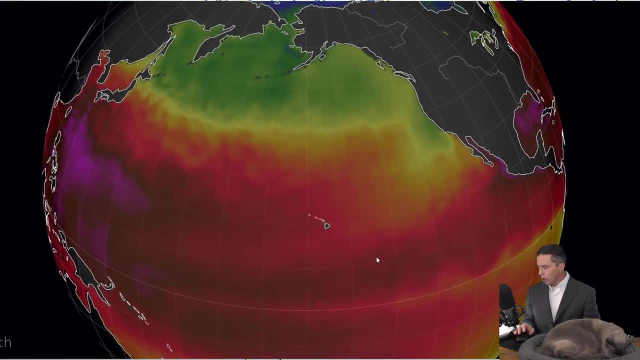 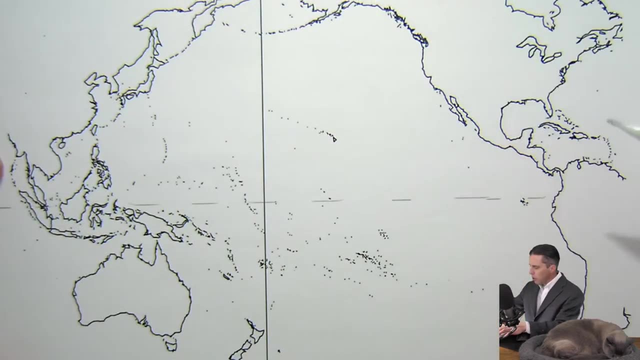 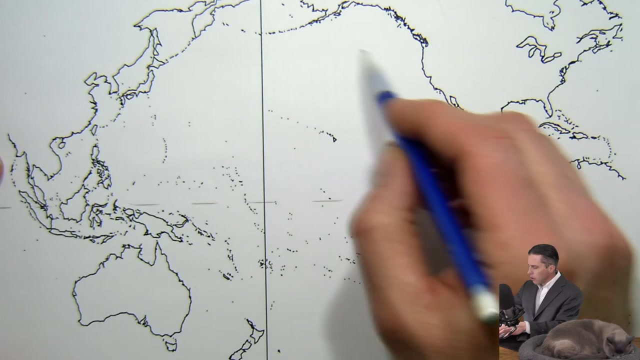 warmer water. okay. so i've got a little map here of the world, and so, in general, what we would notice is that. so so before i start, this is i kind of sketched in the equator. here there's a big loop that's out in the ocean, a big circulation pattern, and it kind of looks like this: 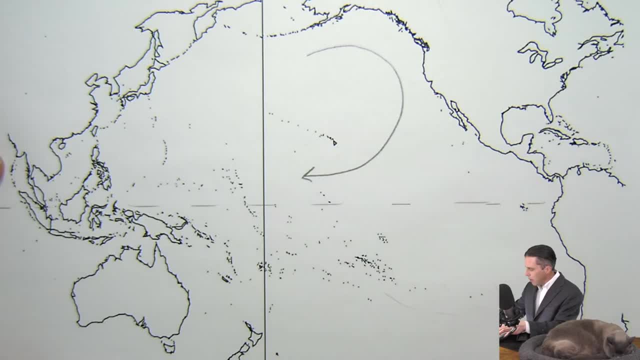 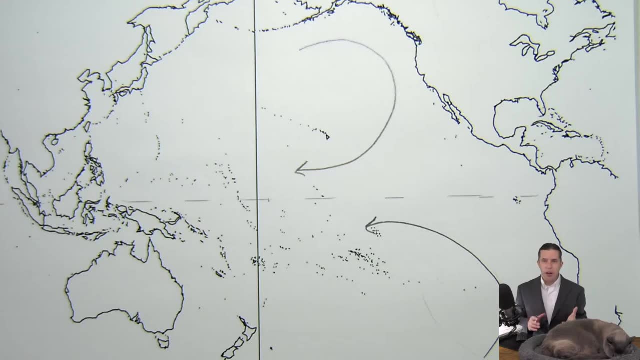 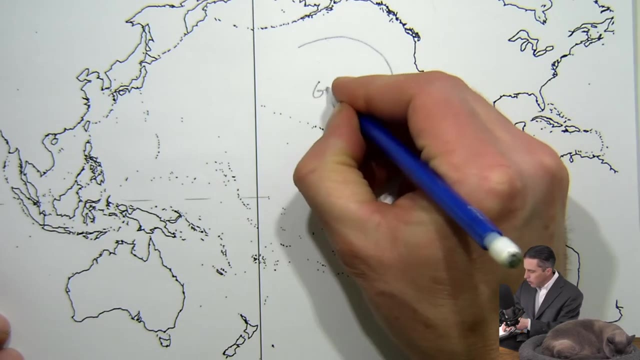 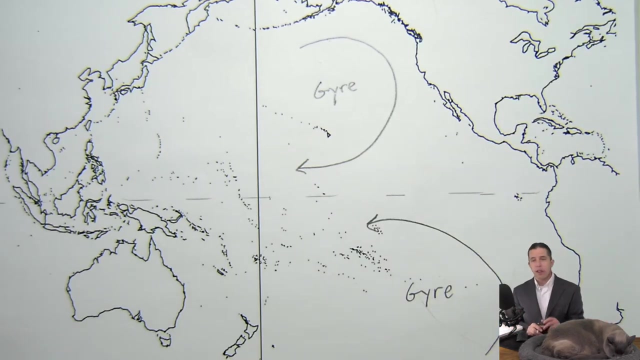 and down here it kind of looks like this: and those loops are being caused by the subtropical highs and in the you know, it's swirming the ocean around in the giant circle and that giant circle is called a gyre. so the the big circulation pattern that we see in the ocean basins is this big. 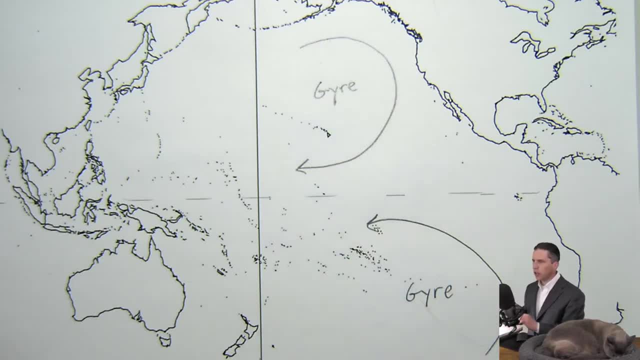 clockwise and then counterclockwise rotation of the ocean caused by the pacific or the subtropical highs, just spinning and spinning, spanning. okay, so that's a primary feature that we see. well, let's add a few more things to this. now. what we know is that near the equator we have the ITCZ right and if you remember back to that, 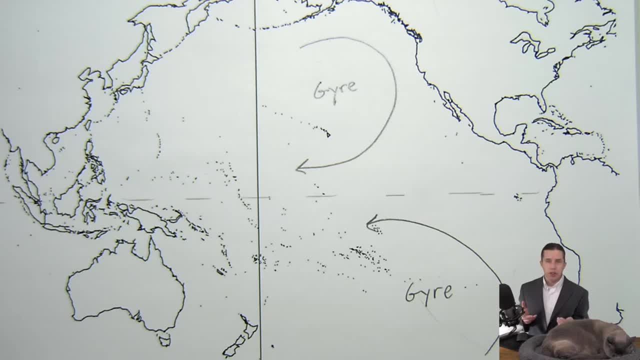 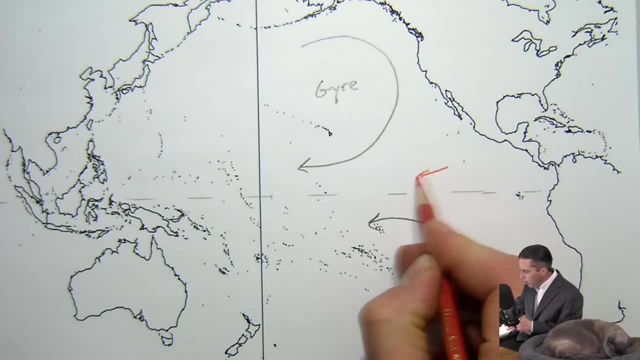 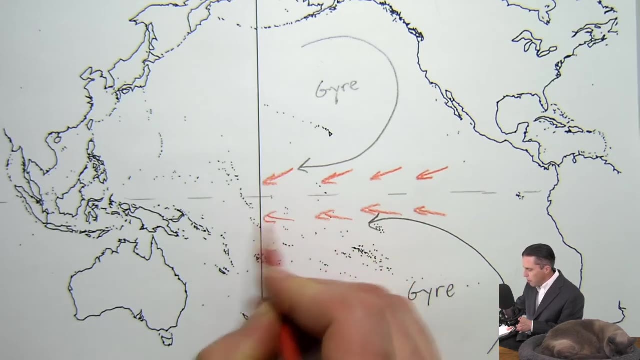 what's happening at the ITCZ. we've got easterlies. what are they doing? they're converging. so I'm going to sketch that in a little bit. so all along here I have easterlies that are coming together now. remember, we said in a past- or yeah, in the past- lecture, that the convergence isn't exactly. 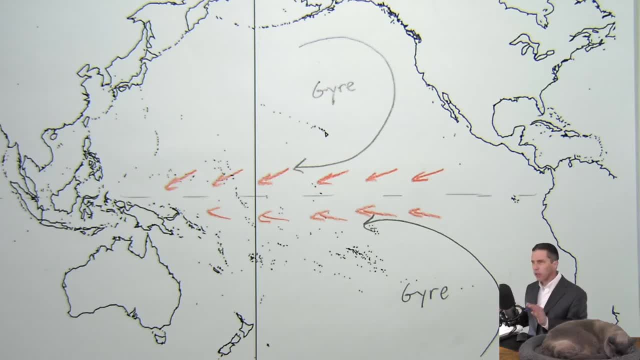 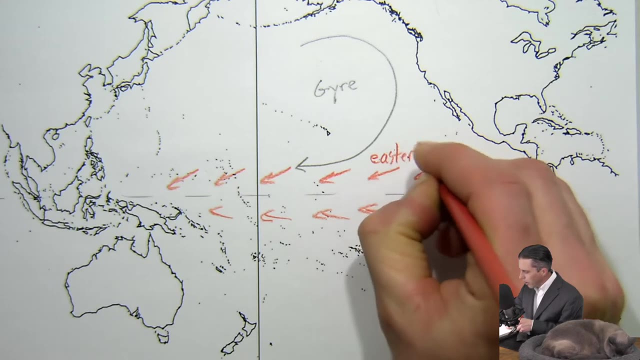 at the equator, that it moves around with the seasons. okay, so I'm drawing this to be along the equator, just to show what to make a point here. but remember, this exact spot changes with the seasons. okay, so there's our easterlies. okay, so let's just think about that for a minute. if you had wind blowing from, 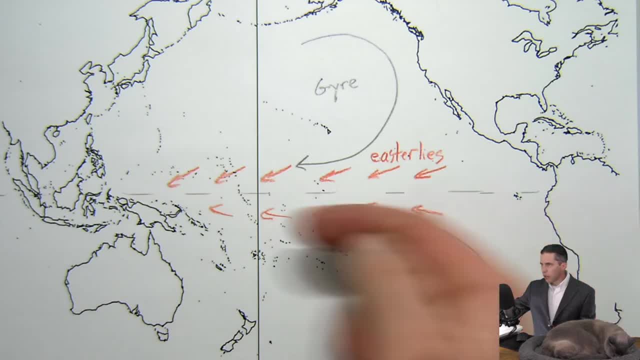 from east to west this direction, and it's blowing along the top of the ocean. what it's going to do is it's going to basically skim the warmest part of the water and push it towards the west. so let's imagine like if you're in a swimming pool and you start doing this. 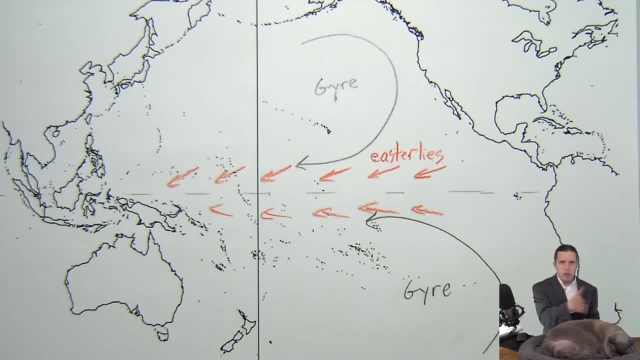 to the top of the water. with your hand, you scoot that water along the surface of the pool. same thing's happening here. so, as a result, we end up taking this warm water because this is near the equator, so it's going to be some of the warmest water in the ocean- at least it should be, and we're. 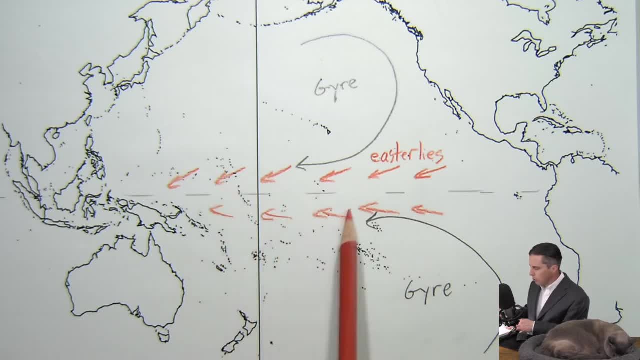 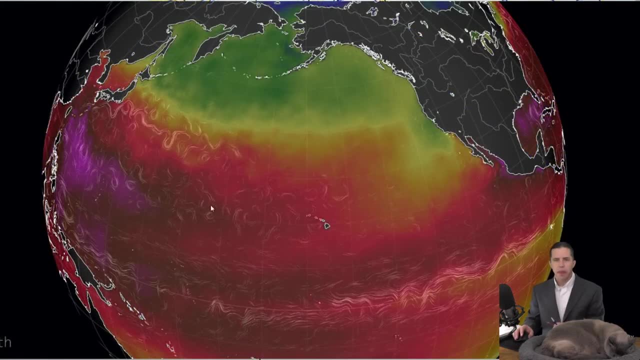 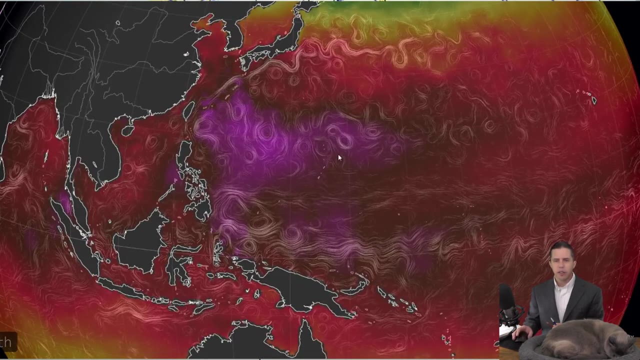 going to shove it this direction and what's going to happen is that really warm water pools up over here. okay, so that's what we're seeing over here. so this purple blob, this is all really warm water. that's kind of been uh shoved over, uh, from the, from the east, it's blown across the ocean. so if 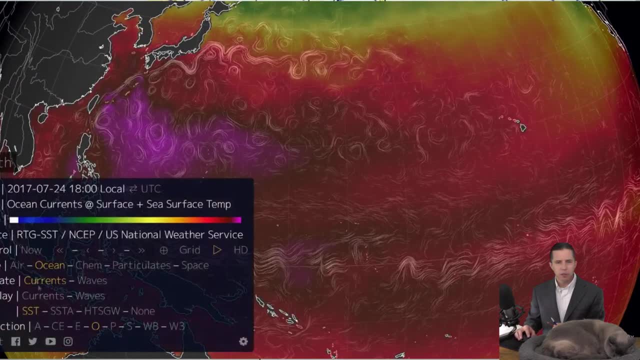 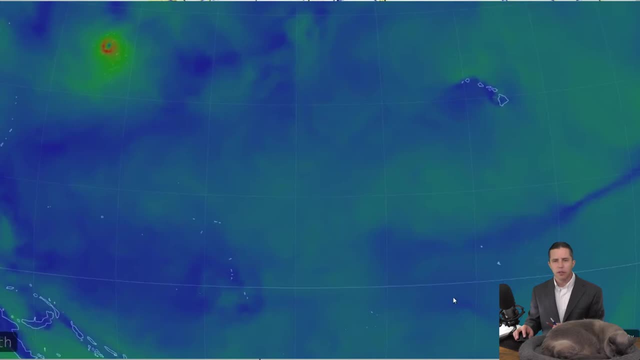 i look at my easterlies, let's look at my. okay. so there's, there's my easterlies, okay, right there. so those are winds, and the winds are just kind of pushing that warm water across the equatorial zone. you see, they're going. today that's a little curvy there, but they're coming this direction. 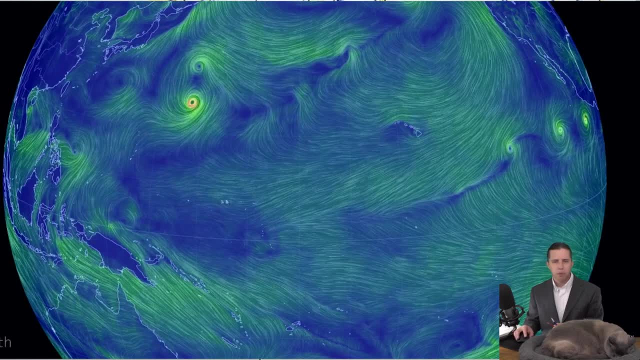 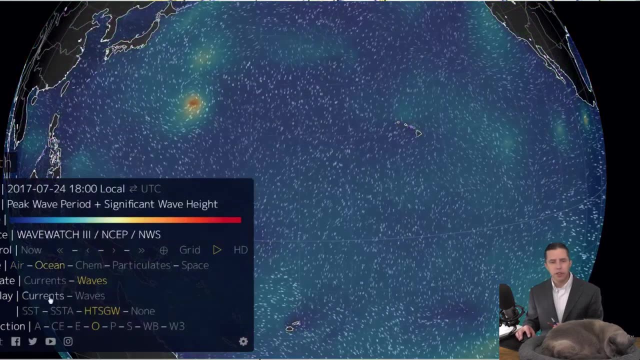 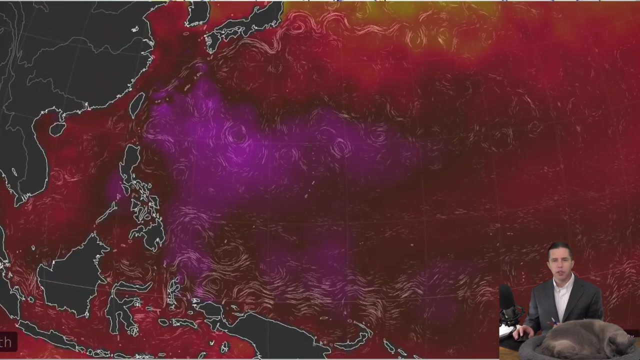 and they kind of die out on this particular day, but they're, they're pooling this really warm water over here by all these island nations. go back to this again, okay. so there it is, that purple water that's the warmest part of the ocean. there's always a pool of just really warm and you feel like bath water if you got into it. 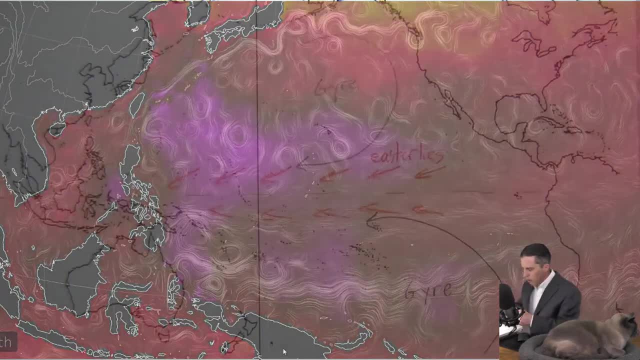 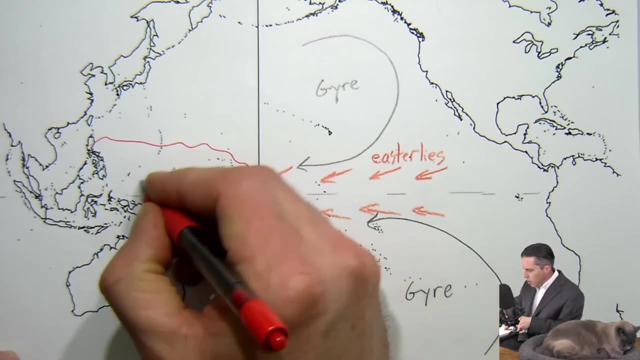 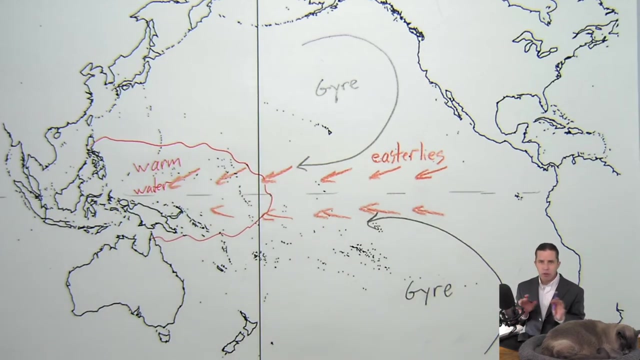 okay, so i'm going to add that to my drawing and i'm just going to kind of approximate that. out in here there's this pool, very warm water, right, and the boundaries are always changing, but it's just kind of over here, okay, so if you're. 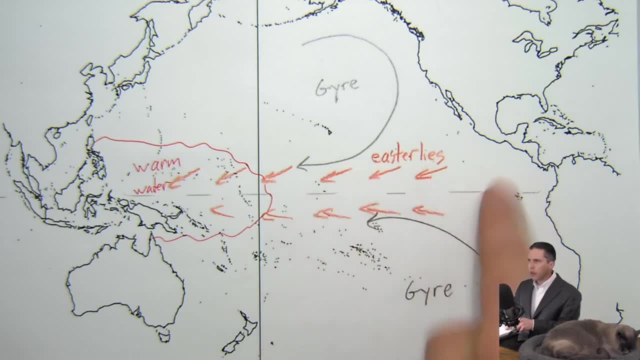 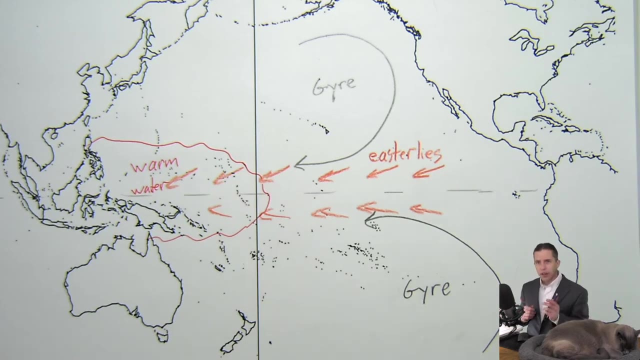 if you're removing water from this part of the ocean, then there has to be some other water that comes up and takes its place. okay, so that's part of the story here, that if i remove the warm water, you're going to have to replace it with something else. now the something else. 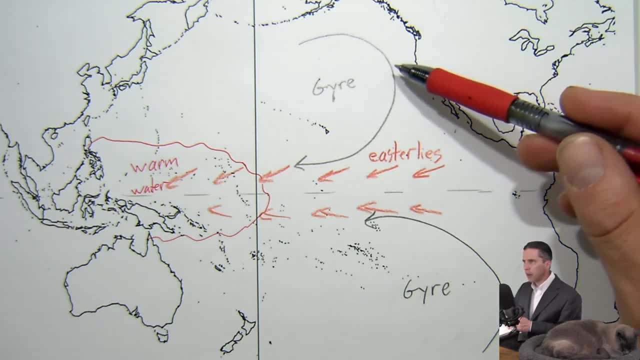 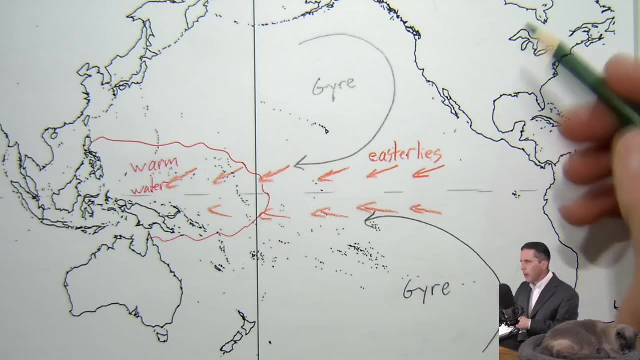 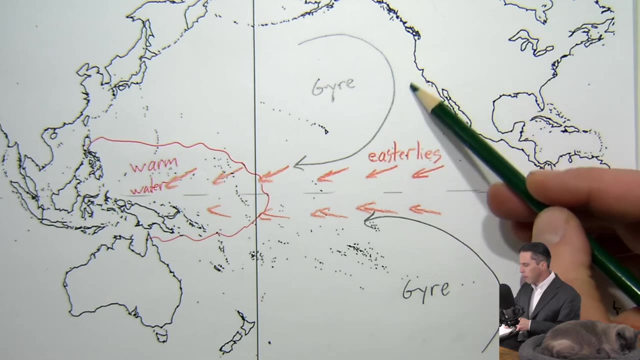 happens to coincide with a place where there's this big bend. okay, so right here, where the, where, the, where the gyre is making a turn by the continent, Imagine it's like you're pulling water away from the continent. So I'm just going to draw some arrows to show that. 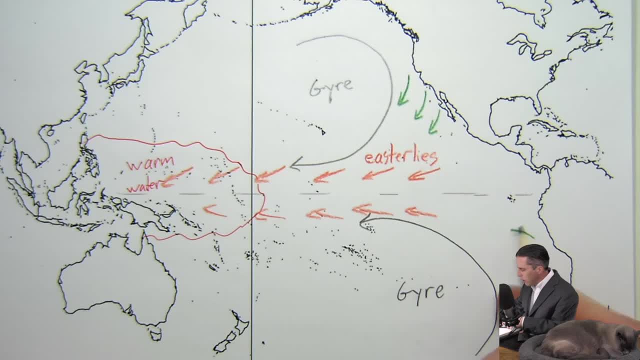 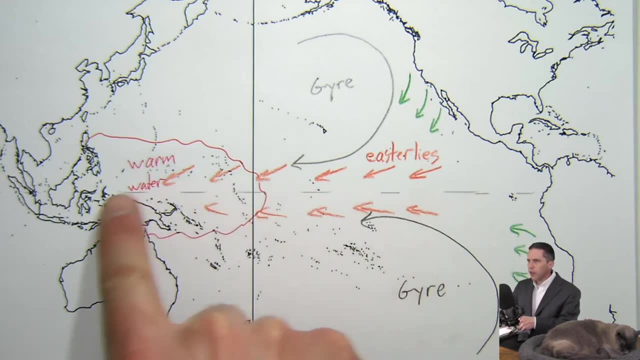 I'm pulling water away from the continent like this. So if I'm moving water across the ocean here and I'm pulling water away from the continent here, we need to produce more water to replace the water that's being pulled away And it turns out the water that comes in to replace it. 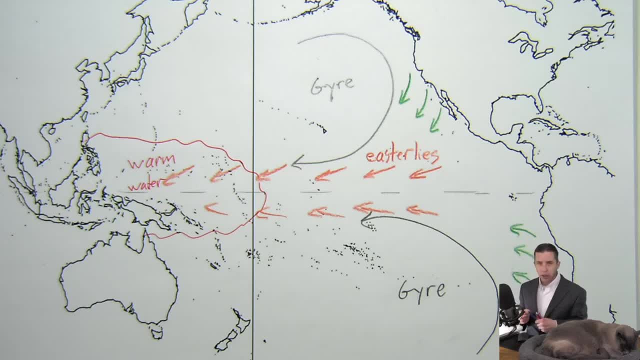 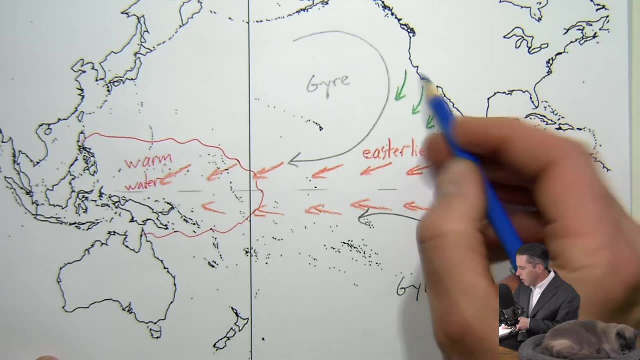 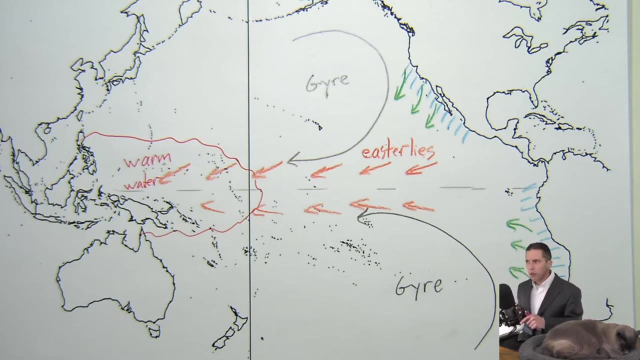 comes up from near the bottom of the ocean. That's called upwelling. So all along here, all along here and all along here, there is water that's coming up from the bottom of the ocean. OK, I'm going to draw that in blue. 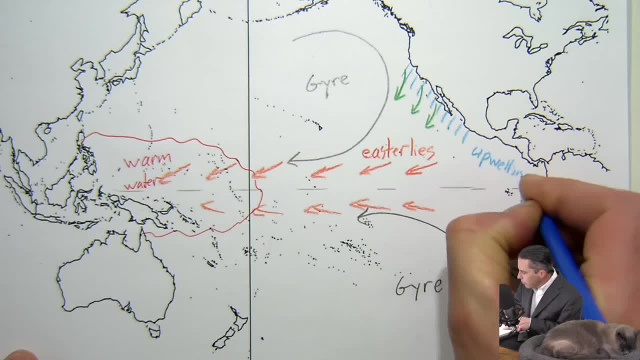 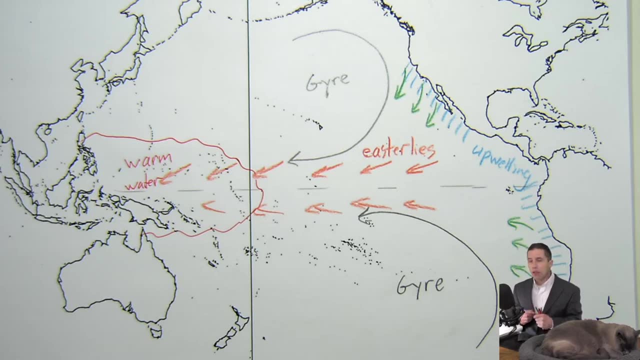 I'm going to call this upwelling. So what's the water? The water at the bottom of the ocean-like. it's very close to the freezing point. Now, because of all the pressure, it doesn't actually freeze down there, but there's places. at the bottom of the ocean that are actually at about 0 degrees Celsius or 32 Fahrenheit, that's at the freezing point. It's just not frozen, So that water comes up to the surface and is really really cold. So this is also a shock to anybody. 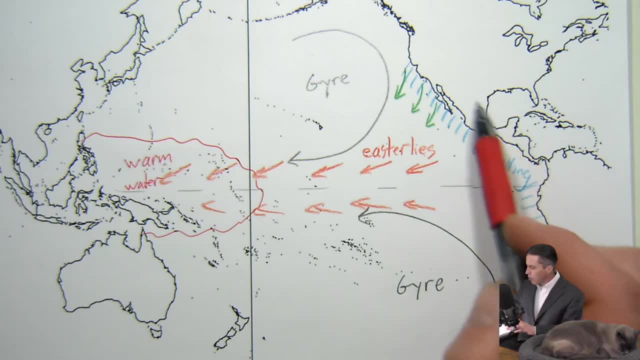 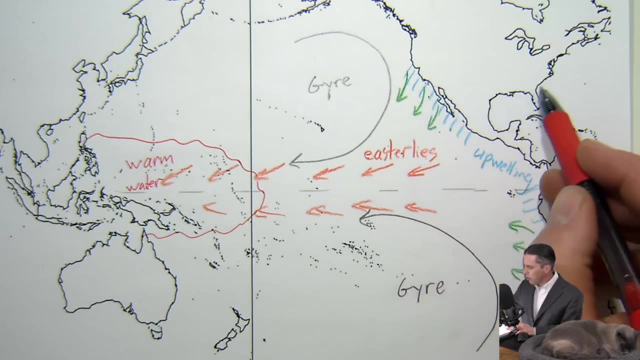 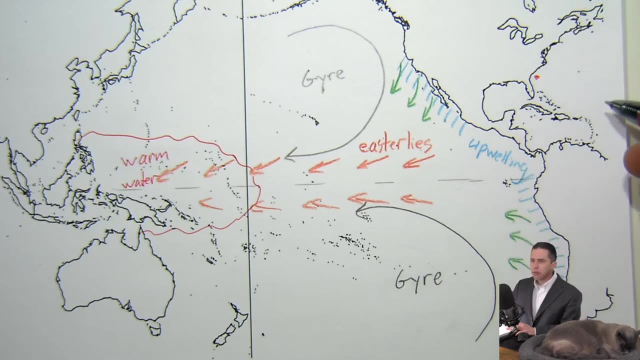 who has tried to go swimming in Southern California. So, for example, LA is somewhere kind of like right in here And if I go across in latitude you're somewhere over here on the East Coast right. If you went swimming out here, it's pretty pleasant. 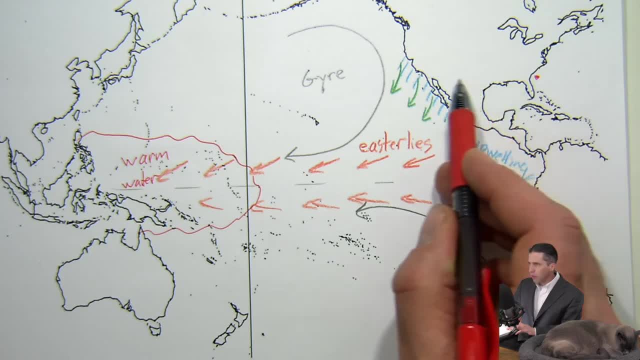 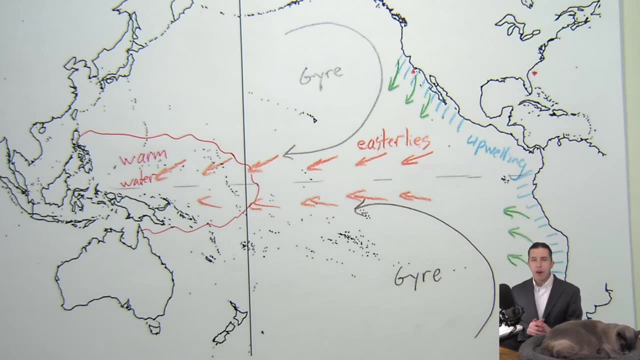 It's nice and warm. If you go hold the same latitude and come over here and go swimming off the coast of, let's say, Los Angeles or San Diego, you find out it's actually really cold And this shocks tourists because they 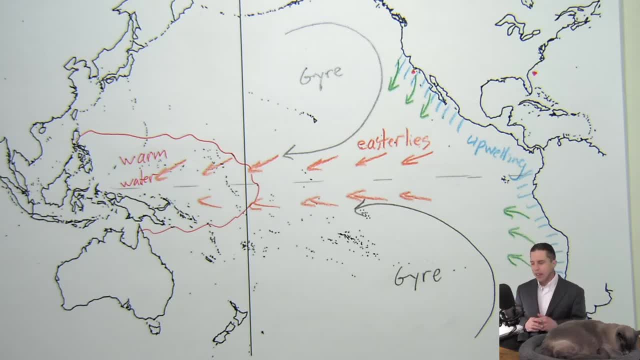 think about Southern California. it's sunny and there's surfers and all this And they get out in the ocean and they're like holy crap, it's cold, Because that water was actually just recently at the bottom of the ocean. 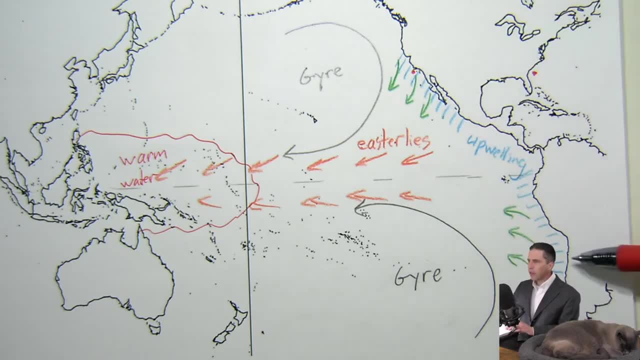 And it's coming up to the surface, as is all along this part of South America. This is all deep cold water coming to the surface. OK, well, it turns out that, besides the water being cold, it has a lot of nutrients in it. 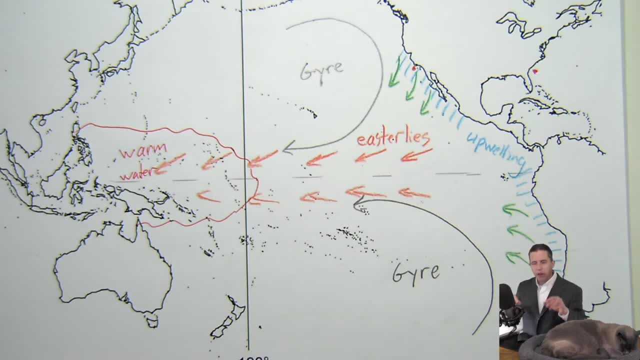 Things die out in the ocean and as little things die and they fall down. that kind of sets up a food chain. When that water comes back up to the surface it's got nutrients in it. Little microorganisms eat that and bigger things. 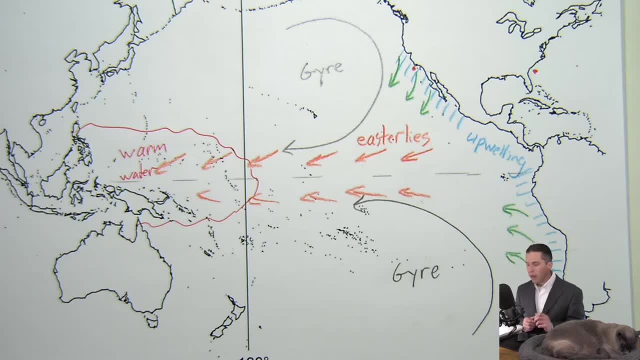 eat the microorganisms, and so on and so forth, until finally you get to fish. And so the fish- actually most of the fish in the ocean live near the continents, in these zones with the cold upwelling water. The fish like the cold water. 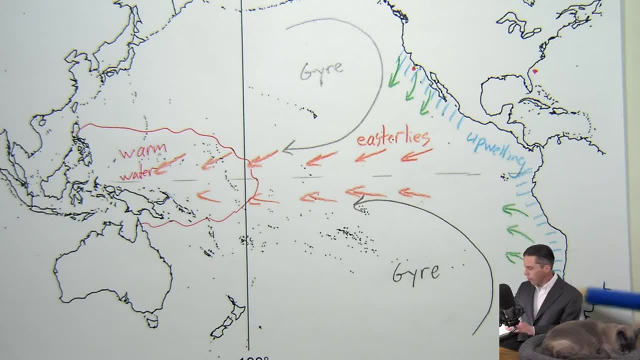 It has all the things that they want to eat in it And so most of the fish they like it. Most of the fish fisheries in the world are kind of up in here, up here and other places where this happens. 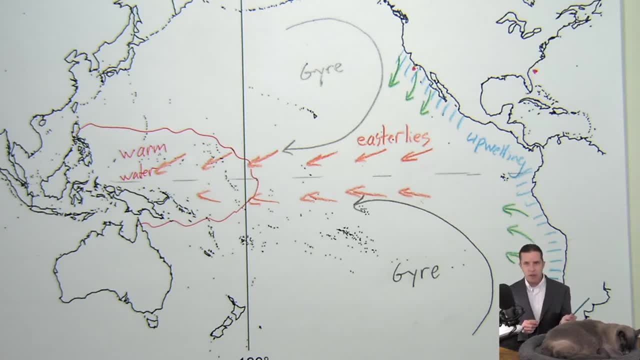 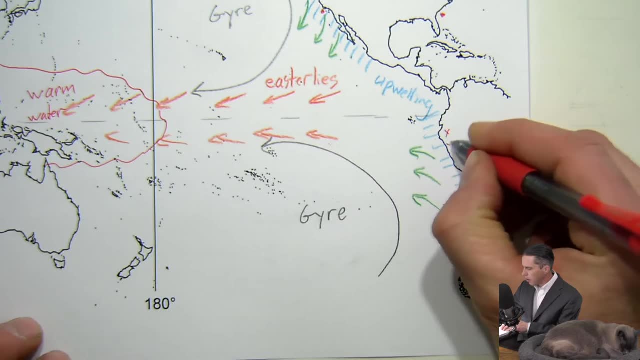 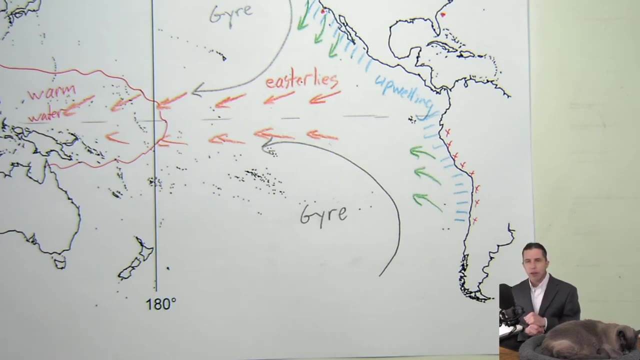 OK, so go back a few thousand years and you've got people that are living all up and down South America. So you have to imagine, in what's now modern day Chile and Peru, people living up and down the coasts. Now, we didn't really talk about this at the time. 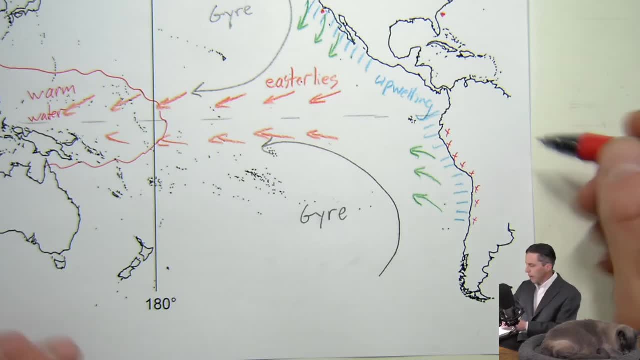 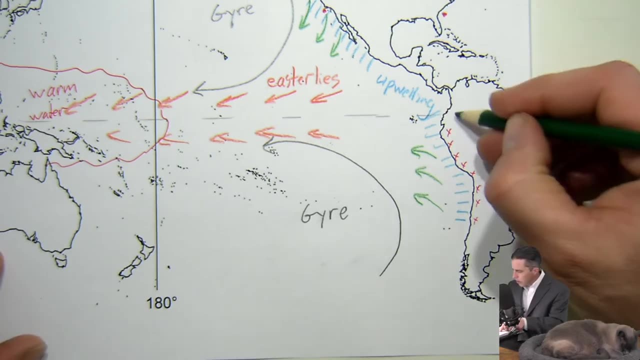 but when we talked about rain shadow, there are the Andes that are right along in here. Let me just sketch that out real quick. So the Andes are a mountain chain right through here And they're very- you know it's a tall chain of volcanoes. 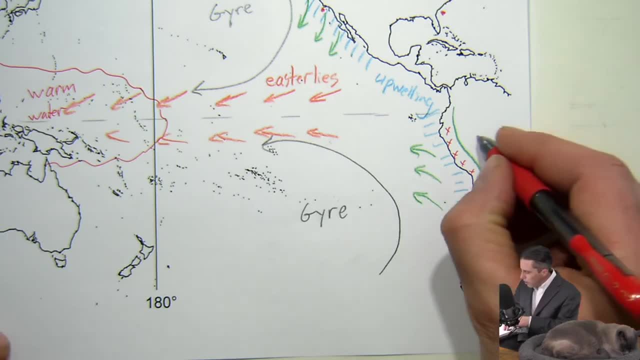 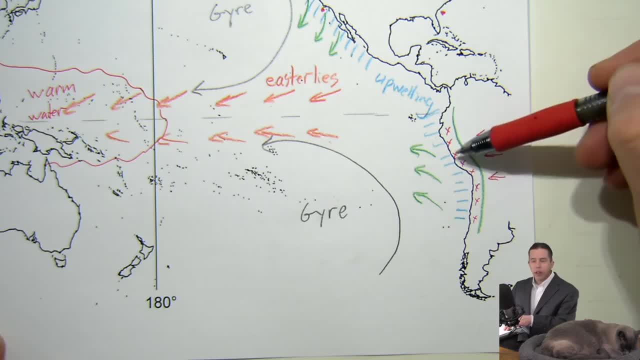 And this is very extreme. This is extreme rain shadow. There are areas here where it literally has not rained in over 10 years. Some of it's called the Atacama Desert- You may have heard of that, So these early people that lived along the coast here. 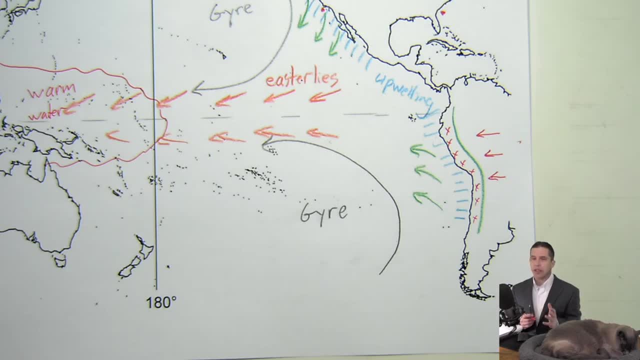 if you want protein, you really only have one option, And that's to get fish. Because it's so dry it's really hard to grow much of anything, So fishing became a livelihood for all the people that lived here, And they kept records. 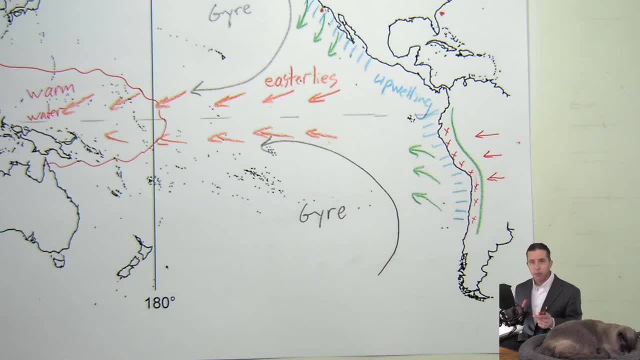 So for those people that lived Along this west coast of South America, you had to make your living as a fisherman. That was just the way it was. Well, they noticed, once in a while they would go out in their boats. 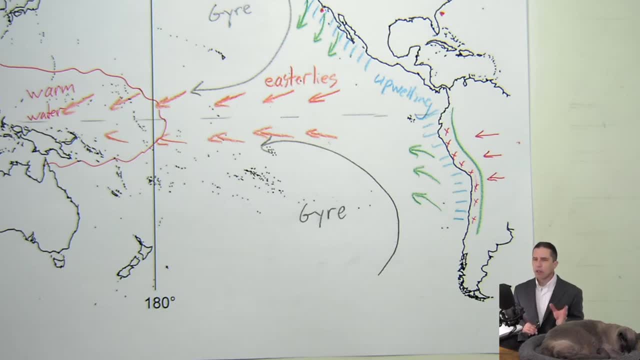 And this would happen, maybe kind of around Christmas time, near the end of the year, And they would go out and they would notice that actually this zone right in here, the water was unusually warm right through here And they would notice that the fish were gone. 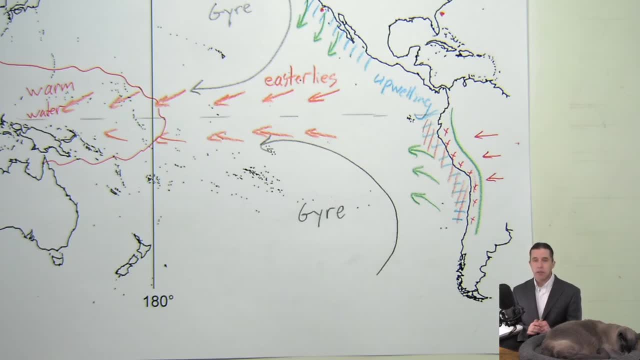 And this was a disaster because they depended on the fish And the fish wanted the cold water And the cold water had disappeared And they didn't know what caused this, But they seemed to notice that this often seemed to happen when he got close to Christmas. 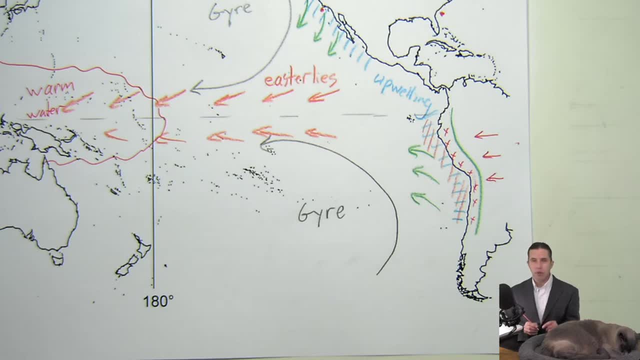 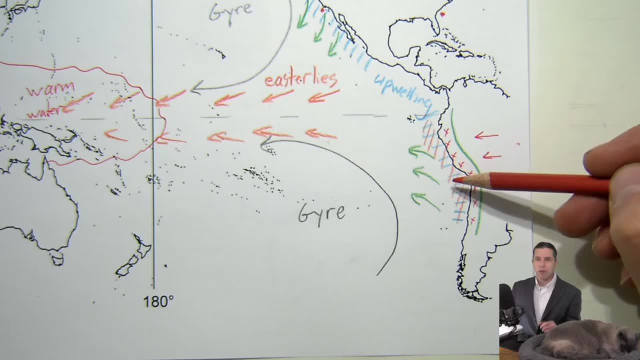 And it was possible, people were going to starve because he couldn't catch fish, maybe for six months or more. This is where the name El Nino comes from, And they named it that because of association with the time of year, of Christmas and baby Jesus. 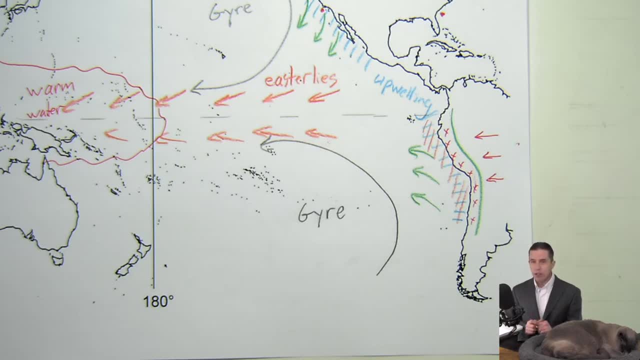 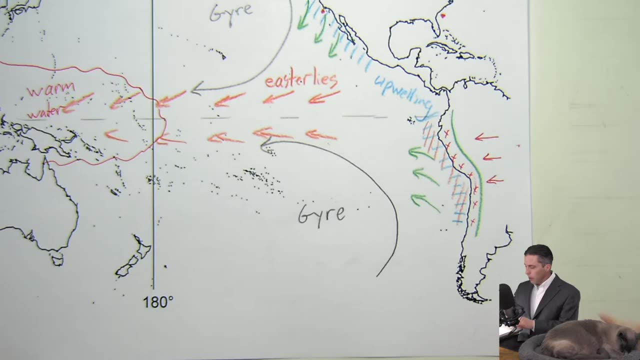 and all that good stuff, And so that's where El Nino actually gets its name. So what caused that Now? what we now know today- and they did not know this back then- is that something is going to shut this whole circulation system down. 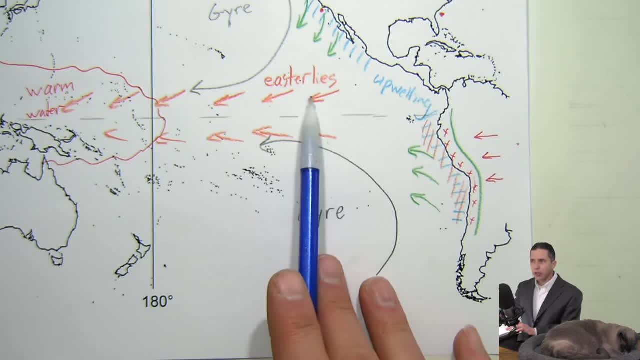 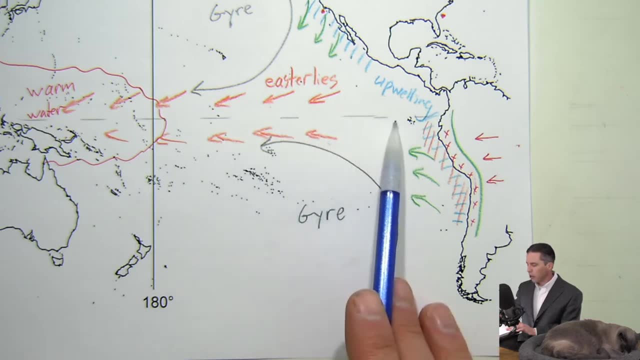 The easterlies are going to die. The easterlies die. The warm water moves back across the ocean. As the warm water moves back across the ocean, the upwelling dies. When the upwelling dies, the cold water stops coming to the surface. 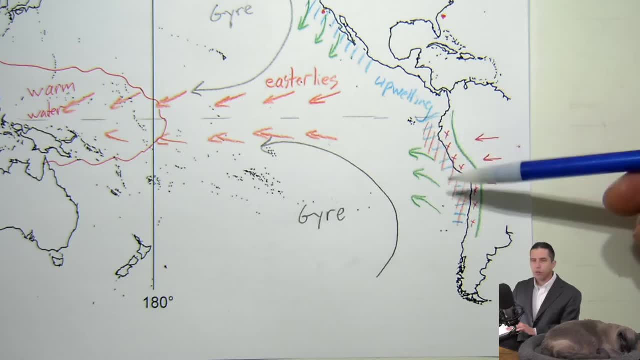 When the cold water stops coming to the surface, the fish go somewhere. I don't know exactly where they go, but they leave. That's El Nino. So to explain this, I'm going to show a couple of animations that explain what an El Nino event looks like. 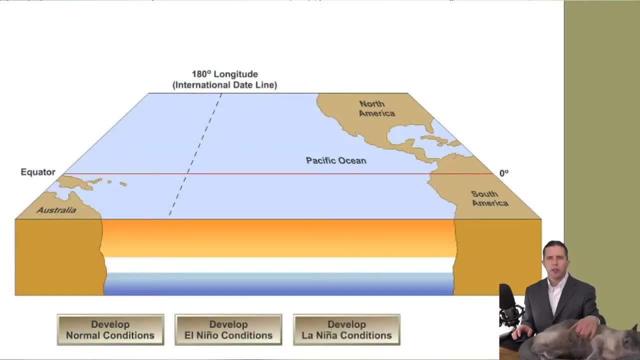 So this is a simple little animation that just explains. First we're going to look at what I just talked about, which is not El Nino, not La Nina, but just a normal condition. So here it's going to show. 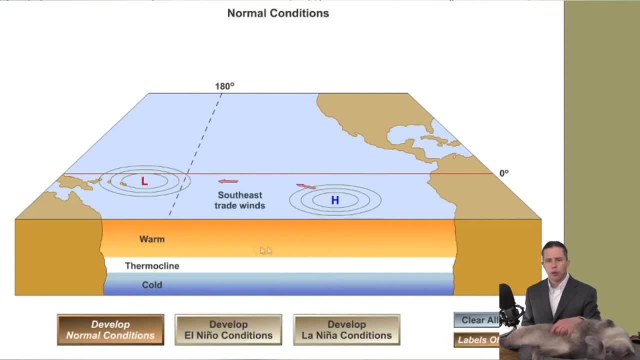 this is a cross-section through the ocean and the warm part of the water is this upper part, And here's our easterlies, also known as the trades, and they're blowing from east to west and they're going to pull up the warm water over here. 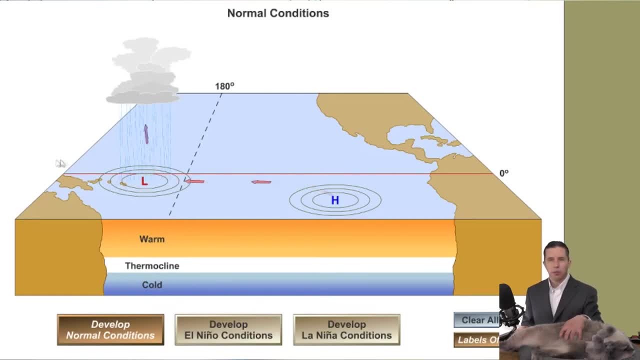 and you're going to get rising air because you've got this big pool of warm water and that's going to create a relatively low pressure, and that's going to create a relatively low pressure, and so that's what they're showing here. 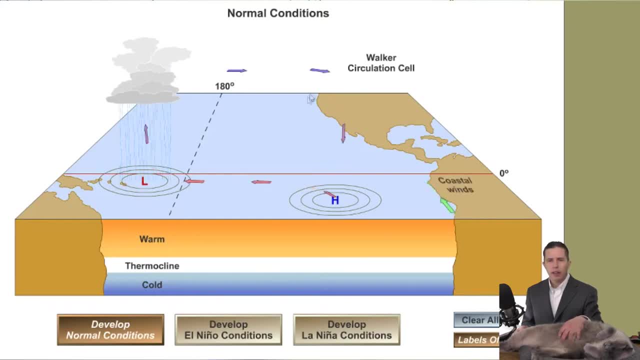 and a lot of precipitation. It rains over here every day And there is also air kind of sinking back out here and making a high. This is called the Walker Circulation Cell. Now, what they're trying to show here are those coastal winds. 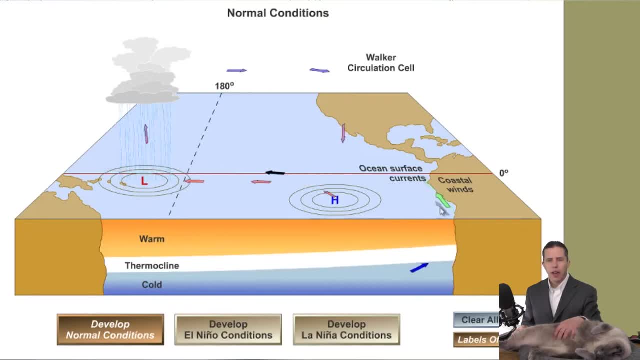 from the gyre coming up the coast and here's the upwelling. So they're trying to show that here comes that cold water and it comes up to the surface and then it gets pushed along the equator here and then you have this pool of relatively warm water over here. 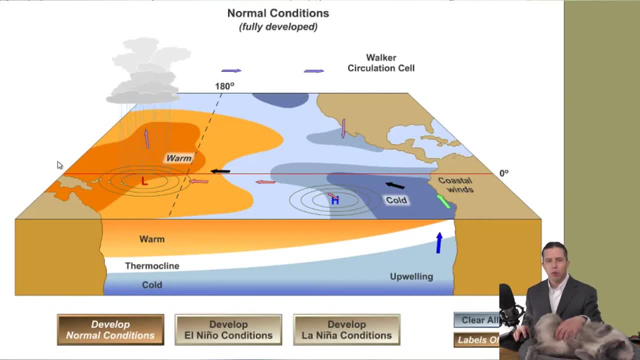 Now the animator got this wrong because you saw that the warm water started creeping in from the west over here, which is not right. We said that the warm water was pushed across the ocean this way, so they got that wrong. But this is kind of to show what I just talked about. 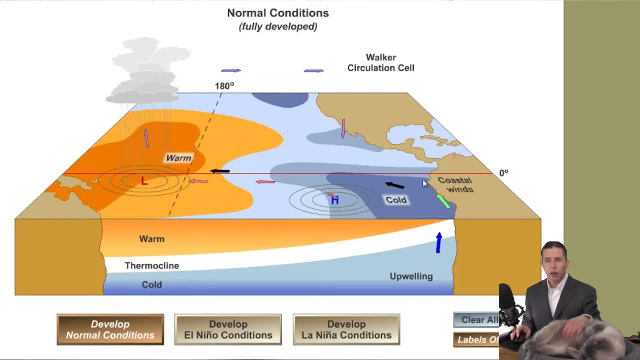 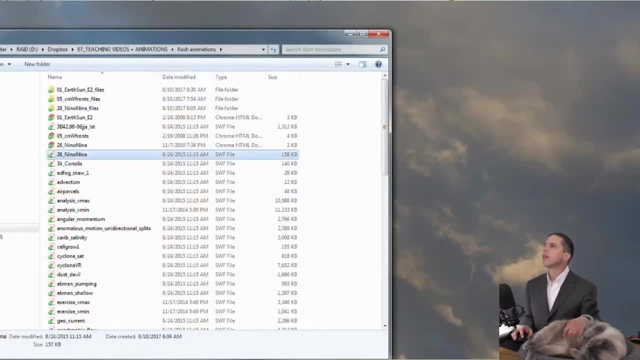 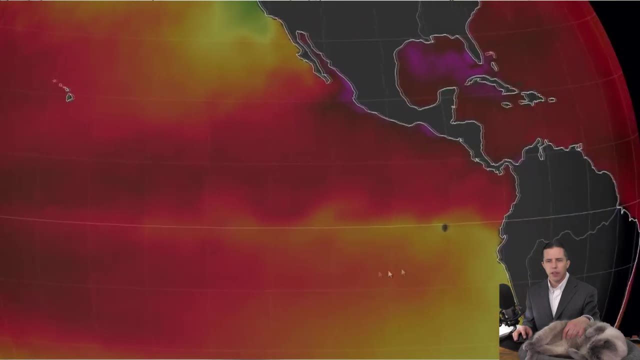 There should be not just cold water along the coast, but a little bit along the equator here. Okay, so we can see this If I go back. Okay, so now we're back to looking at sea surface temperatures. All right, so notice this. 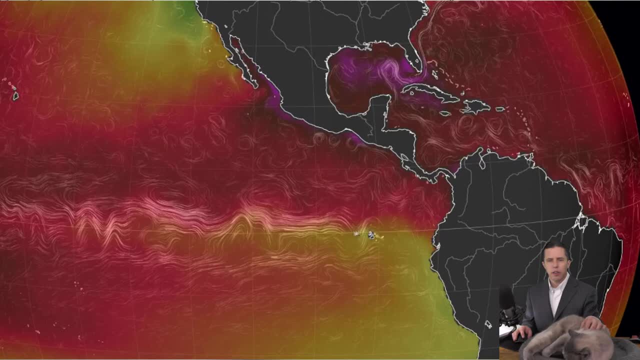 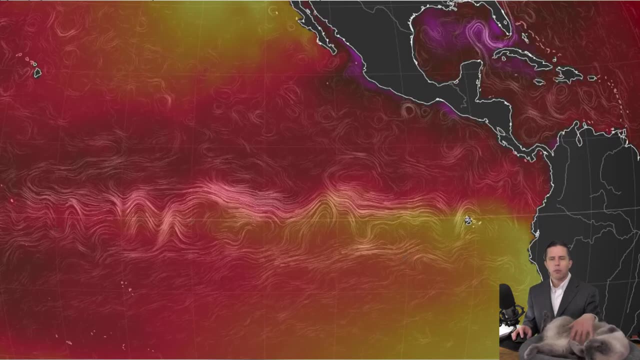 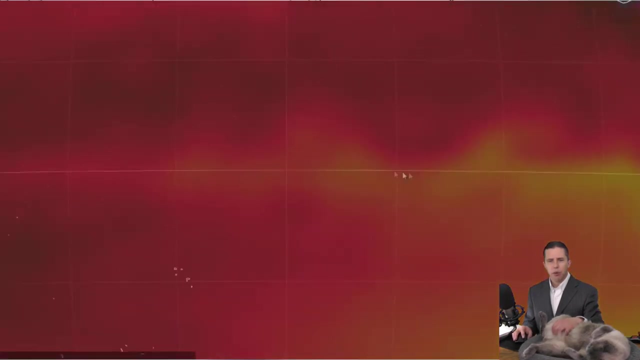 You've got this yellow, this cooler water, and there's this ribbon of yellow kind of along the equator. That's cooler water, that's being pulled up from the upwelling. The upwelling is happening down here And then it's being kind of pulled along with the easterlies. 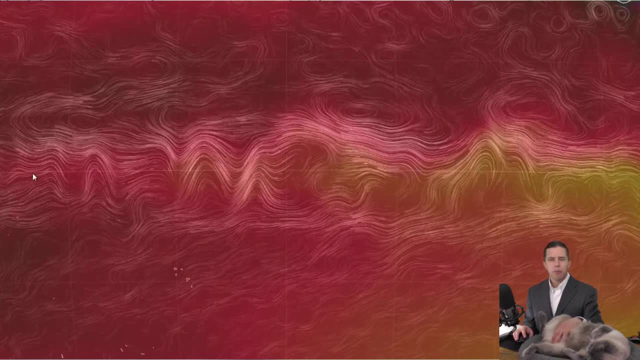 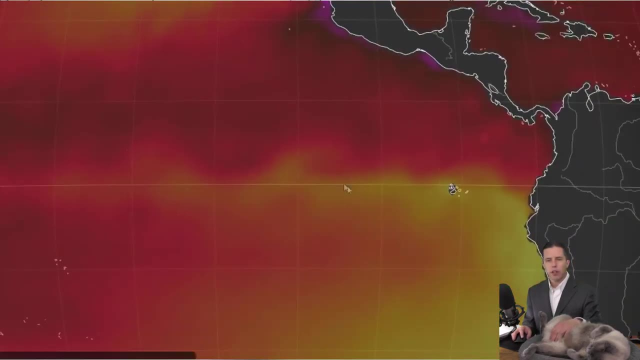 You can see the direction of the currents here being essentially pushed to the west over here, So that's why it's weird that you've got. some of the coldest water around here is right along the equator, where you'd expect it to be the warmest. 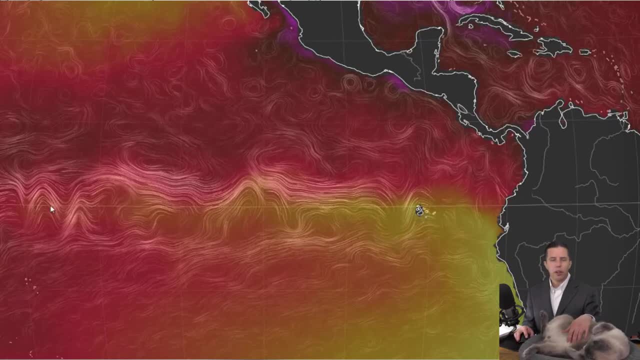 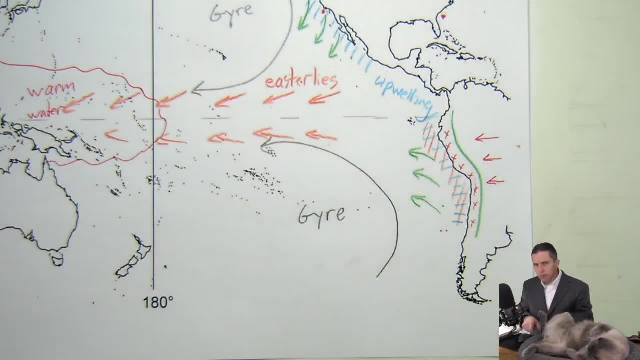 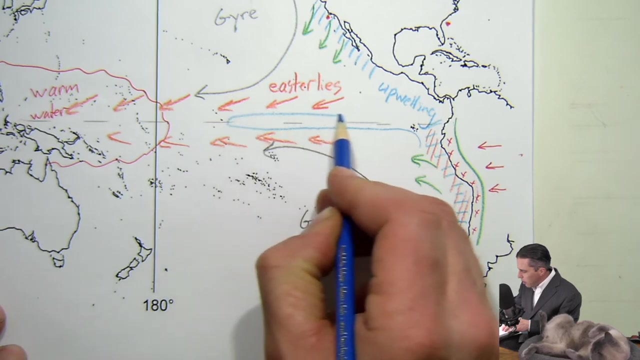 because the winds are pushing this cold water along here. Okay, so that's our upwelling, So I'm going to add that to our diagram. So we've got this ribbon of cool water kind of like in here, which I'll just shade. 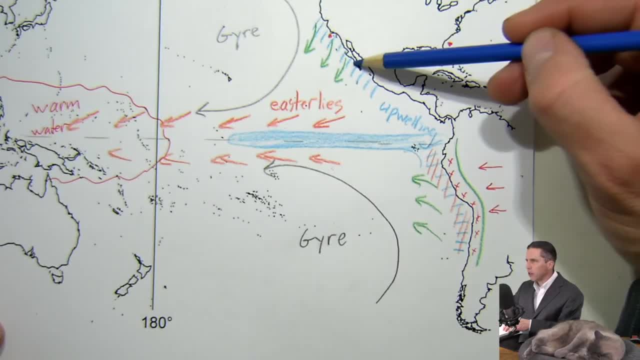 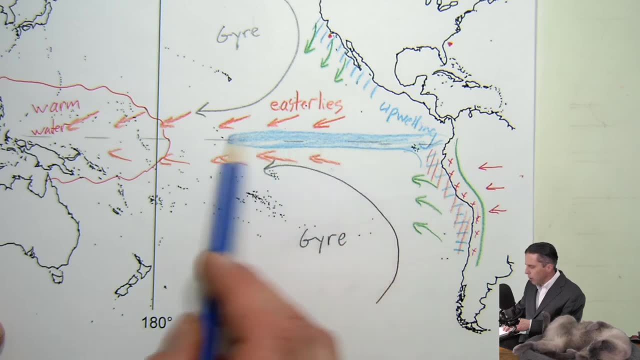 So, just to be clear, we've got cool water along the coast. We've got cool water along the coast down here, And the easterlies are pushing that along the equator, So we have this ribbon of fairly cold air. Okay. 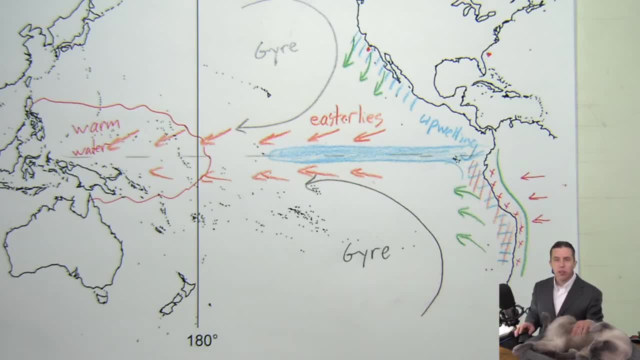 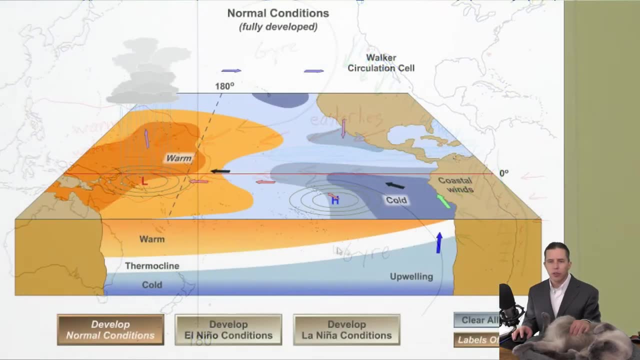 So this is not El Niño, This is a normal year. Okay, All right, So now we're going to go back to the animation. Okay, So this is where we left off the animation. So let's see what happens in an El Niño. 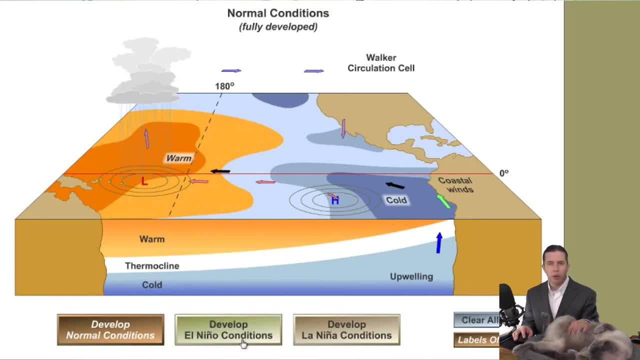 So the El Niño animation is going to start from this point, which is a normal year. Okay, So here we are. Now what happens is those winds, the trade winds, the easterlies, they die down for some reason. 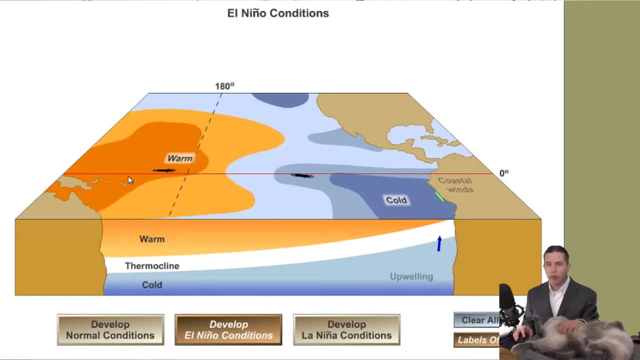 And in fact they might even reverse, And so the ocean starts to slosh back across the equator. This big pool of warm water works its way back across the ocean, The upwelling stops And instead of having cold water here and cold water along the equator, 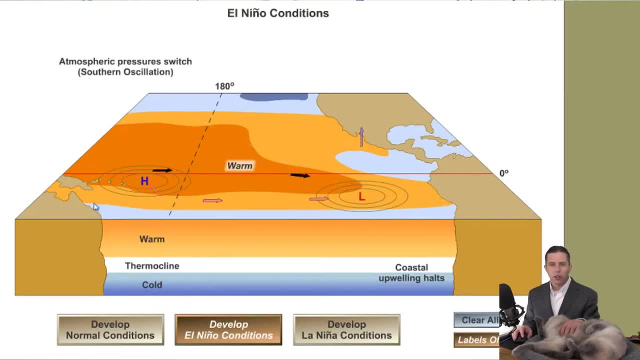 you have relatively warm water. Also, these two pressure centers reversed, So now you've got more of a low pressure over here And more of a high pressure over here. So these guys are now relatively dry And these guys are relatively wet. 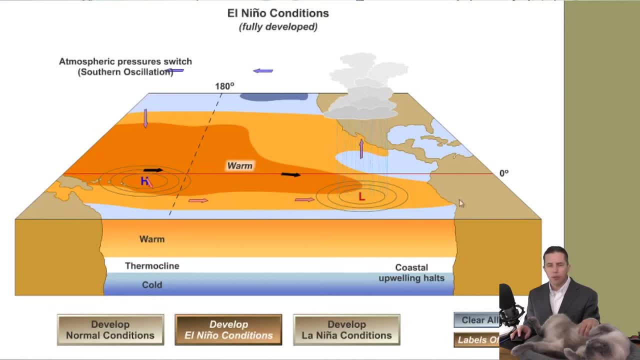 So this whole system that is now referred to as El Niño. So trade winds or easterlies, die. Warm water sloshes back across the ocean, Upwelling stops. You've got warm water along this coast, along this coast. 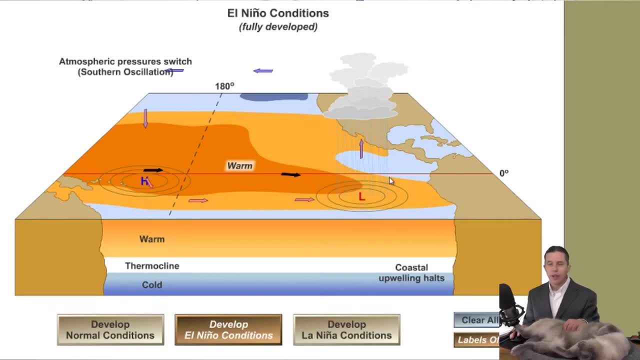 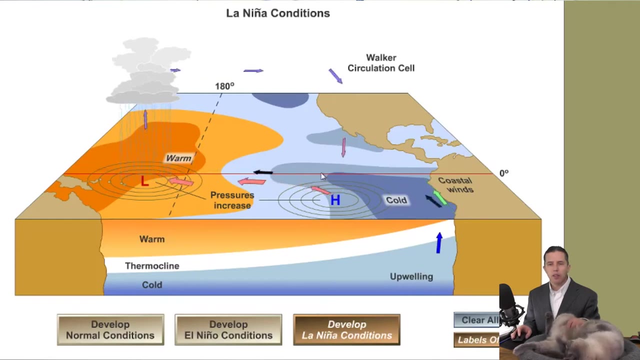 and along the equator, where you didn't have it before. That's El Niño. Now what's La Niña? La Niña, we're going to start again from a normal year. So this is a normal year, And what happens in La Niña is that the trade winds get stronger. 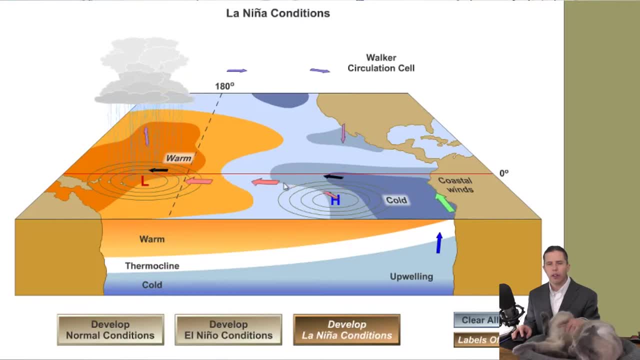 So this is. they're showing the arrows here, getting kind of fatter. So the wind is blowing. the easterlies are blowing harder than they were. This makes more upwelling than we used to have. That blows the cold water further along the equator towards the west. 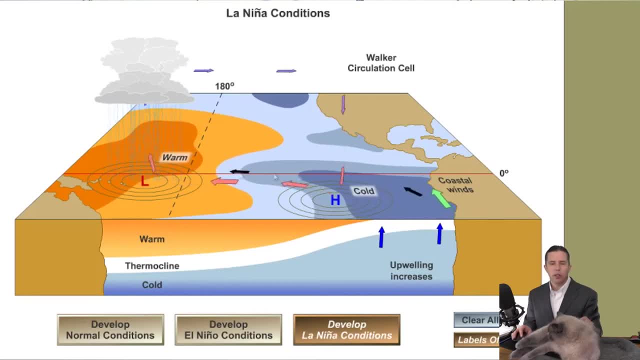 And you'll see that this pool of warm water shrinks a little bit And this pool of cold water grows a little bit. That's a La Niña condition. Now we know from these Chilean fishermen- and they kept records, for I don't remember how far back, but several hundred years. 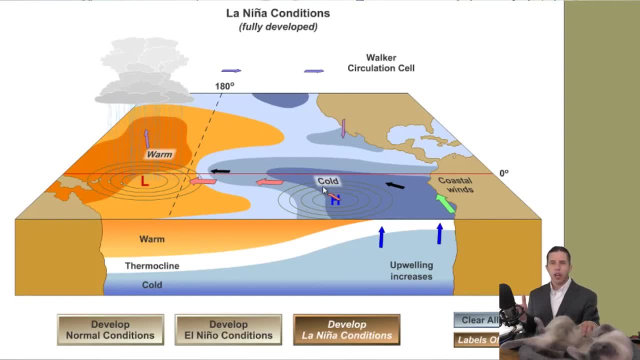 that this is a naturally occurring thing. So this was happening on Earth long before humans were having any effect on the climate, And it would happen maybe every five or six or seven years. they would have one of these El Niño events, And so it's a naturally occurring thing. 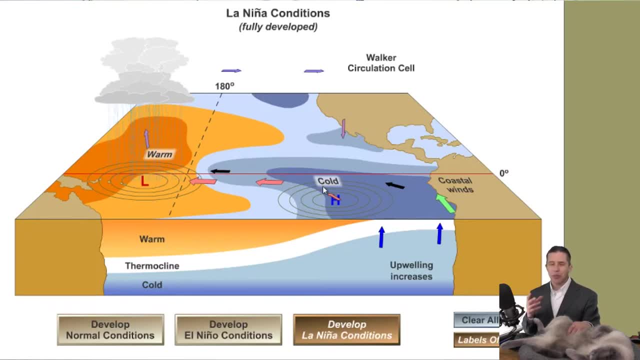 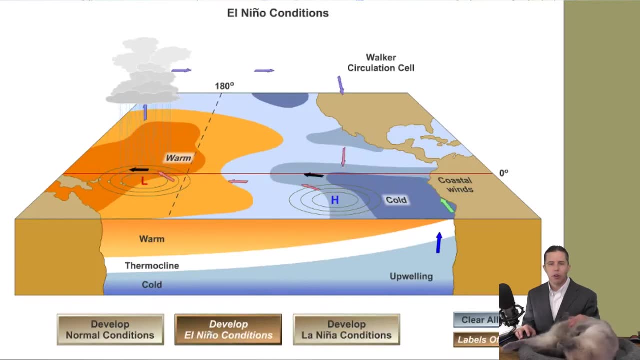 And for the most part, we can't really predict it. The way we predict it is we actually have. if I go back to my El Niño here, so let me pause it. So if an El Niño is coming, 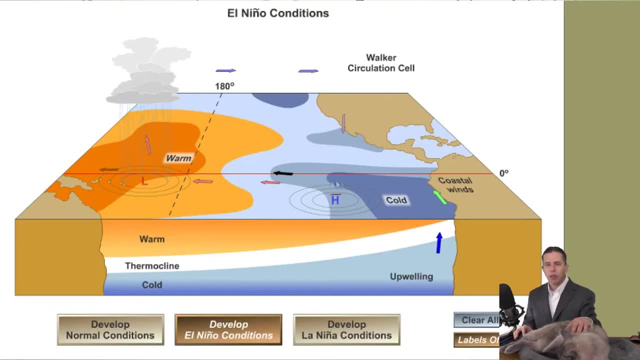 and we have some like ships out here or buoys with thermometers in them, or maybe we can see this from satellites. we can watch, we can notice it when this warm water starts to creep across the ocean right. So if an El Niño is going to happen, 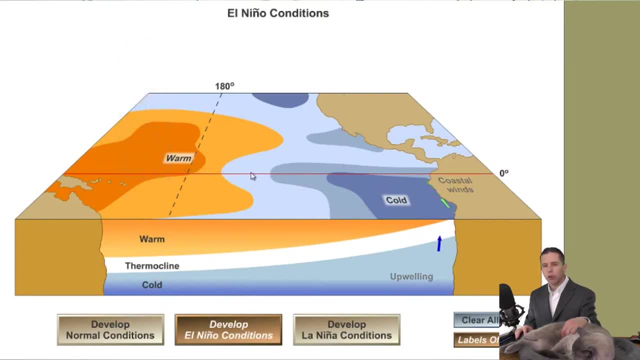 we can detect this warm water on the move, before it actually gets to the coast, So we can predict it that way. But we have no way of saying, oh, next year is an El Niño, or the year after that is an El Niño. 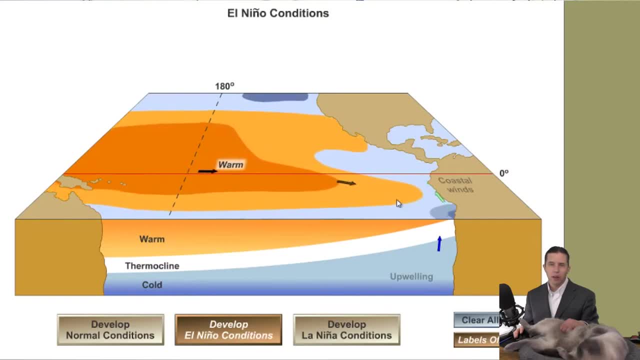 We can't do that. This is not a predictable process. When an El Niño happens, it happens. this condition lasts for several months. So it's not really weather and it's not really climate. it's kind of in between right. 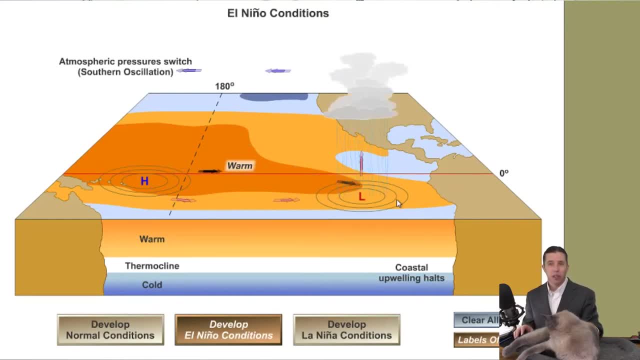 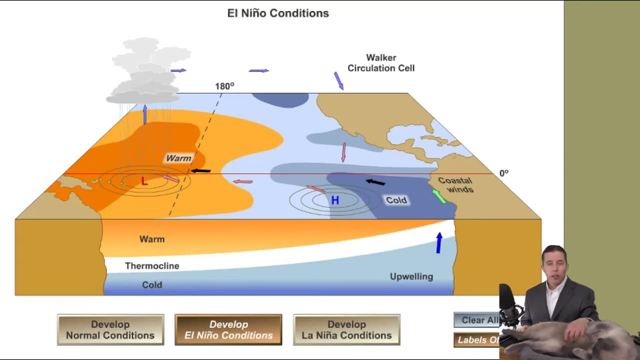 It kind of bridges the gap between climate and weather. It's a process that will change the weather for several months at a time. So El Niño is one of the two phases, with the other being La Niña. We generally refer to both of these together as ENSO. 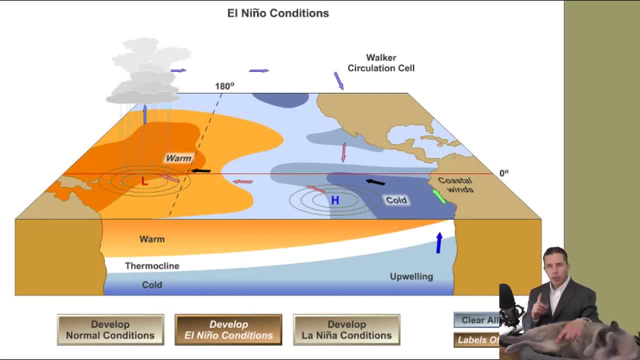 El Niño- Southern Oscillation. The Southern Oscillation refers to these two pressure centers that swapped. So again, this right here. this is a normal year, not El Niño, not La Niña. We've got a low over here, we've got a high over here. 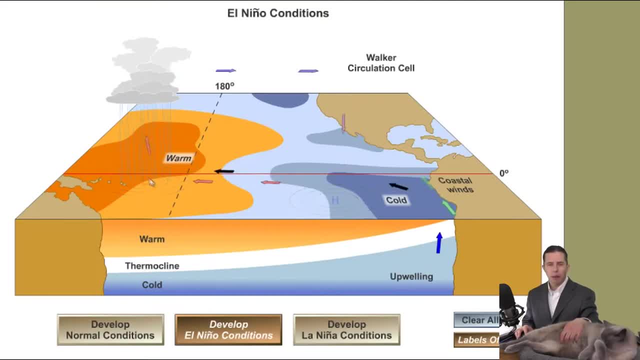 And in the El Niño, one of the things that happened is that these two pressure centers swapped places. That's what we call the Southern Oscillation. Okay, that's what it refers to, And we're not going to get too deep in this class about what all that means. 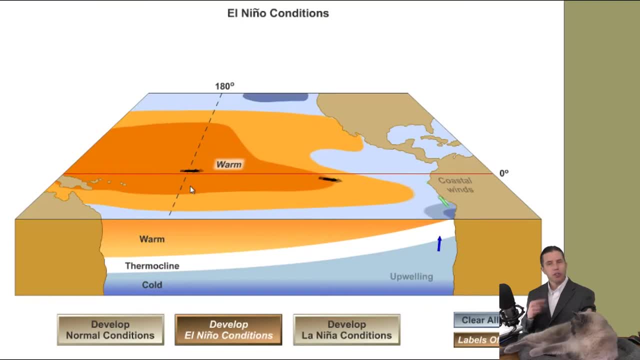 except to say that that's where the name comes from, So you'll hear this term ENSO. When you hear ENSO, just think El Niño and La Niña together. Like it changes between one and the other from year to year. 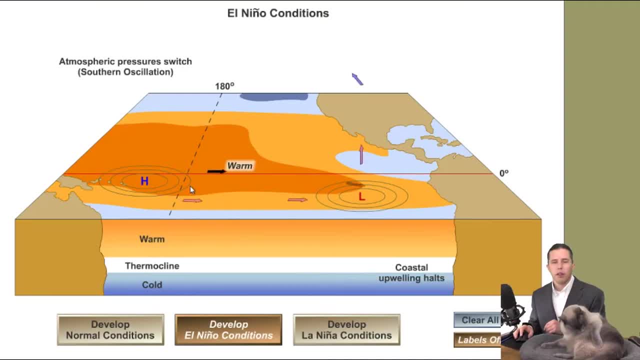 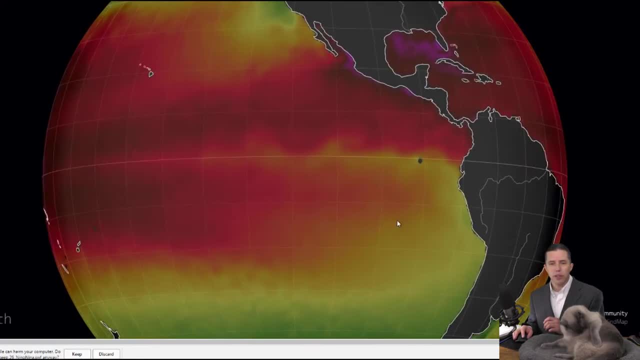 but collectively we just call this thing ENSO. So before we move on to the effects that El Niño has on our weather, I want to point out a couple other things with the SST maps. So when we talk about El Niño and La Niña events, 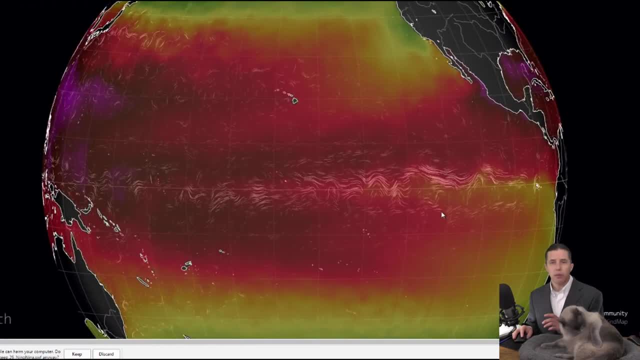 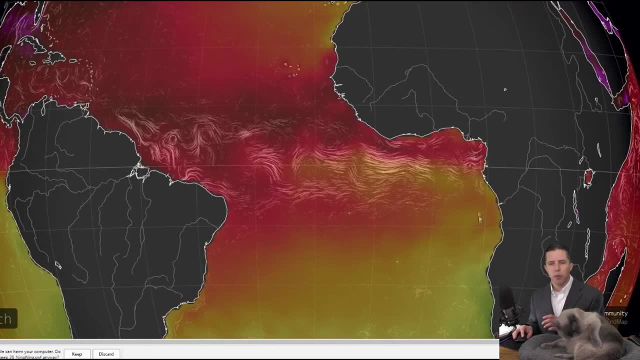 it's only happening in the Pacific Ocean, So apparently the Atlantic Ocean is too small. Now there's something similar going on here. There's some upwelling here. You can see this ribbon of cool water along the equator here. 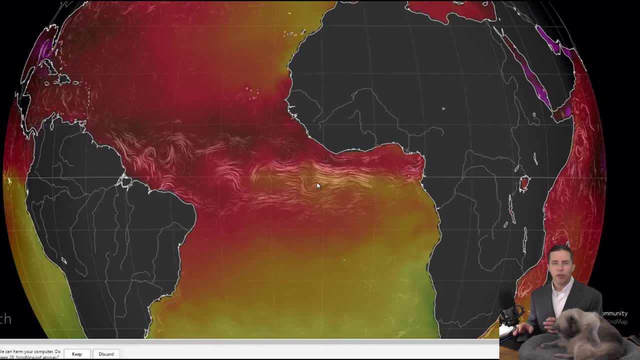 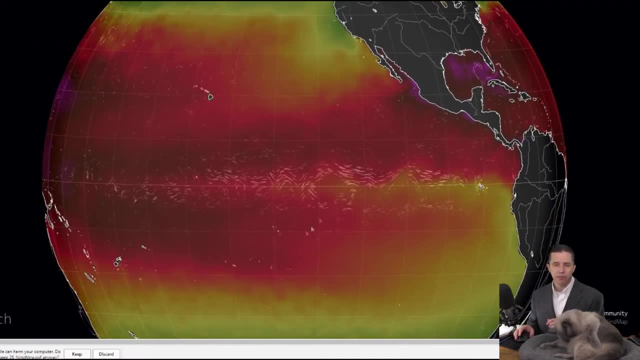 But when we talk about La Niña and El Niño events, it doesn't really seem to affect the Atlantic Ocean. It's only the Pacific Ocean where all this stuff happens. The other thing I want to point out is we also have some interesting ocean currents. 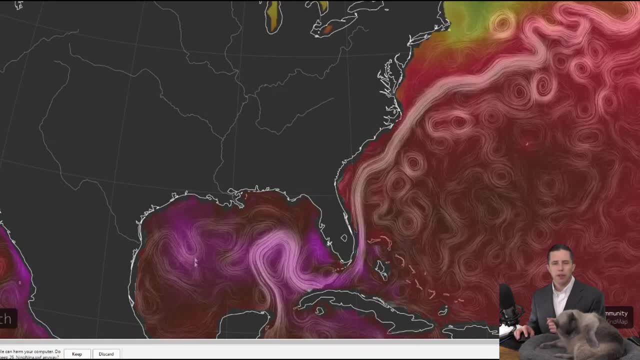 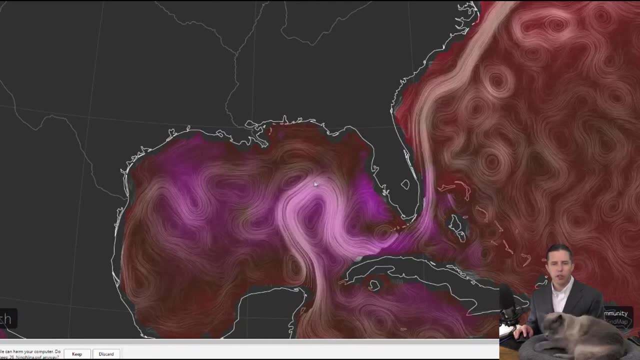 in our part of the world. So here's the Gulf of Mexico And again, this is a day in the summer, so we have especially warm water here in the Gulf of Mexico, And I want you to notice this, This stream, this current coming out of the Gulf. 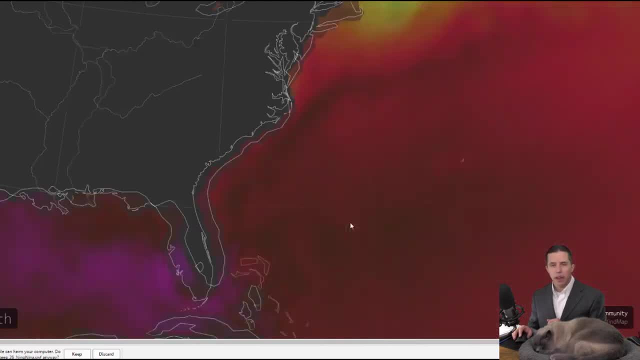 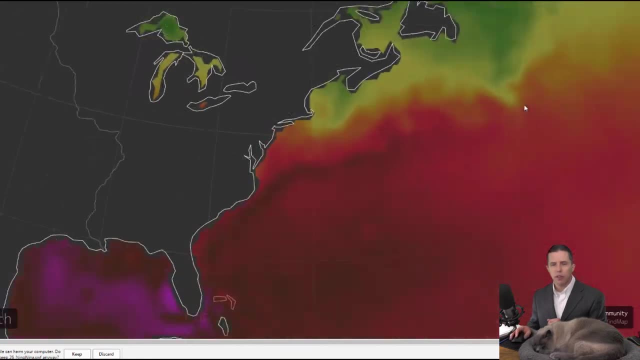 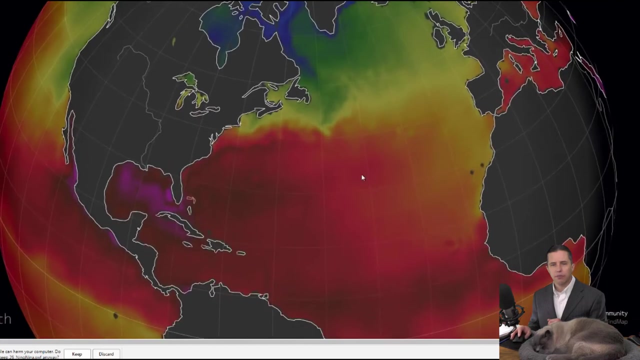 that's called the Gulf Stream And if we kind of follow where it goes, there's this ribbon of warm water that there's a bunch of eddies and stuff and it makes its way across the Atlantic Ocean. And if I kind of look at the big scale here, 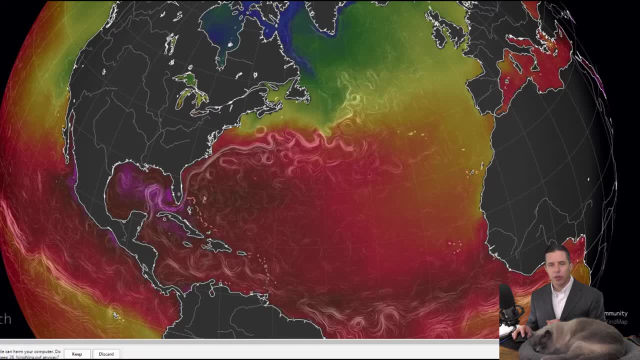 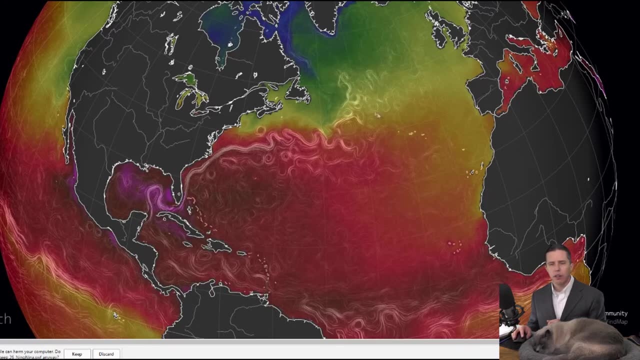 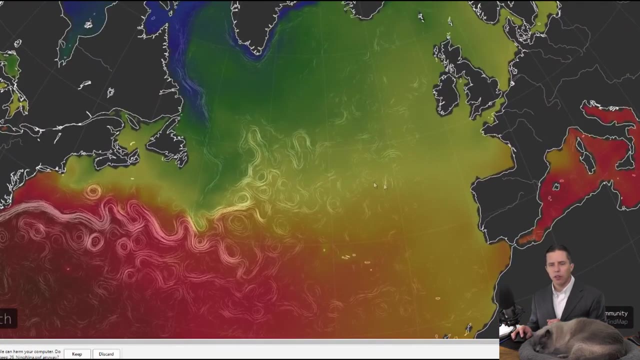 really warm water is coming out of the Gulf of Mexico, comes up the East Coast and it heads out to sea And it ends up actually over here by Europe. So this part of the ocean right here you can see, it's relatively kind of yellow in color. 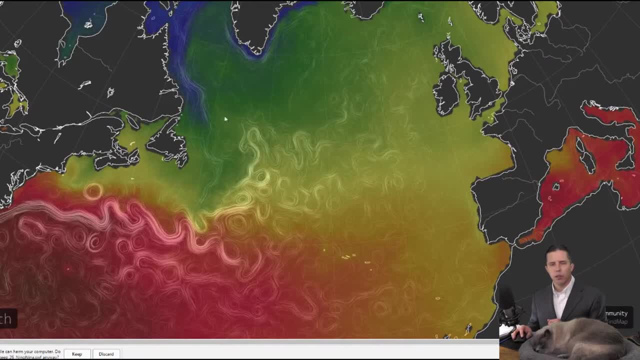 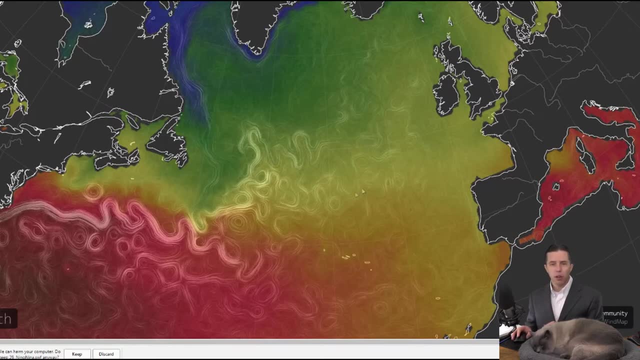 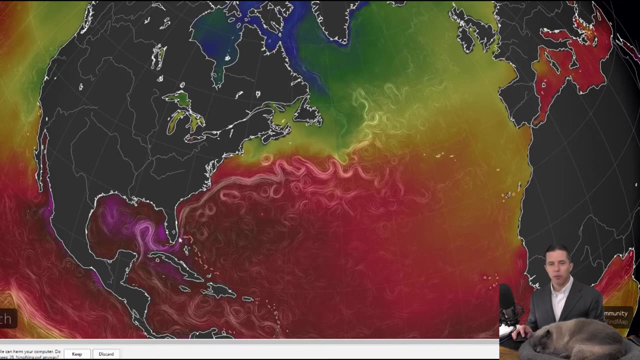 compared to over here, where you've got this colder green and blue colors. So this part of the ocean is being kept warmer because there is a current of warm water that's basically stealing our warm water from the Gulf of Mexico and pumps it out here. 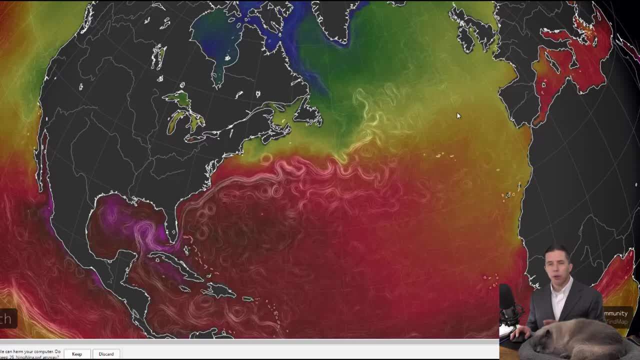 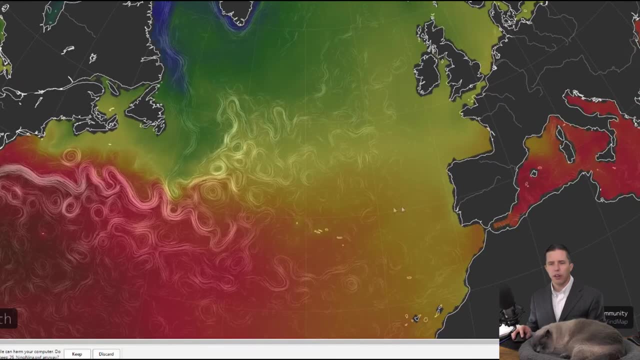 and dumps it out in this part of the ocean. Now, this is important because, for people that live in Europe, if you think about their latitude here, right here, if you follow this line of latitude across, okay, you're in the 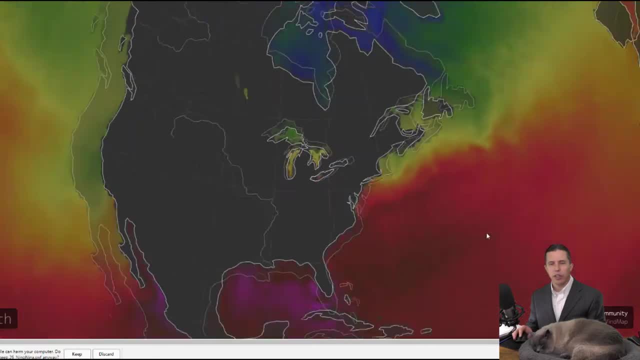 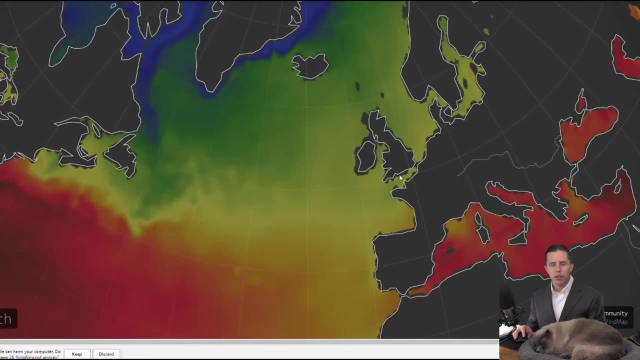 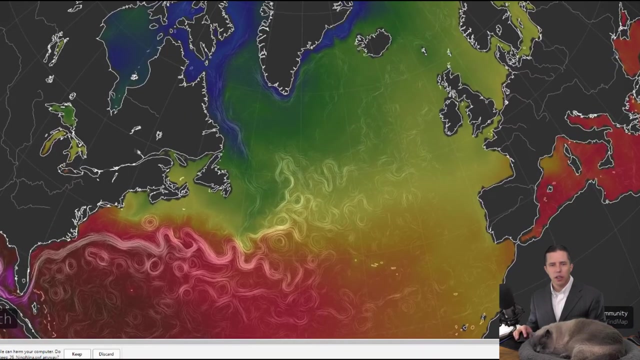 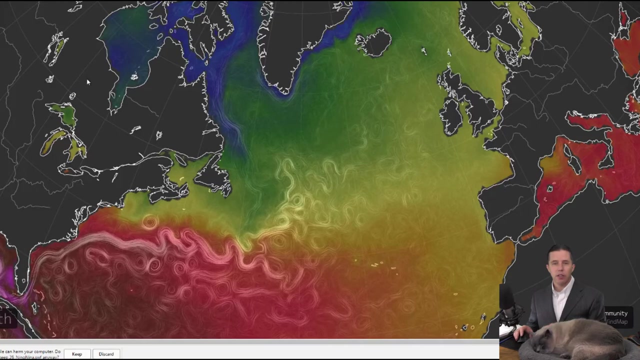 that would be equivalent to the middle of the United States. What if you went up, say to this one: Okay, so there's the UK and all that there. Follow this one across and you're in Canada, right? So what are the winters like in the middle of Canada? 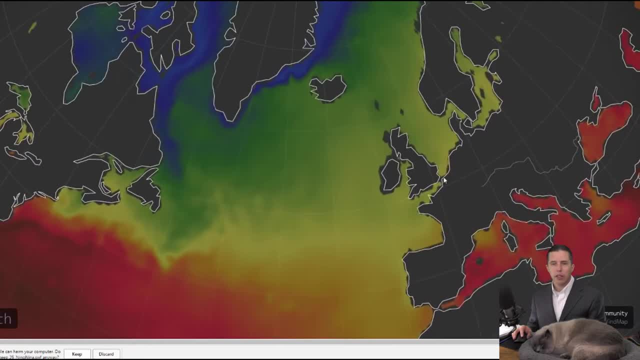 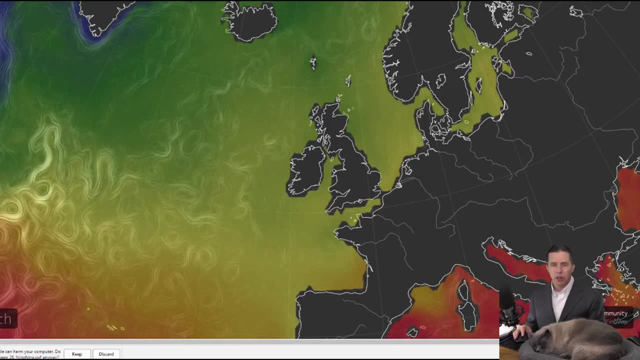 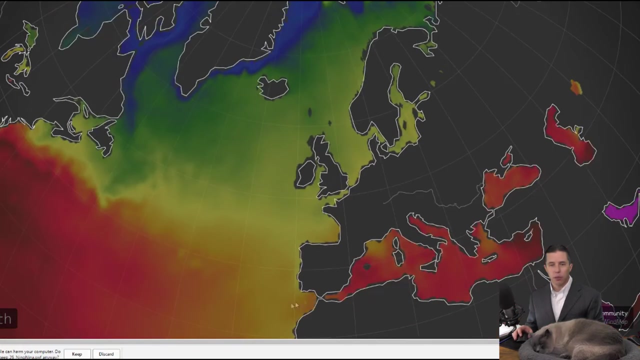 Well, very, very cold, But they're not nearly so cold over here in Europe, even though it's the same latitude. Why? Because this body of water, this part of the Atlantic Ocean, is warmer than it would be if it wasn't for the Gulf Stream. 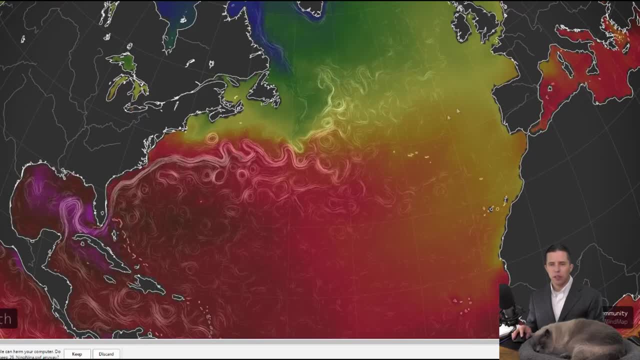 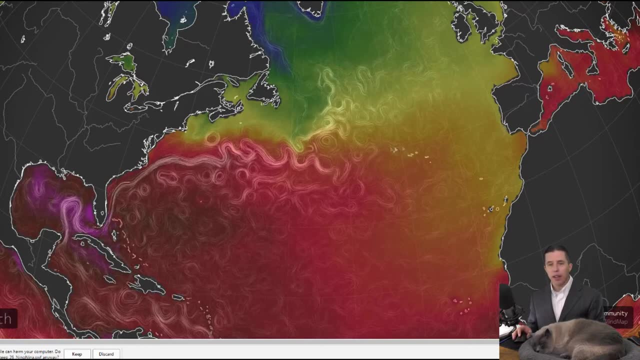 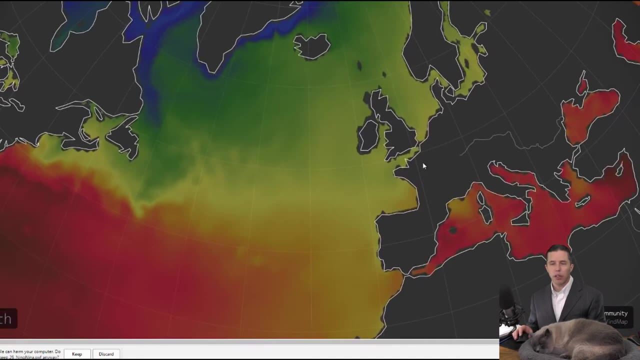 The Gulf Stream takes this warm water, brings it up, dumps it into this part of the ocean, keeps Europe warmer than it normally would be. In fact, if you shut this off somehow, Europe would be much, much colder. In fact, it would look similar. 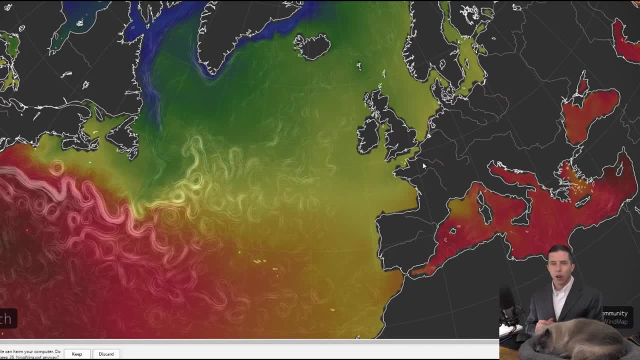 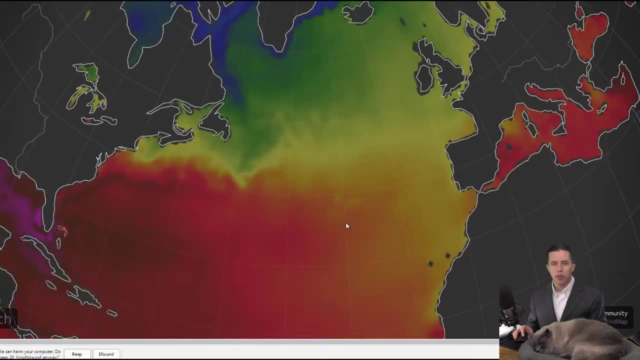 to what it looked like in the last ice age. So when we get to climate change, which is a couple weeks away, one of the things we're going to talk about is the possibility that this stream might shut down, And if it shuts down, 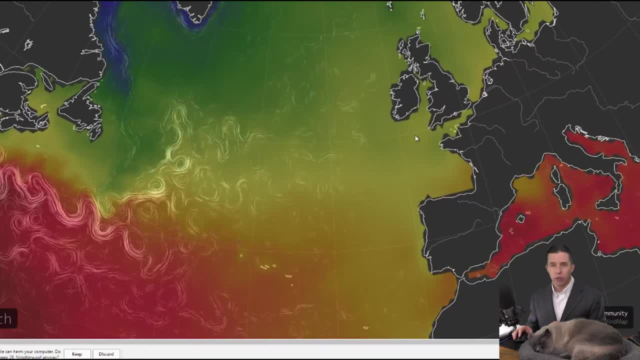 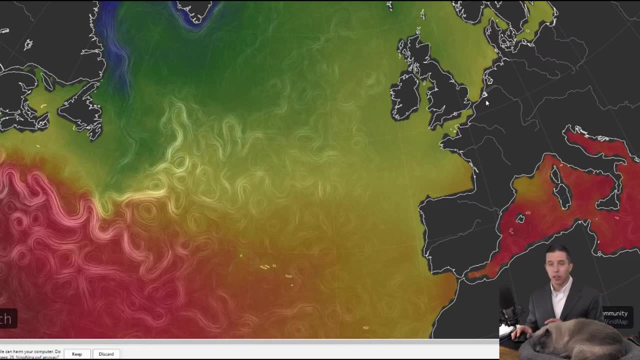 that's going to make Europe a whole lot colder. Okay, So that's a little counterintuitive. When we talk about the Earth getting warmer, why could Europe suddenly get colder? It has to do with this. I just want to point it out now. 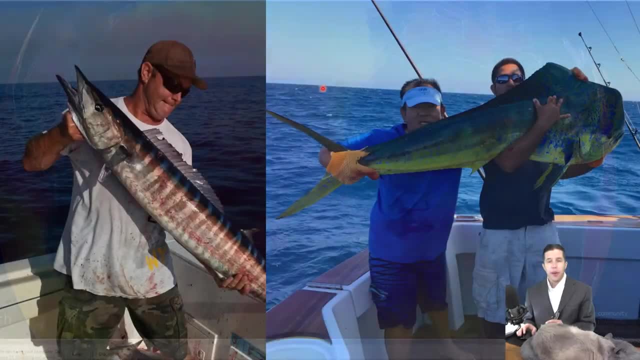 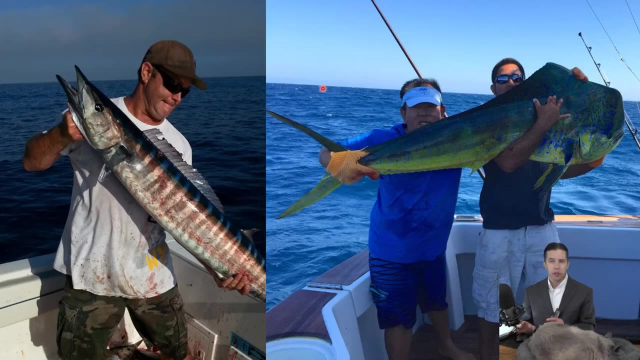 because that's what we're talking about. So if we have an El Niño or La Niña event, we can get some really radical changes in the weather and in ocean temperatures, depending on where you live. So, for example, these guys are catching tropical fish. 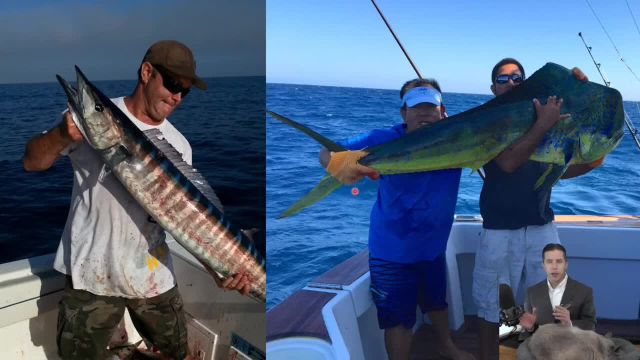 off the coast of Southern California. Now, we just said that the water off the coast of California is really cold because it's from the bottom of the ocean, But during an El Niño that upwelling stops and that warm water sloshes back across the ocean. 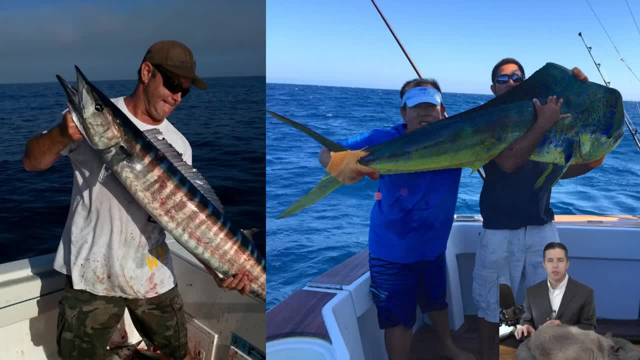 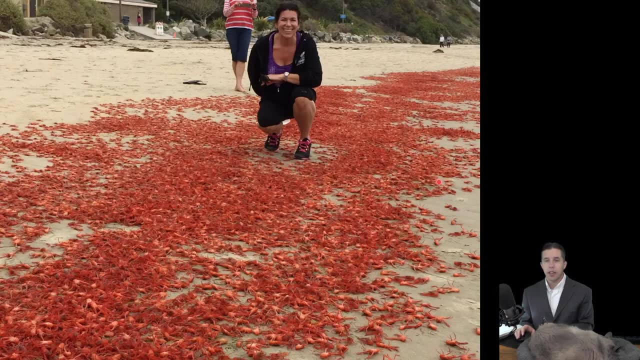 and the tropical fish follow that, And so these guys are catching tropical fish in a place where it's normally really cold water. A lot of times, animals just can't handle the changes in water temperature, So these are jillions of dead crabs. that couldn't handle the warmer water of El Niño. And again we're in California. They've washed ashore here by the millions And you got to wonder how bad this smells after a few days of this, But during an El Niño. 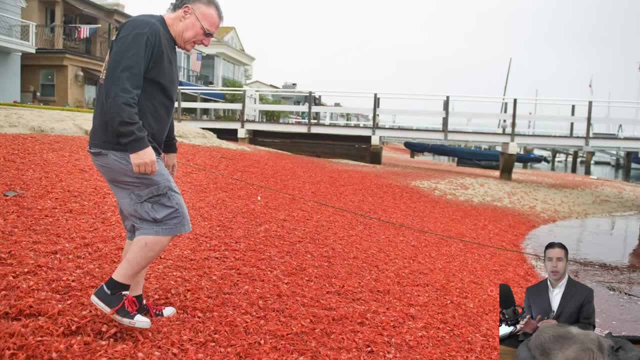 that sudden change in temperature can really kill a lot of animals that have adapted to growing in an environment with, you know, pretty cold water- Like I said, it's usually not too much warmer than freezing most of the time- And suddenly you have this warm tropical water. 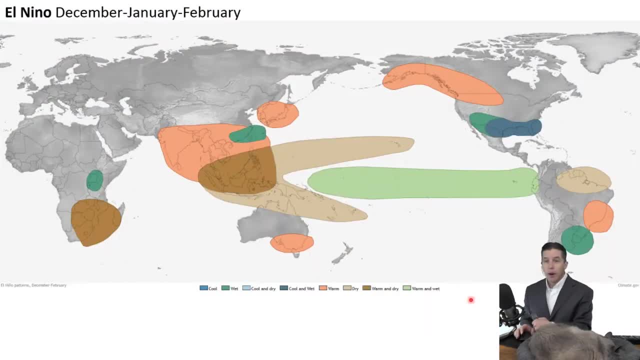 and a lot of animals can't handle that. Now the El Niño event itself, or La Niña, is affecting this area right near the ocean or near the equator, And you'd expect well, the weather through here will probably be different because of this. 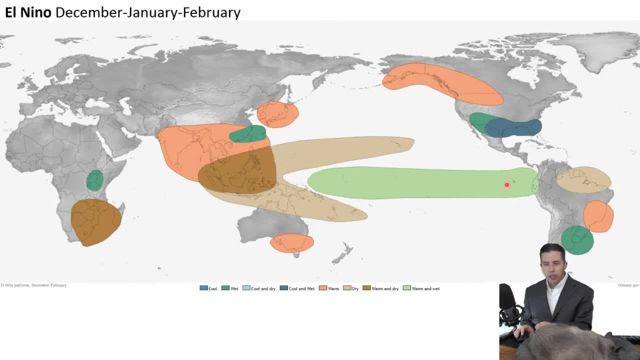 But what you may not expect is that this change in an event down here triggers all kinds of changes of weather all over the world. So here's a map showing the types of weather changes that occur during an El Niño and in the winter. So December, January, February. So, just to reiterate, when we have an El Niño or La Niña, it lasts for several months. Okay, so it may last six months or eight months or four months, And so during that time it will have effects on the weather. 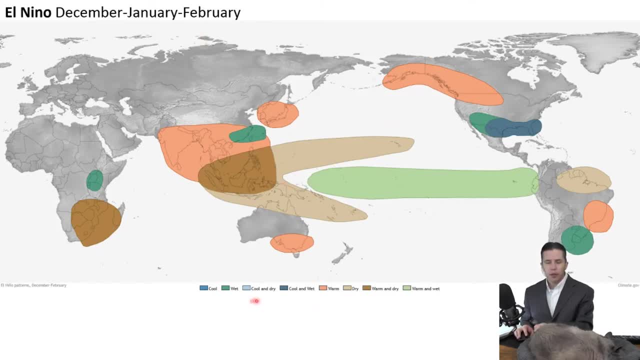 So, for example, you may not be able to quite read the key down here, but along the equator it says warm and wet. Okay, that makes sense, And at El Niño you've got warm water sloshing across. 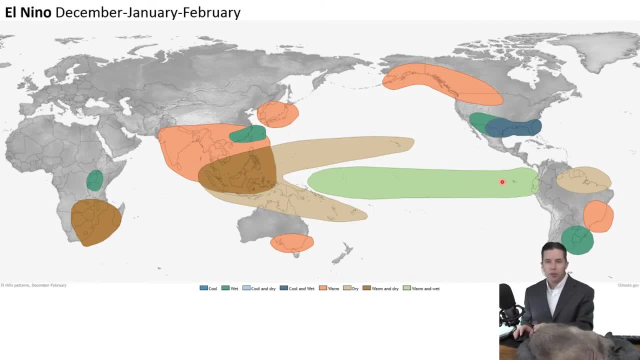 That should make it warmer and give you more precipitation. But then, for example, up here, it says it's going to be warmer, or warmer and drier, Or places where the precipitation increases. And notice what's happening over here. We've got a green zone that says wetter. 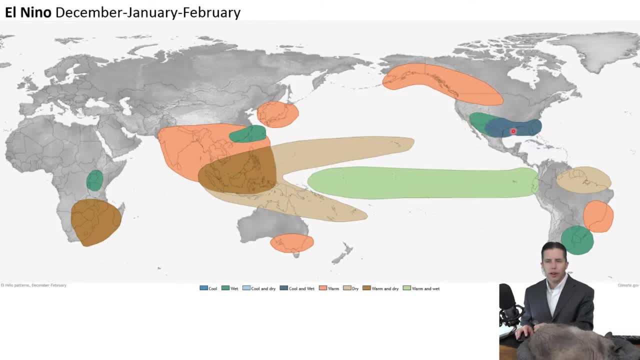 And we've got kind of a bluer zone that says cool and wet. So this change here is affecting things all over the planet And for us, as in New Mexico, we're in this green blob, So we're going to explain that in a little bit. 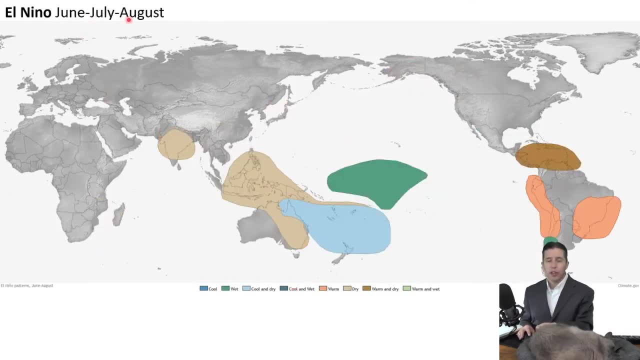 Now here's El Niño- June, July, August- And notice that we see some changes in different parts of the world Right. so down here it's cool and dry, or what have you? But notice that for the most part, 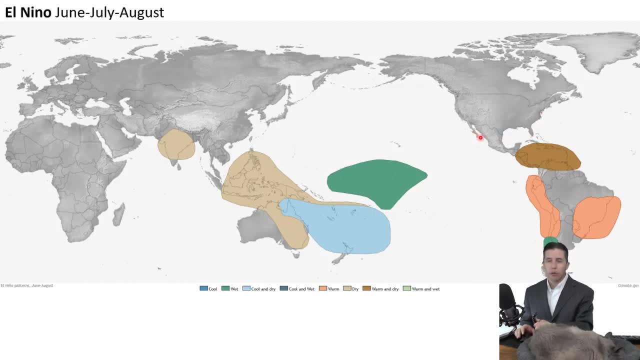 not much is changing in North America in general, and especially not in the United States. So for us, if we have an El Niño, it affects our winter precipitation and our winter temperatures, And we'll talk more about that in a second. It does not seem to affect us in the summer. Okay, so keep that in mind, that El Niño really affects our winter time. If we have a La Niña again, that's going to make this. you know the definition of La Niña. 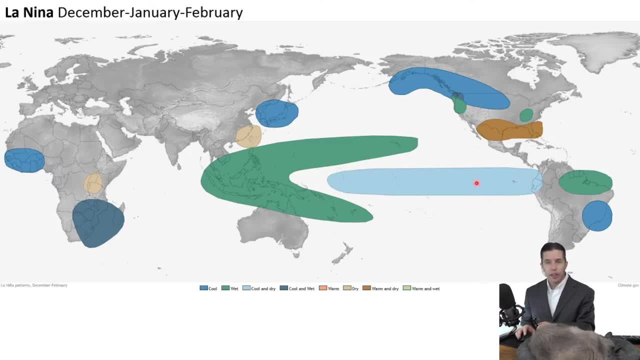 is, the winds here are blowing stronger from the east, which makes this colder. Okay, so if it's colder, you'd expect it to be cooler and drier. That makes sense, But it also has effects all over the world. So, for example, up in here, 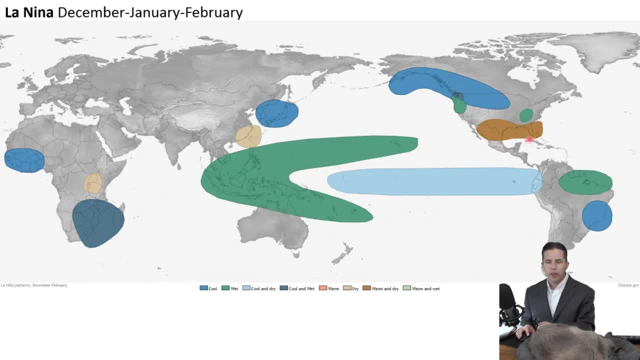 it says it's making it wetter, And down here it's making it drier. Okay, and so we're actually, you know, we're kind of getting up here in New Mexico where it's going to have some kind of effect. 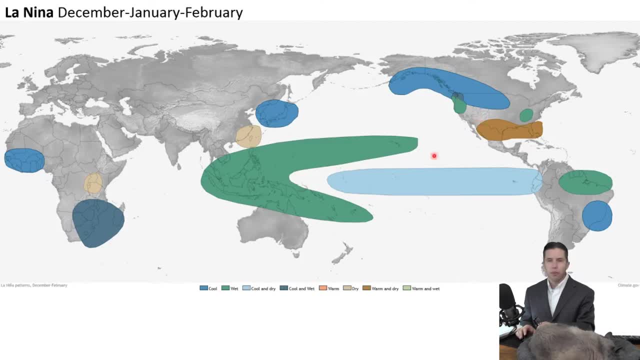 for us too, which we'll talk about in a second. So the point is, you're only changing this, but somehow it's having effects all over the planet. So why might this be the situation? Oh, and before I forget, 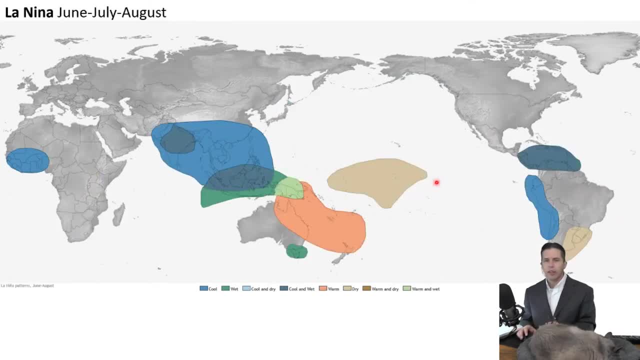 if I look at La Niña again in the summer, we see really nothing changing. Nothing changing here in the United States. Okay, so El Niño or La Niña doesn't really affect our summer weather, at least not that we've been able to determine. 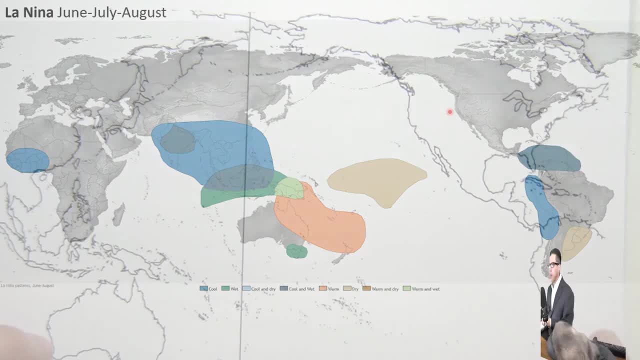 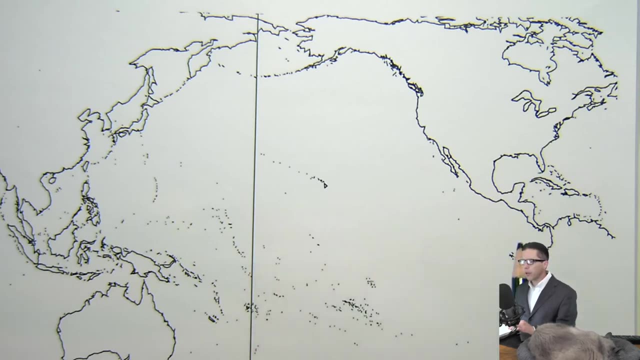 Does affect our winter weather. So how is it that a change in the temperature along down here by the equator can have effects all over the planet? Short answer is that it's really complicated, But there's one thing that we can learn about in this class. 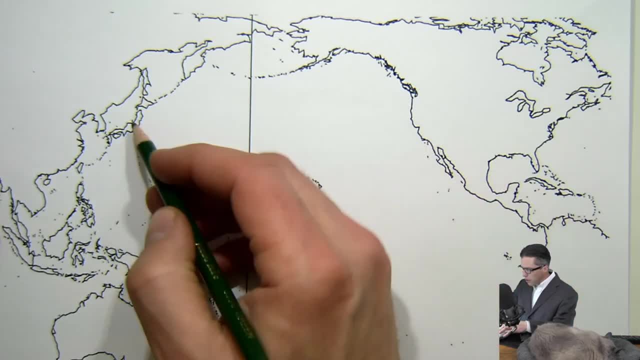 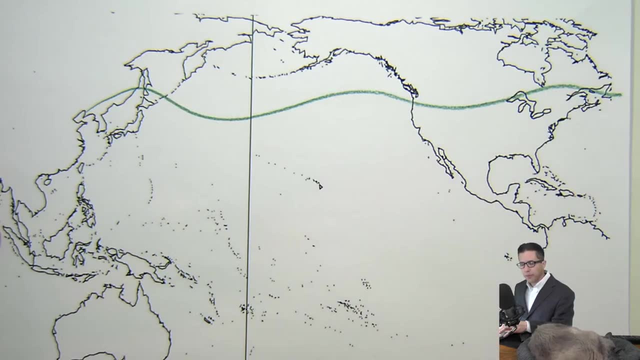 that we've talked about before. So we talked about the polar front, right? So let's imagine the polar front is going kind of through like this on a normal year. So to remind you, the cold air is up here, the warmer is down here. 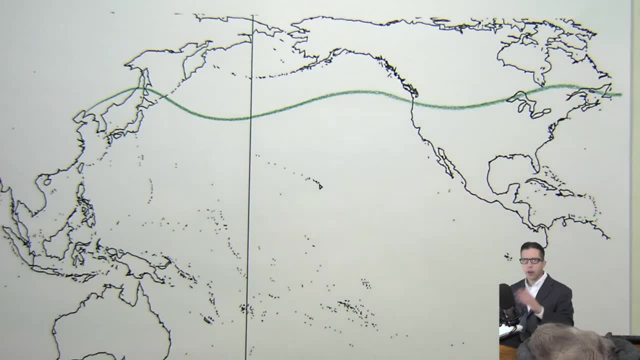 and the middle latitude. cyclones basically follow this path And it's always changing right. There's these curves and the whole thing we've talked about with the Rossby waves, But in general the storms are kind of coming in through this direction. 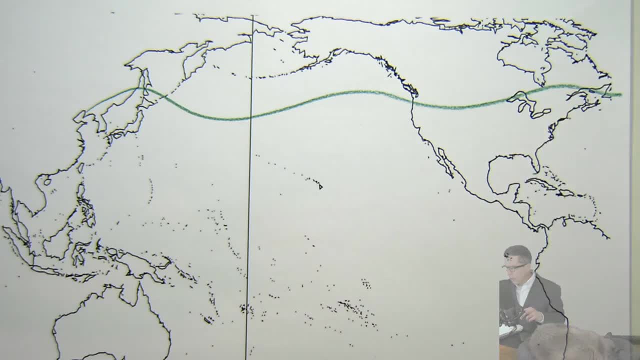 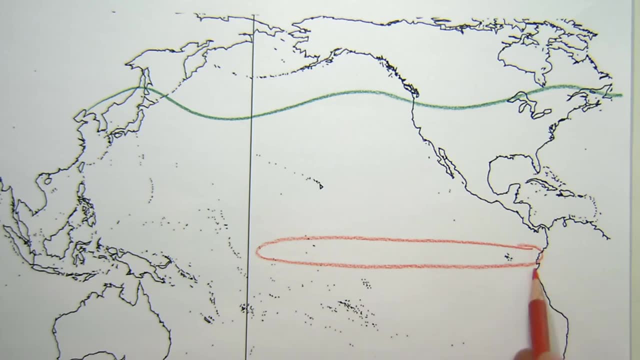 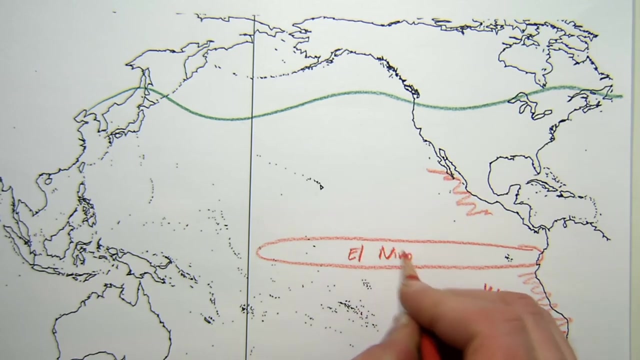 Now let's say, we have an El Niño. So an El Niño means that we have warmer than usual temperatures here and here and here. Right, This is, in an El Niño, warmer than normal. Okay, so let me just write this out here. 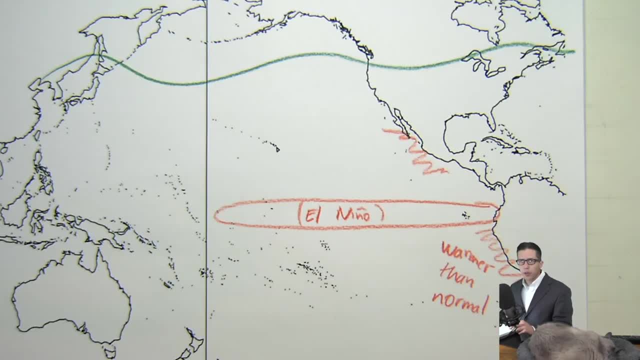 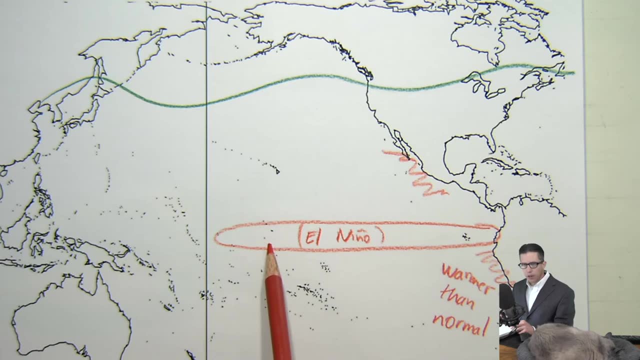 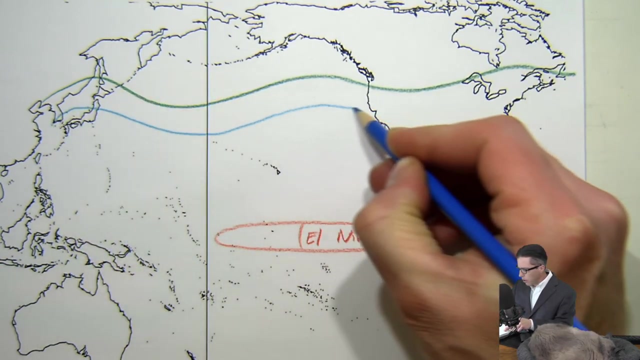 Okay, so in an El Niño event it's warmer than normal. Now, the fact that there is a pool of warmer water here will cause the polar front to shift positions a little bit, And it will actually shift a little further to the south. 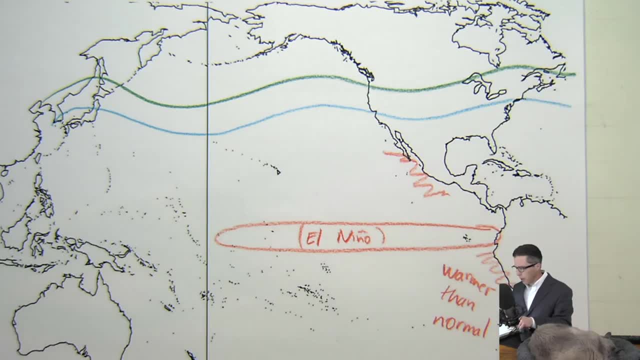 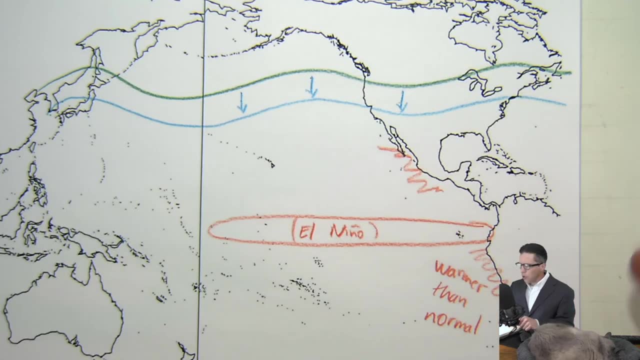 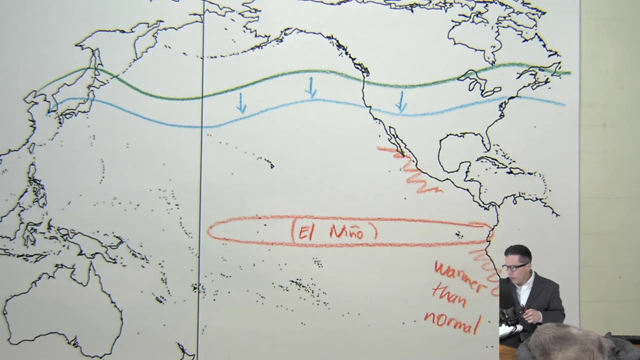 I'm exaggerating this greatly, just to make a point. So the polar front shifts a little further south during an El Niño winter than a normal winter. So if we think about mid-latitude cyclones, right The mid-latitude cyclones. are forming along the polar front. Where are they going to go? Well, during an El Niño, because the polar front shifts further south, then the mid-latitude cyclones shift further south. So what that means is in a non-El Niño year. 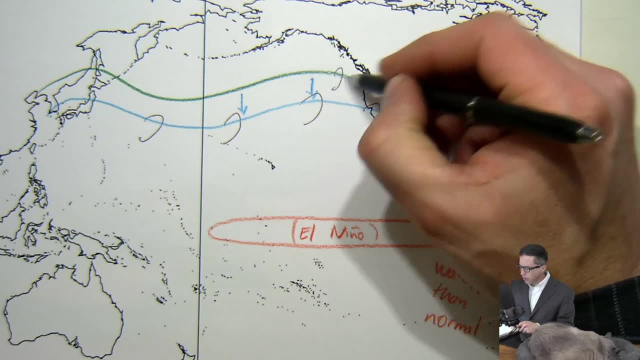 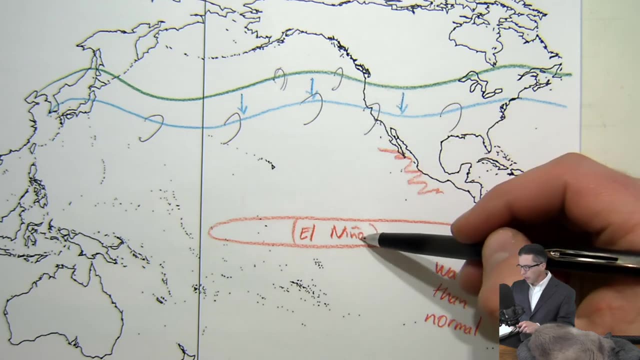 just a normal year, you'd expect the mid-latitude cyclones to kind of be following, say, the path of the Green Line coming up into the Pacific Northwest. But in an El Niño year this whole thing will be shifted down and the Pacific 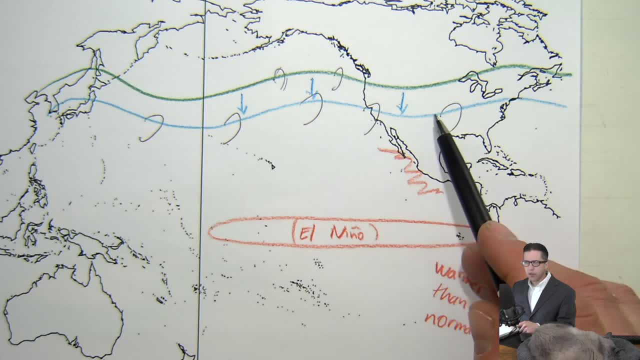 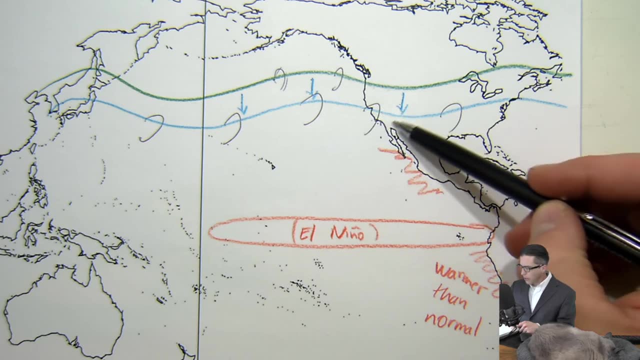 I'm sorry. the mid-latitude cyclones will be traveling further south. Well, what's further south of this Green Line? Well, we are. So us, as in New Mexico, will be in a position where we are more likely to get mid-latitude cyclones. 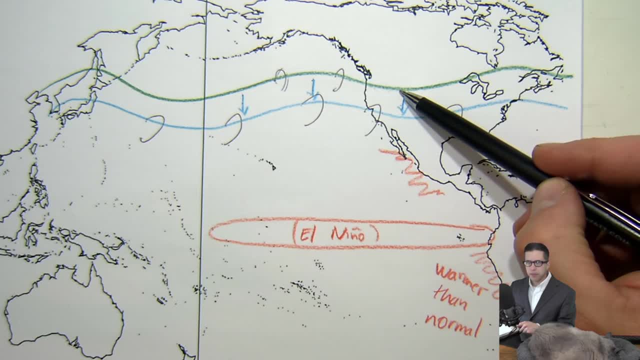 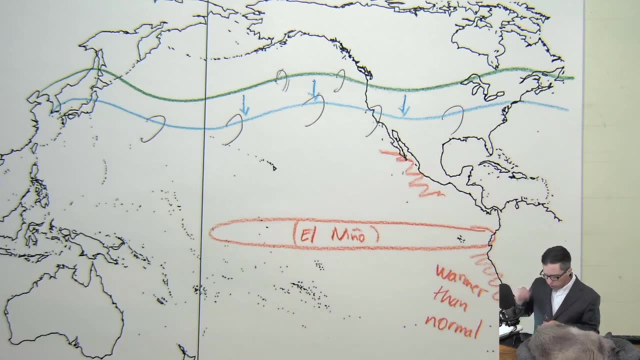 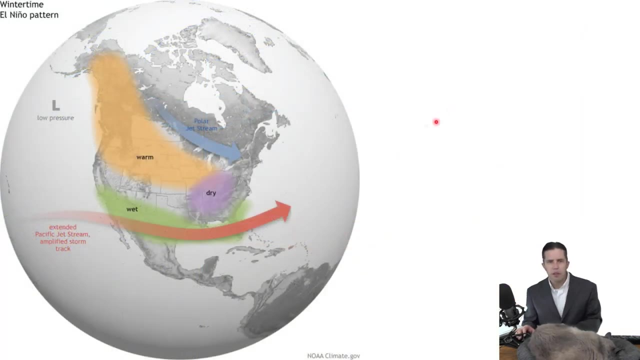 than in a normal non-El Niño year. Okay so this is going to have an effect on our weather because it's shifting the polar front south. Okay so let's look at a couple maps here. So here is a couple of. 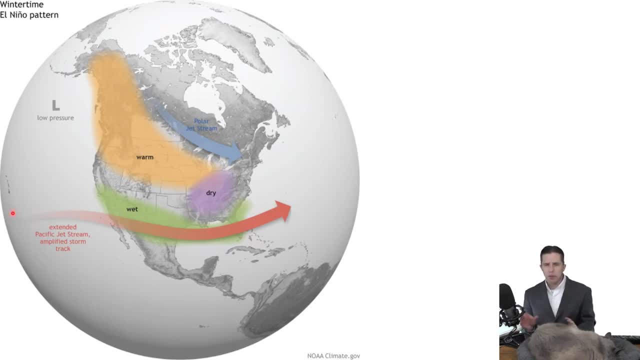 cartoons to try to illustrate this And they're using some slightly different terminology than what we've been using. So so far we've been talking about the jet stream and one type of polar front. There's- actually it splits. there's more than one type of jet. 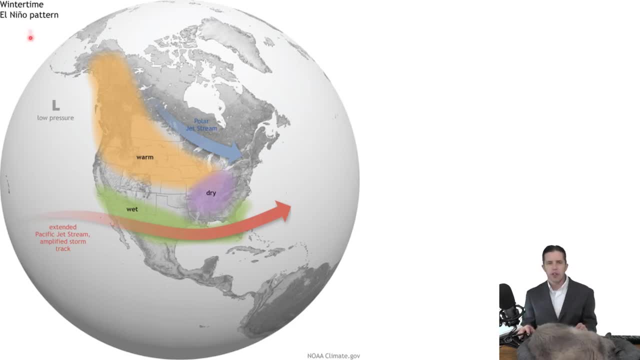 I don't want to get too deep into this, but what they're trying to show here is, in an El Niño, this jet stream, what I'm calling the polar front is bringing in storms kind of right through here in this orange line. 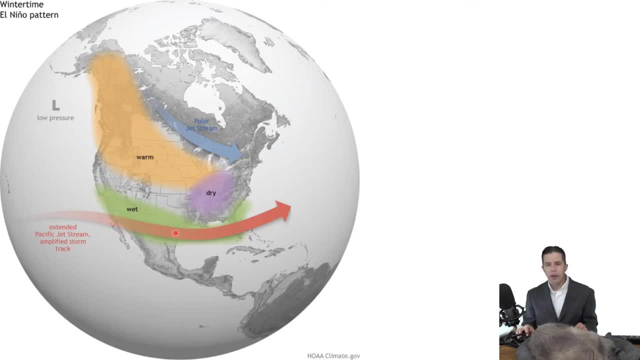 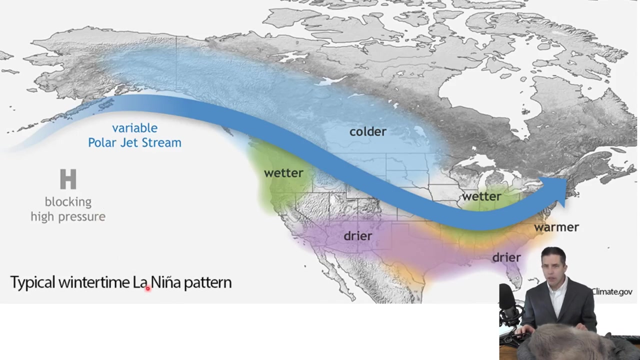 which is going to make this area wetter than normal and this area warmer and drier than normal. So the storms that were coming up here are now coming further south In El Niño, the opposite happens. In El Niño, the jet 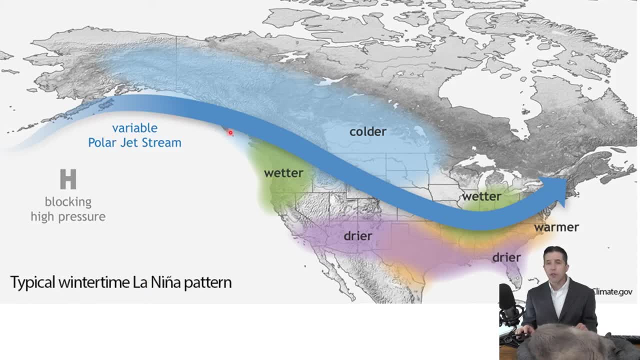 the polar front again is shifted further to the north, So it's exactly the opposite, and the storms tend to go further to the north and skip us more often. So we end up to be drier and they end up to be wetter. 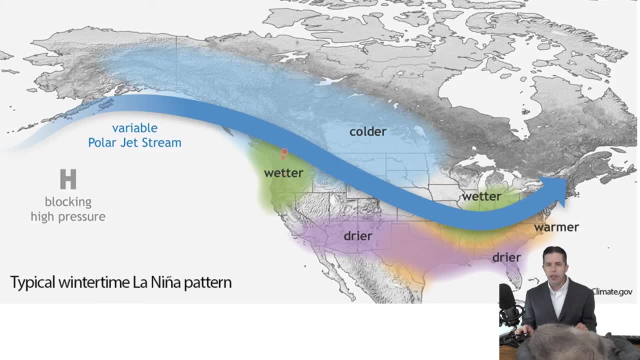 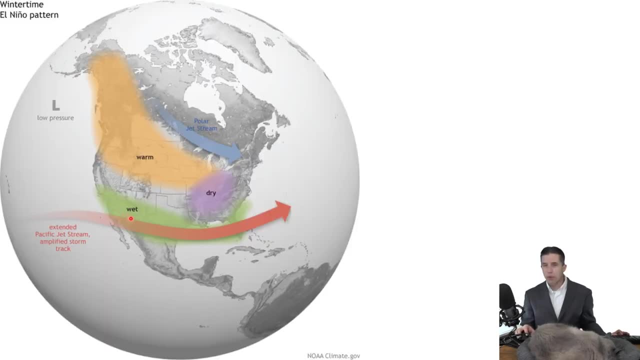 Okay. so what we're doing is we're shifting the location of where those middle-atitude cyclones come in. In an El Niño, they tend to come further south. they make us wetter. In a La Niña, they tend to go further north. 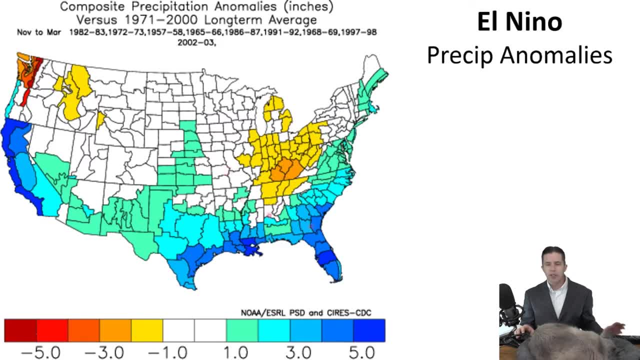 make us drier, So that's going to have an effect on our overall winter weather. So this is a new type of map we haven't seen in this class yet. It's called an anomaly map. Anomaly means something that's different than normal. 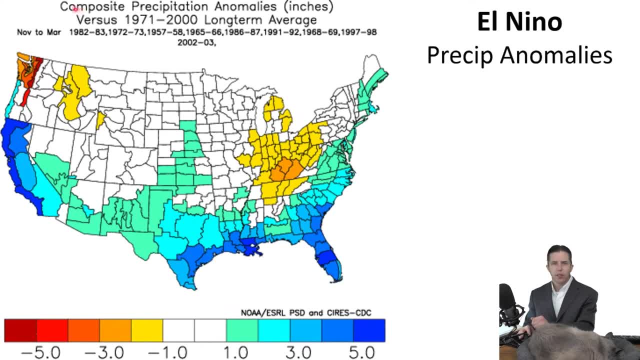 So these colors, this is a, this is composite precipitation anomalies, And what they've done is they've: every time there was an El Niño, they looked at all the precipitation records for that El Niño event and they compared it to what the average precipitation. 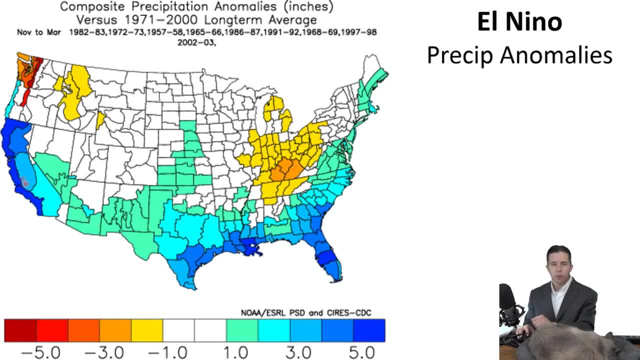 was in the past. Okay. so what they've noticed is that the places that are blue, so it says five, okay. so what does that mean? That means that during the winter, places that are dark blue on average got five inches of precipitation. 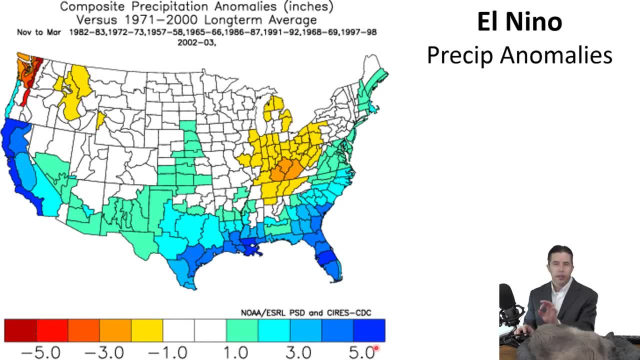 more than they normally would. That's an anomaly, Whereas places that are, say, yellow or orange, got minus one, minus two, minus three inches from normal. So this isn't telling you how much precipitation they received, It's telling you how much extra. 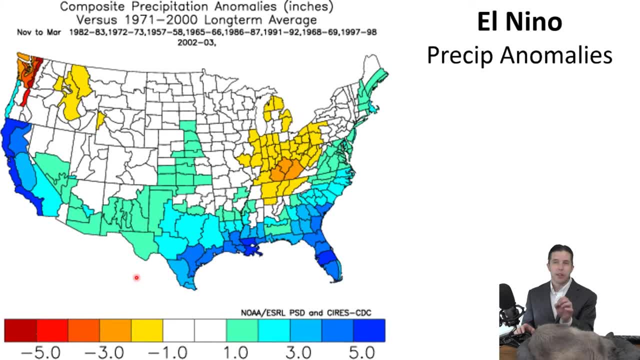 or how much less they got than what they normally expect, right? So everyone, everybody that's on this side, in these green and aqua colors, are getting more precipitation than a normal year, And you'll see that New Mexico is right in here. 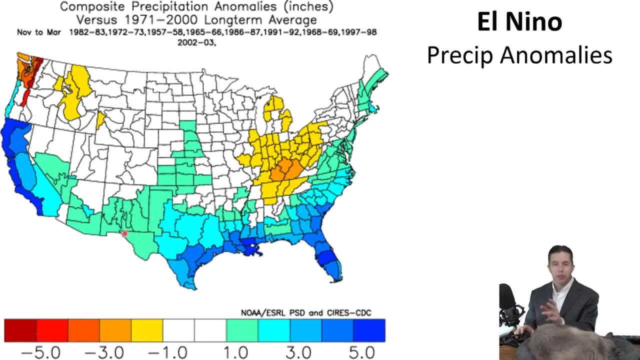 So we get about one inch more than normal during an El Nino Again. this is spread out throughout the whole winter, right? Why is that? Because the mid-latitude cyclones are being directed further south, So they come in. they dump a lot in California. 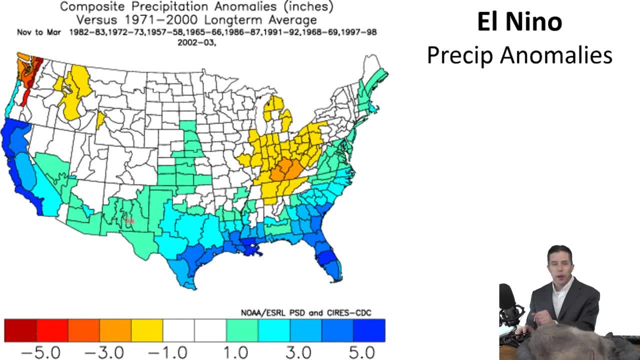 then they kind of move downstream towards us and we pick up some of that extra precipitation. Now these guys are in the red. You can see the minus three, minus four, minus five inches. These guys are getting less precipitation than they normally would. 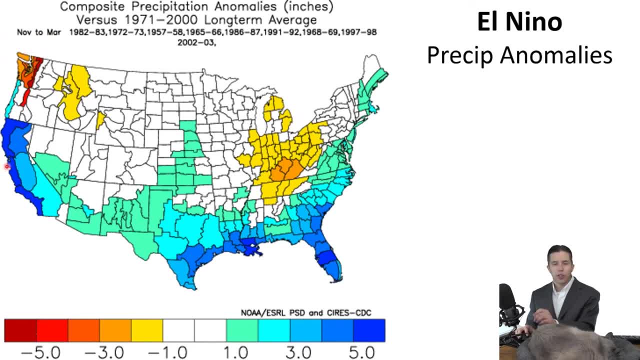 because the storms that used to come in here are now shifted further south. So whether El Nino is good or bad depends on where you live. Let's say you're a skier, right? Well, if you're a skier in New Mexico, 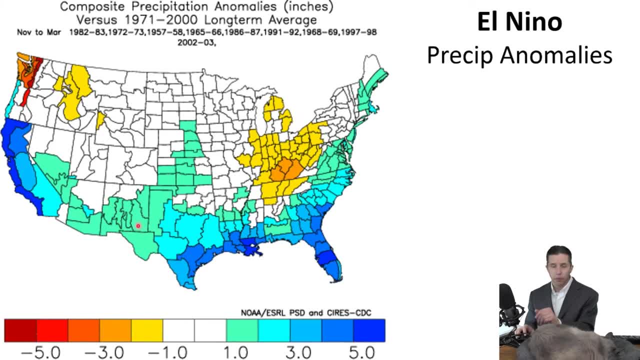 you're happy when El Nino happens. We get more snow. If you're a skier in Washington State, you're sad when El Nino happens because you have less snow. Now, this is an anomaly map, so this is different than average. 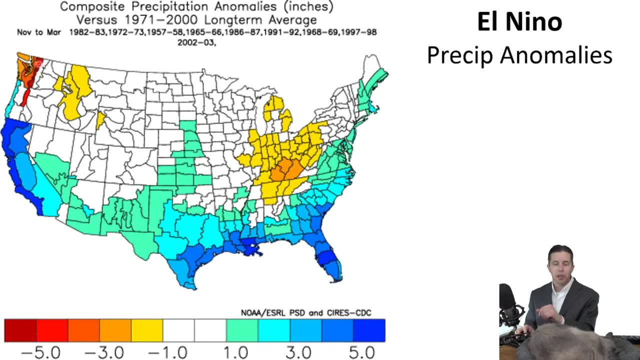 So it does not mean the red does not mean that they are drier than we are. This is Washington State right. So we get eight inches of precipitation a year. in Albuquerque They get like 120, something like that. This is saying that there's five inches less. 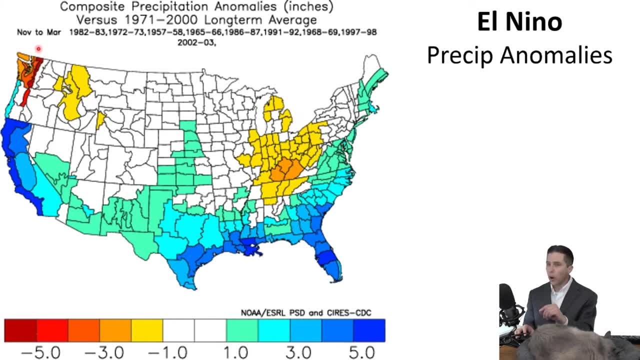 than their normal, but their normal is way bigger than our normal. Keep in mind. this doesn't mean that they're dry and we're wet. That means they're drier than normal. This means we're wetter than normal. So that's how you read an anomaly map. 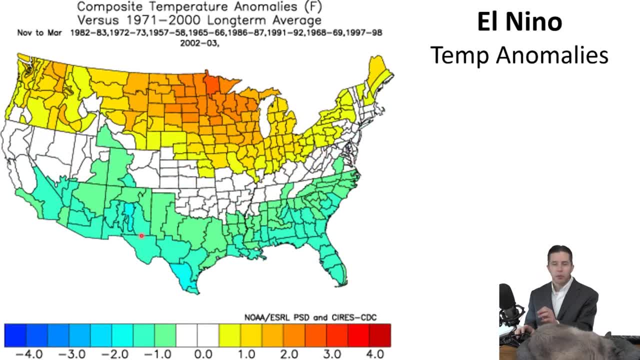 So temperature-wise there is a difference too. So if the middle latitude cyclones are coming further south and they're going across the southern United States, we're going to have more cloudy days, And that's going to lower the temperature a couple of degrees. 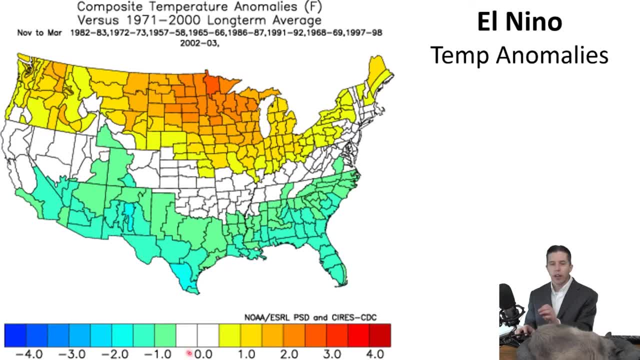 These guys are going to have more sunny days, And so they're going to have temperatures a couple of degrees greater than average. So in an El Nino winter again, all these maps are for winter does not seem to affect our summer. 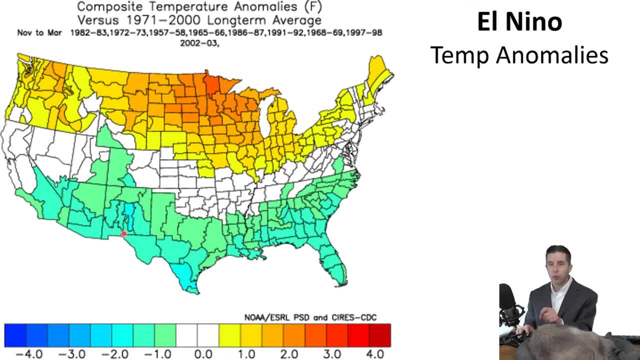 We have a wetter than normal winter. We have a cooler than normal winter. These guys have a drier than normal winter and a warmer than normal winter. for an El Nino, La Nina, everything's flipped almost, So the storms are concentrated. 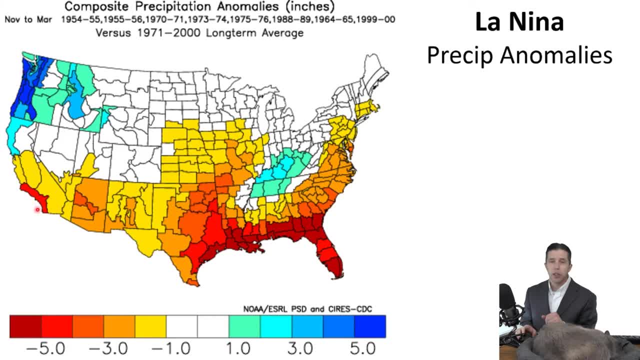 to come up in here more than they do, and they miss us almost completely. And so here we have, you know, negative one, negative two, negative three inches again over the whole winter. that would be one, two or three inches less. 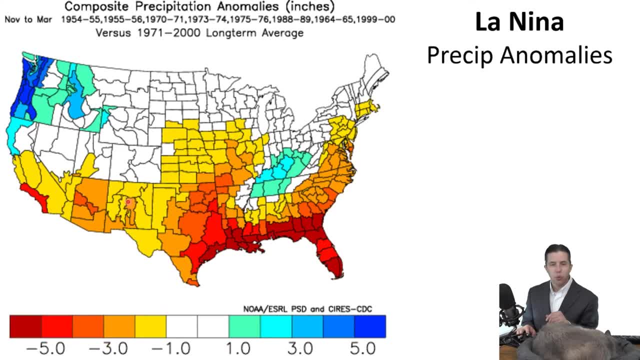 than what we normally get. So, if you notice so, Albuquerque is in this one right here, and it's somewhere between negative two and negative three inches. So that means that during a La Nina winter, we expect two to three inches below normal of precipitation. 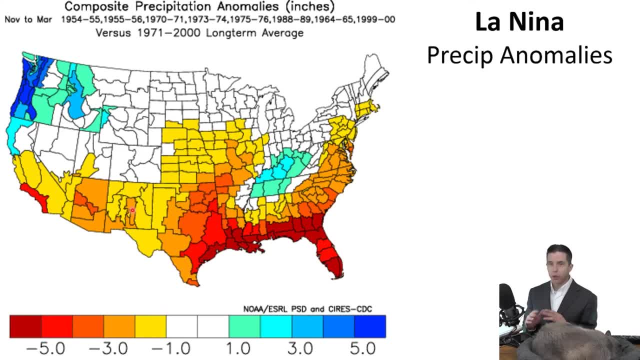 Well, how much precipitation do we normally get throughout the whole winter? in New Mexico, Maybe like two inches. So two inches minus two is zero. So when we have a La Nina, it often, often results in a winter that's almost completely dry. 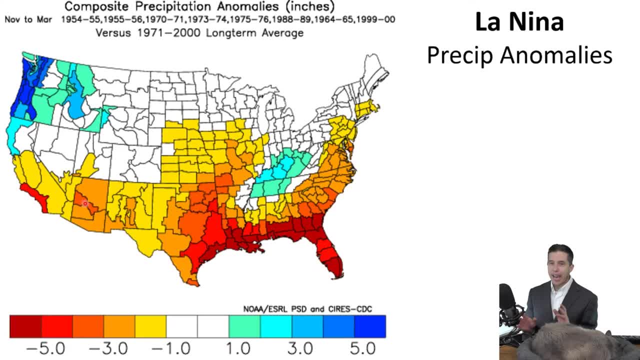 So we in the Southwest hate La Nina because it means the area of the country that's already really dry- Remember that Pacific subtropical high we've been talking about makes this whole area desert. Well, in a La Nina winter it gets worse, because now 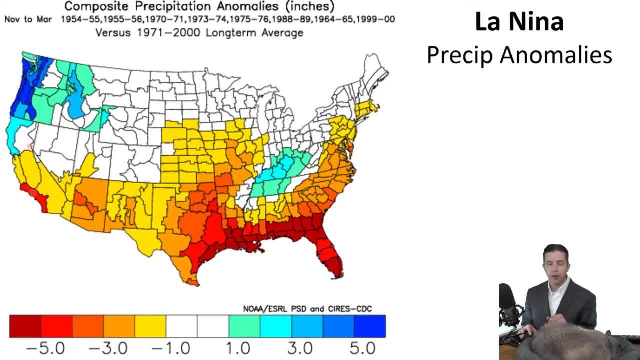 the storms are missing us even more than often. They're going up here and we're even drier. And again there are winters on record where it literally did not produce any measurable precipitation during a La Nina. On the other hand, these guys are getting flooded. 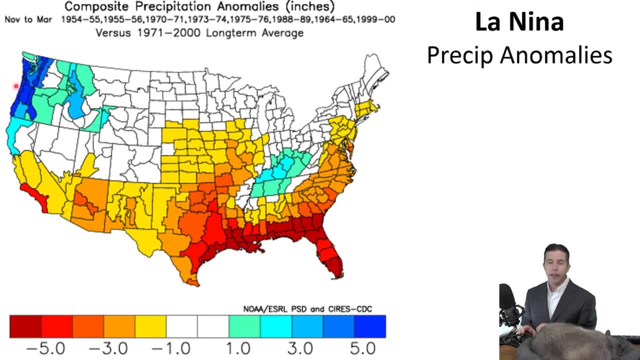 because now they're getting way more storms than they normally get. They're already used to a lot of precipitation because it's Pacific Northwest, but now they're getting even more. So you can see they're getting, you know, excess of five inches above. 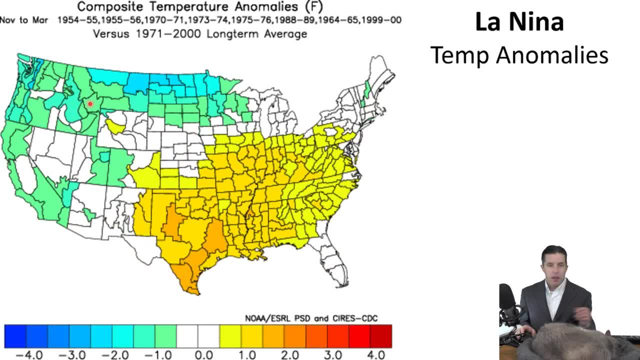 what they normally expect for their winter. Now there's a temperature anomaly, but it doesn't quite match up like you might expect. In general, this part of the country is warmer than normal. in a La Nina, You might think we would be too. 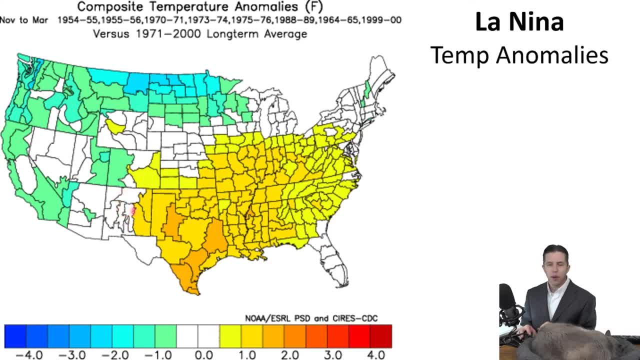 but for some reason it doesn't ever seem to work out that way. So most of New Mexico's temperatures don't change that much with a La Nina, But up in the Pacific Northwest and actually all these northern states up here are usually having cooler than normal. 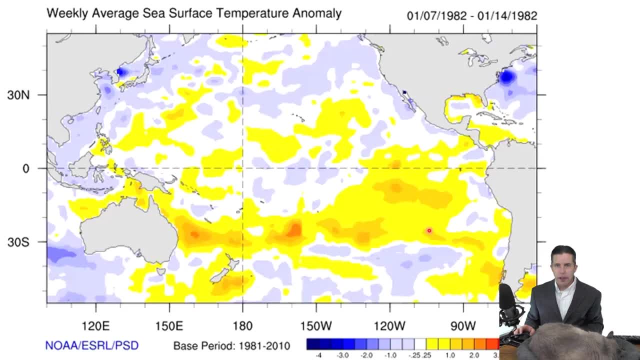 winter temperatures. So we're going to look at another use of the anomaly map And this says weekly average sea surface temperature anomaly. So what that means is everywhere, that's, the yellow and orange and red colors correspond to places where the ocean is warmer than it normally is. 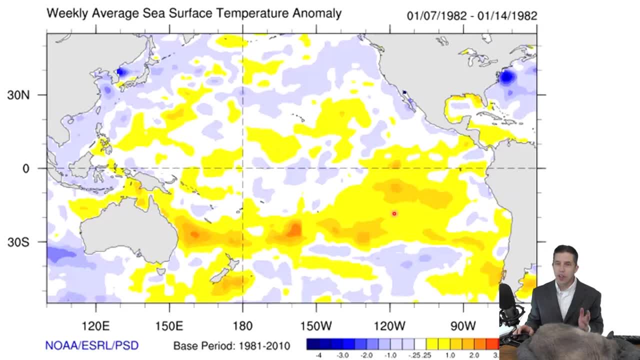 So for this location it's warmer than average. What's average? Usually 30 years, Places that are blue are cooler than their average, So realize how you have to interpret an anomaly map. Right here is a blob of water that's warmer than their average. 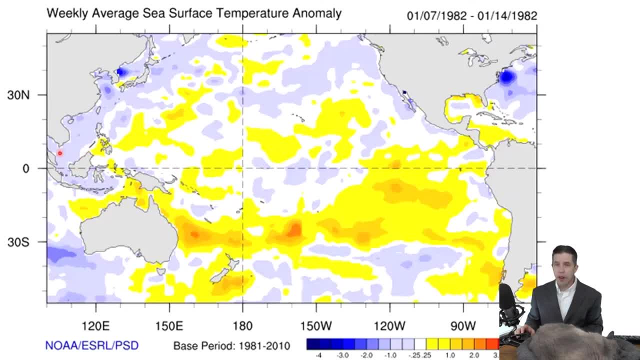 Right here a blob of water that's cooler than their average, But this is that part of the ocean I said was always the warmest part right. So the pool of water right here is really, really warm. all the time. It's always going to be warmer. 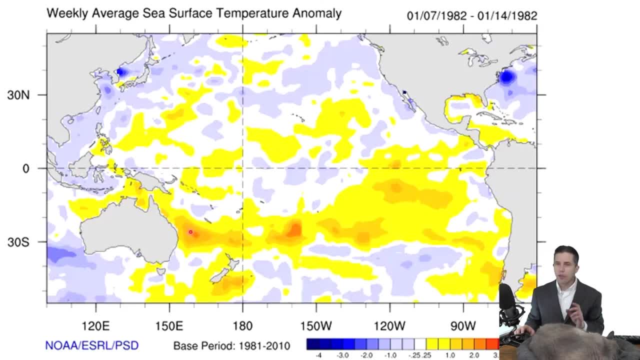 than whatever's down here. So you can't get confused and think that, oh, this is warmer because it's more orange. No, no, no, That means it's warmer than average and this is cooler than average, But their average is still way warmer. 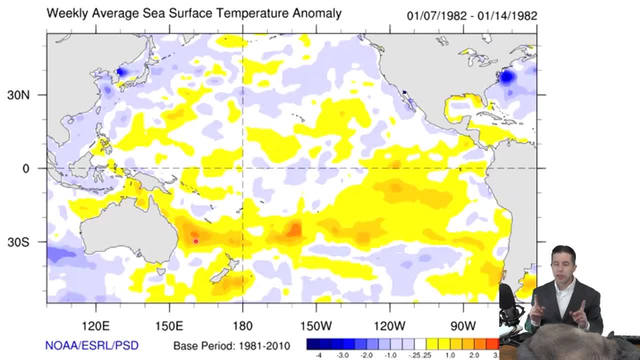 than theirs. So you can't compare direct temperatures in an anomaly map. You can only look at differences from average. Okay, so we're in 1982.. This was an El Niño year, And this is going to become an animation. 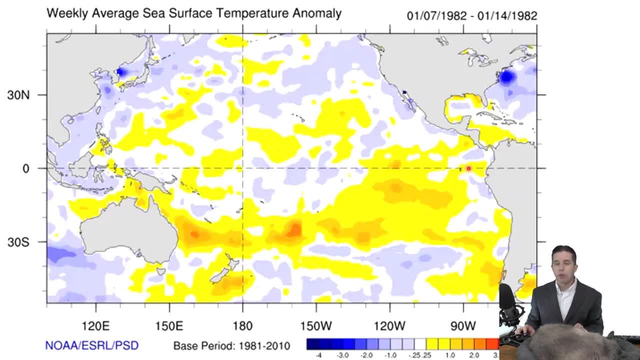 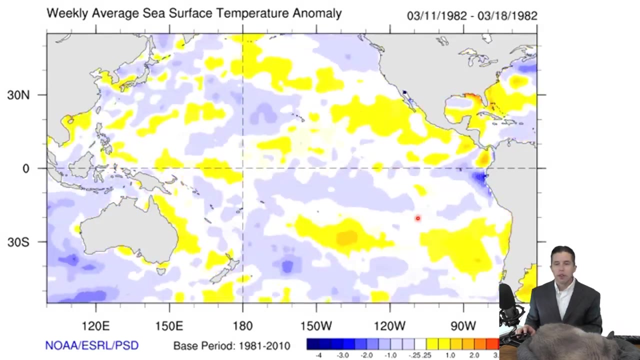 And you're going to see. the weeks click by And what we're looking for are colors around the equator here that show that the ocean is warmer than average, And if we see that, we know we have an El Niño Okay, so watch right in here. 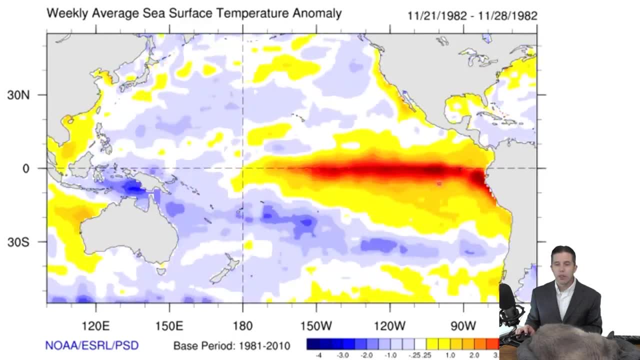 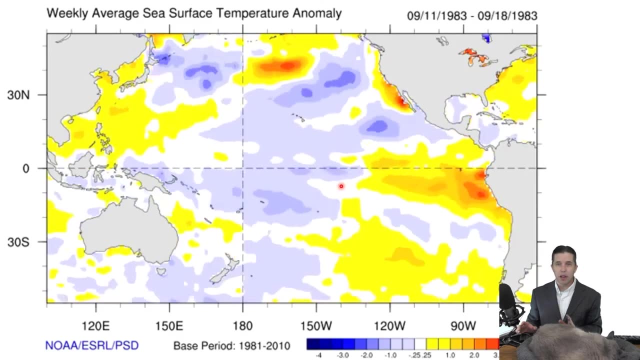 And you see those orange colors come and go right there. That's the El Niño, Right through here. So that's a location in the ocean that's far warmer than normal. That's what happens during an El Niño, because the upwelling shuts off. 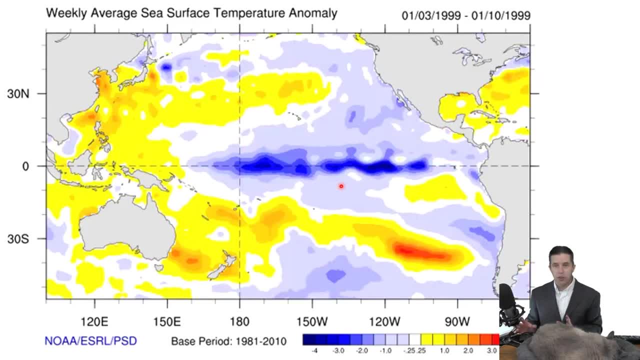 Okay, Similar situation. Now we're in 1999.. This is a La Niña, And we can see the La Niña occurring already. It's this dark blue color. So that's where places are, That's where the ocean is colder. 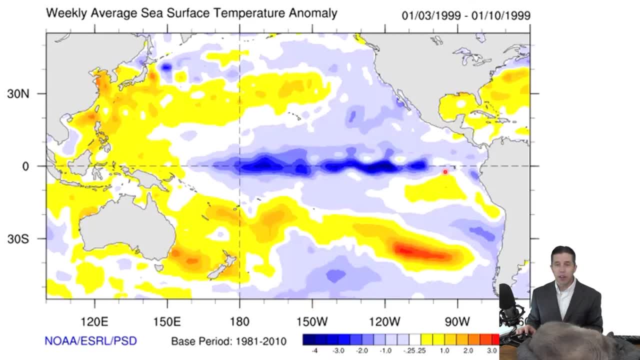 than normal, And so in a La Niña, we expect exactly the opposite than what we just saw. We expect to see blue colors along here, And when you start the animation you can watch how it'll kind of grow back and forth here. 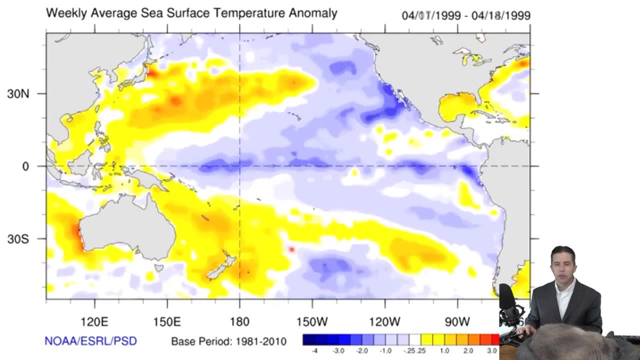 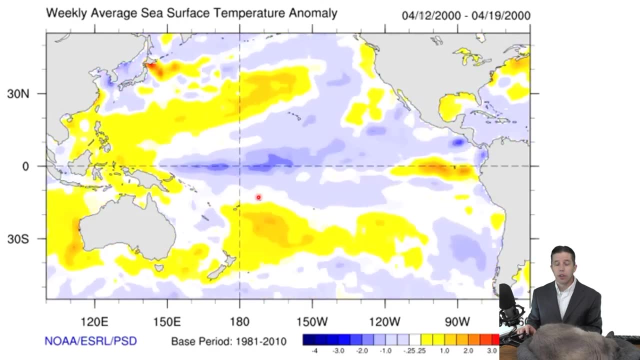 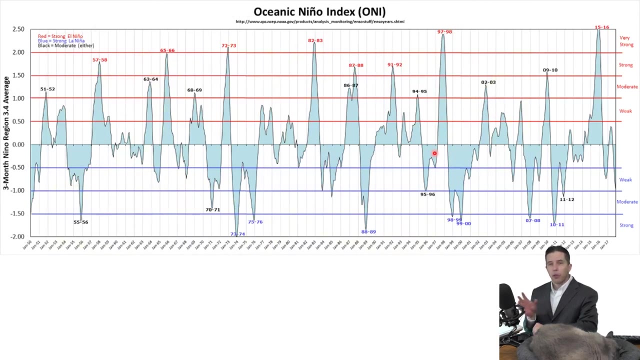 along the equator. Okay, so there's the blue. Goes away a little bit, Comes back a little bit, So this is a La Niña event Right through there. Okay, So the ocean can go back and forth between El Niño and La Niña. 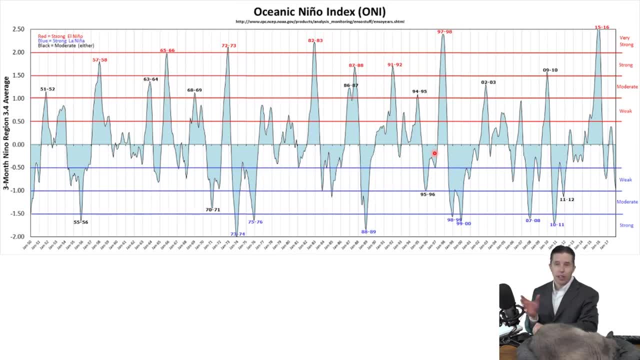 from year to year, And a lot of years is not in either one, And so there's been some attempts to try to describe how strong an El Niño or La Niña is, And so here's one example. It's called the Ocean Niño Index. 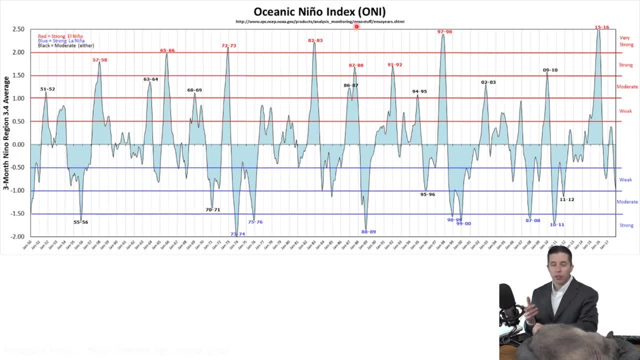 Also known as the El Niño Index or the ENSO Index. So here is on the x-axis. we have time. So this is January 2004,, January 2005.. Each one of these marks is another year. Okay. 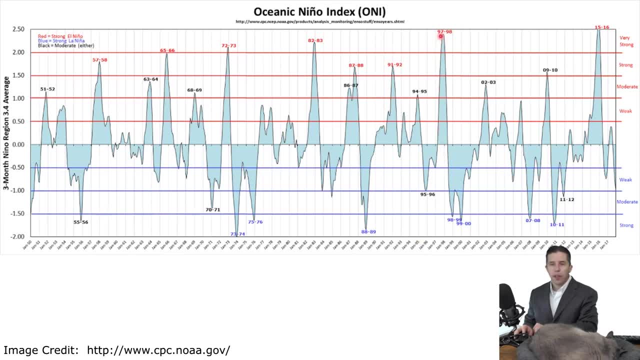 So if you have one of these peaks that's on the red part of the graph, that was an El Niño. If you have a peak in the blue part of the graph, that's a La Niña. And the higher the peak, the stronger. 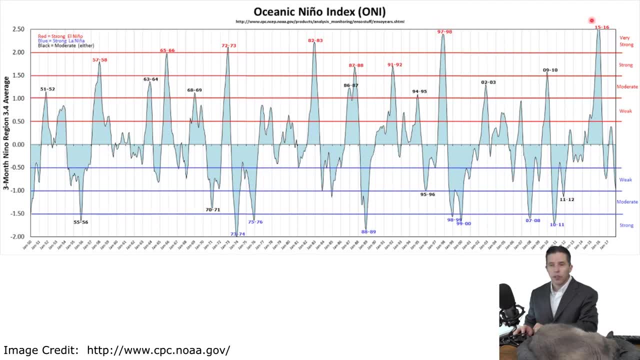 event. So this is a very strong El Niño right here. This is a very strong El Niño right here. These would be considered El Niños, but they're pretty weak. These are pretty strong La Niñas and these are pretty weak ones. 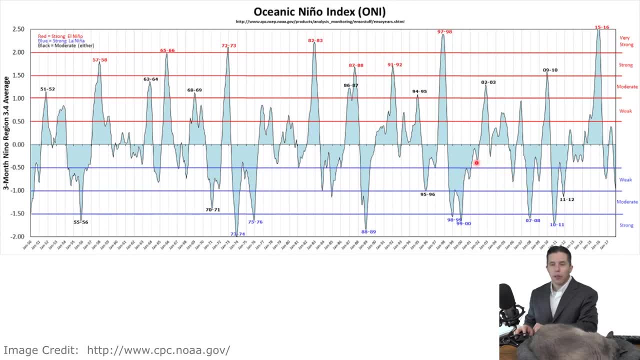 So a lot of years. if you have a little peak like that one or that one or that one, you'd just say this is an ENSO neutral year. It's a little bit in the La Niña or a little bit in the El Niño. 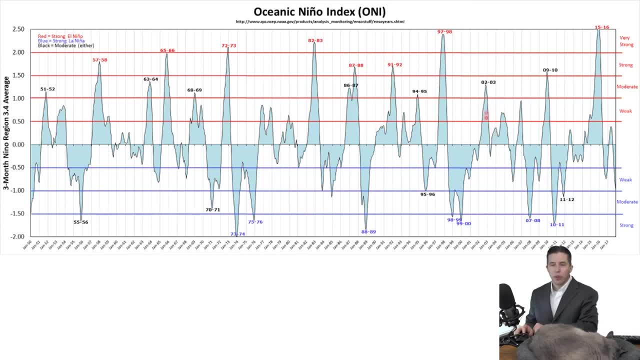 direction, but not enough to count. In some years you've got these weak events and in some years we have these strong events. In some years we have a couple years in a row of the same thing. So, for example, here there was one winter, 86-87. 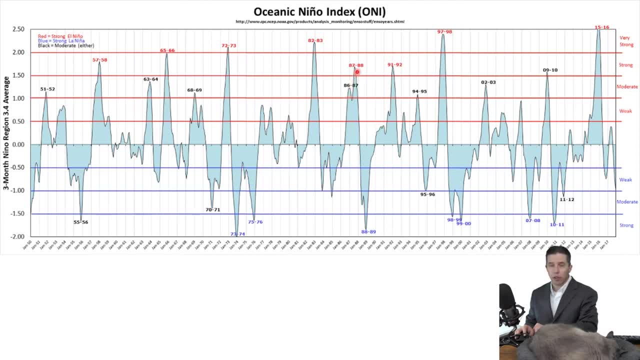 which was an El Niño, and then the next year after that an even stronger El Niño. So think about what that would do for New Mexico's precipitation. El Niño year, wet winter right, So we likely had two winters in a row that had above. 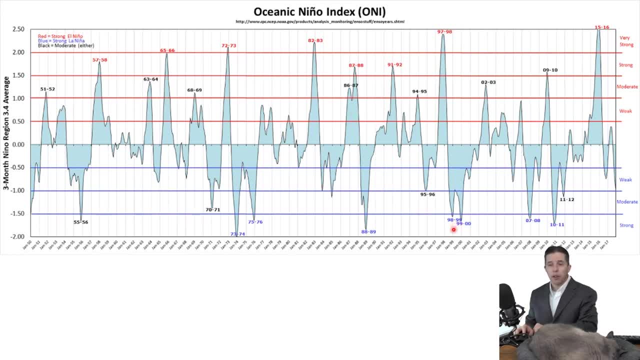 average precipitation. On the other hand, look at what happened here: La Niña, La Niña and then really wimpy La Niña followed after that. This whole time in here, the ocean is in a La Niña state, La Niña. dry winter. So we're looking at two or three or maybe four years in a row where New Mexico would have had a winter with below average precipitation. For us that's a big deal. You've got dry winter after dry winter, after dry winter. it adds up and you've got.